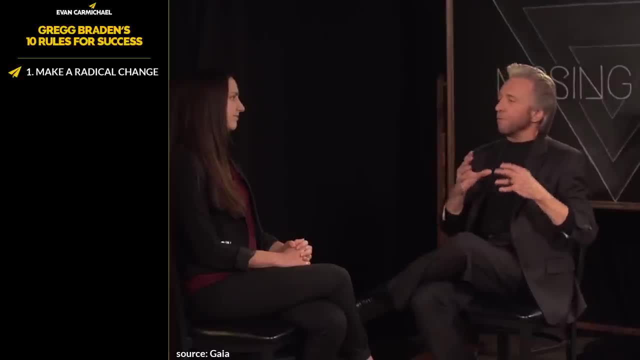 We have been conditioned to live in a world through a way of thinking that has served us in the past, And we have to say it served us because you and I are here now, so it worked well enough to get us here. That way of thinking worked in the world the way it used to be. 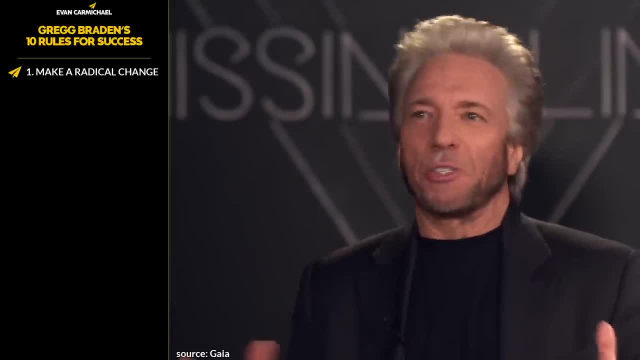 The world just changed and nobody told us. There was no special on CNN or the Discovery Channel. Hey, the world changed. I wish there was. So we've never been given the opportunity to even mourn the passing of the world that no longer exists. So we're trying to solve our 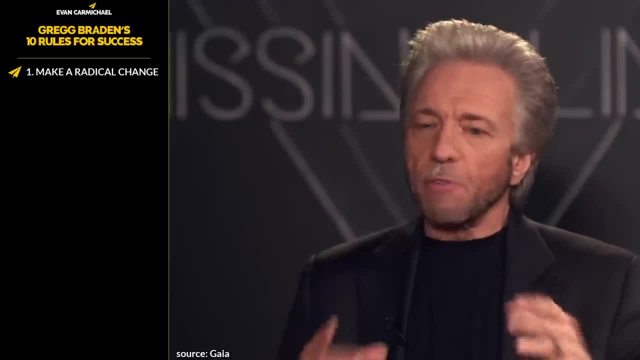 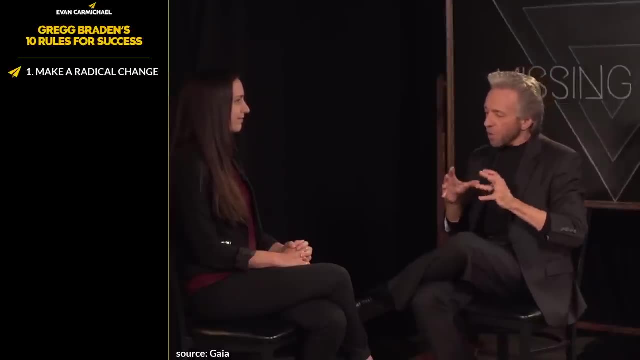 problems and think about ourselves the way we always have in a world that changed and it doesn't fit. It no longer fits. So yes, we've got all these little things going on, But what I've found in my own life personally, 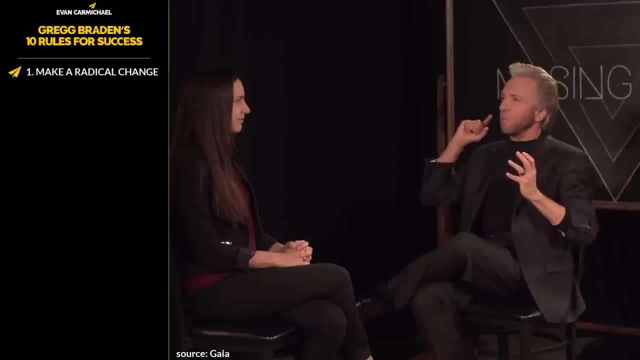 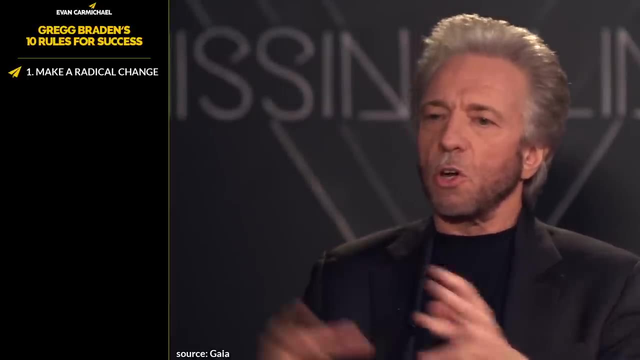 if I can back up and shift the paradigm- and I'll tell you what I mean by that. but if I can shift the paradigm within which I'm seeing everything, all of a sudden all those little things take on a whole new meaning and they become a lot less of a problem, They become much easier. 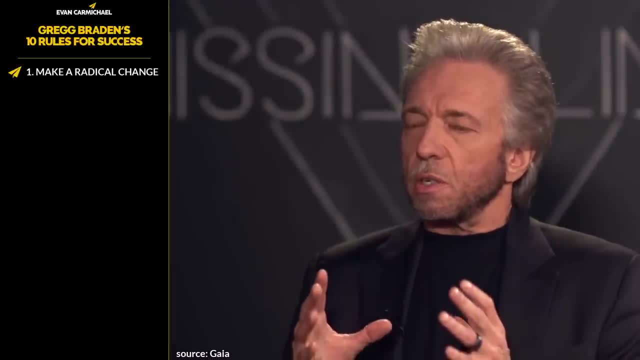 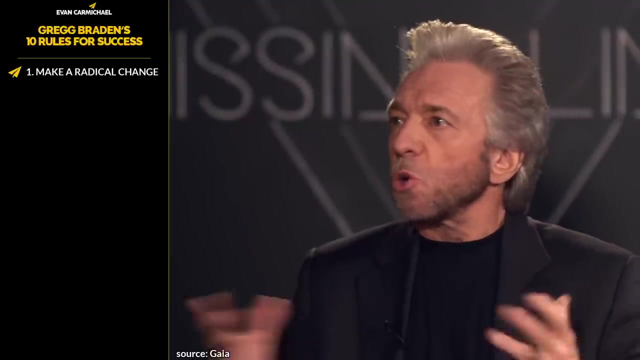 The paradigm is this: We have been conditioned, steeped in a story of who we are that is based in separation, competition and conflict. It began in 1859.. People say to me: Greg, 1859, it was over 100 years ago, 150 years ago. So what? It's a good. 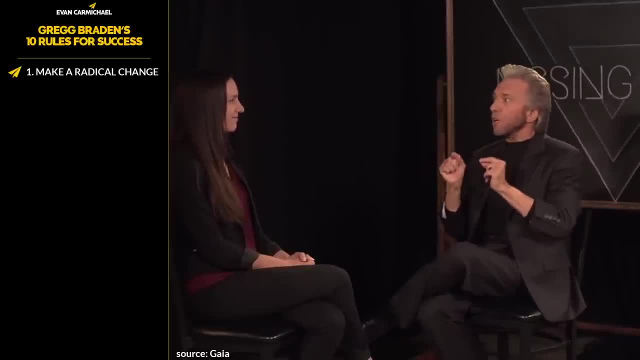 question. What difference does that make? It's a good question. Here's the answer: The world we live in, the society, the economic system, the corporations, the medical model, the way that we're taught to provide for our families, the way that we are taught to have the most intimate. 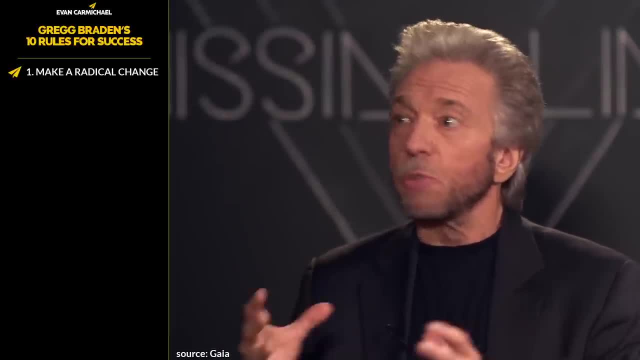 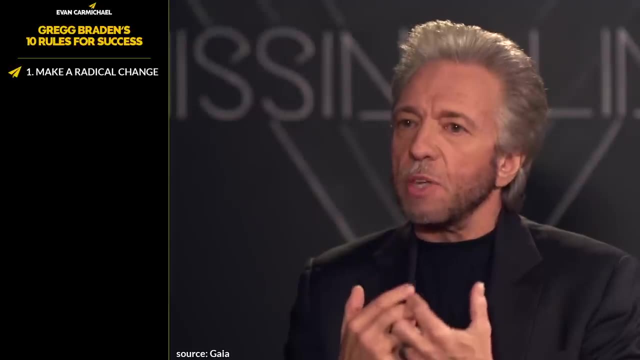 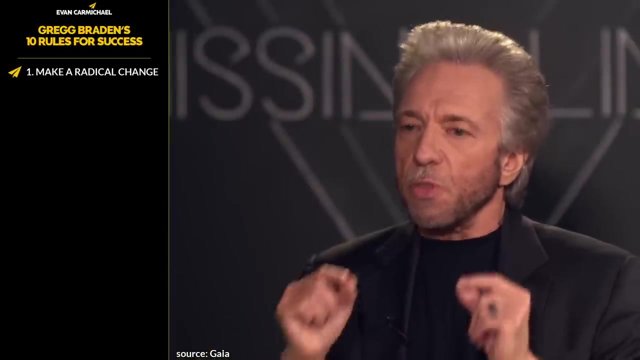 relationships under the roof with the people that we share our homes and even our bed with. I mean, let's just get real. We are taught to interact. We interact with humans based upon these ideas of competition, conflict and separation, And even the most spiritually minded people that say I've transcended that when they are in a 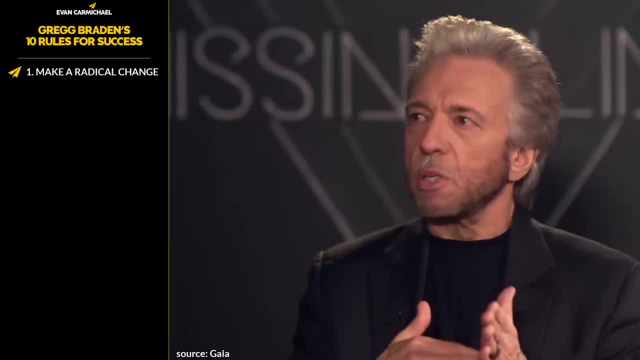 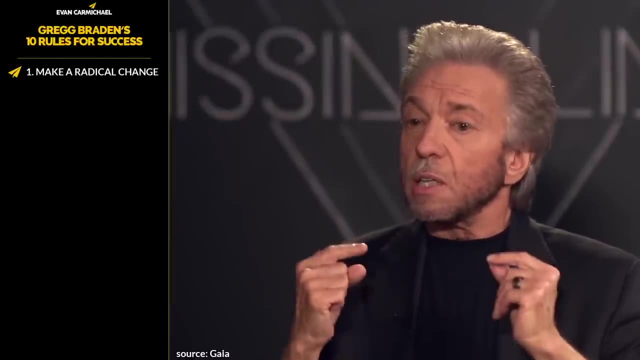 heated discussion and somebody pushes their buttons, they go to that lowest common denominator, often of competition. They will lash out with something really hurtful to defend themselves. It's not their fault, It's deeply ingrained in our subconscious, So as not if because it's. 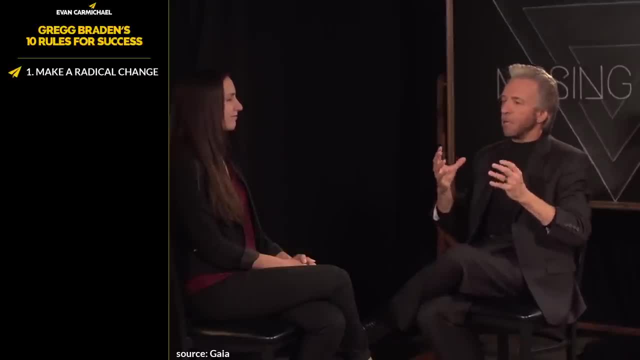 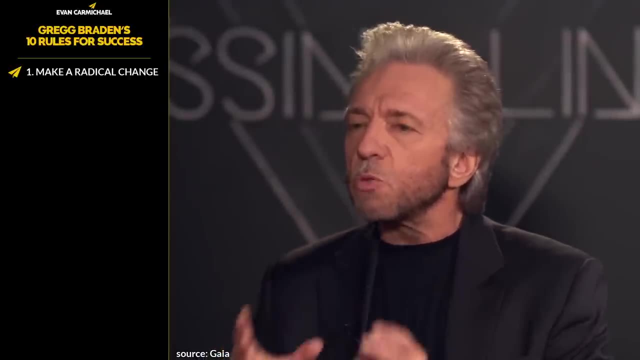 already happening as we back off and embrace the new paradigm of cooperation and mutual aid. that is huge. It is a hugely different way of thinking. It means we live in a world that likes us, where nature is not out to snuff out every good thing. 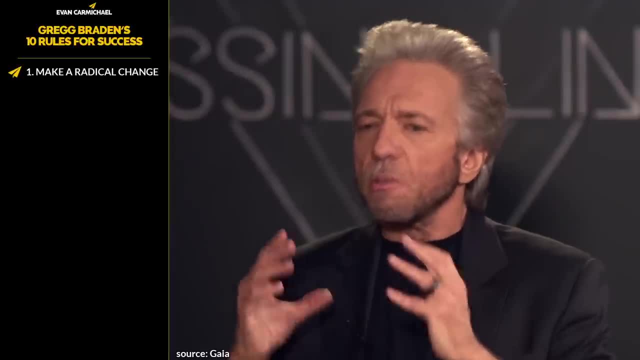 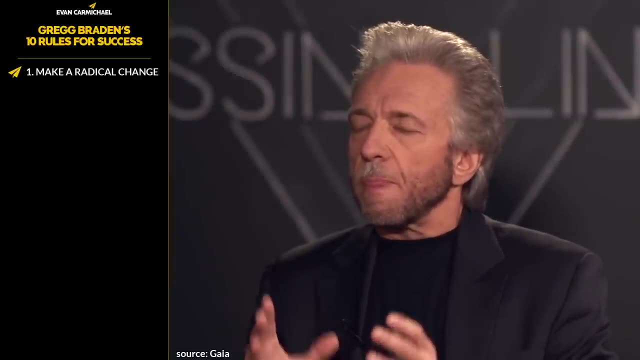 that happens to us. It means we don't have to be constantly vigilant in defending ourselves from the world around us. That is a hugely, vastly different way of thinking, And we have an opportunity now to begin with an entire generation of young people who now are steeped in the glamour of war. 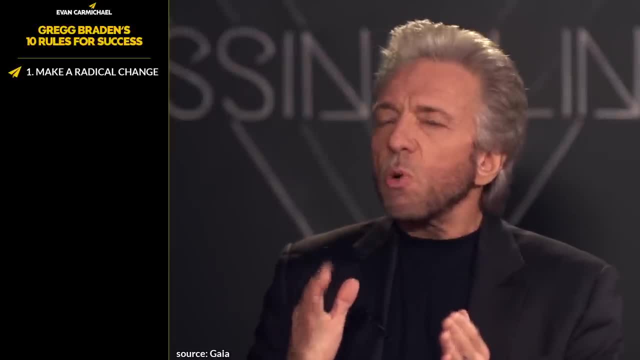 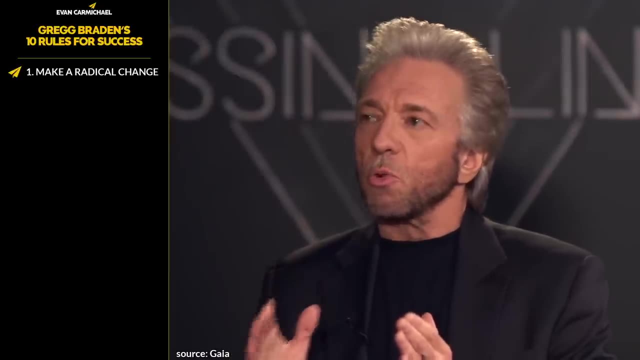 conflict and competition to make that shift. What would it look like to have a world where we have an entire generation of young people that know that nature likes them and that we live in a world of cooperation and mutual aid and connection? We're about to find out. We don't. 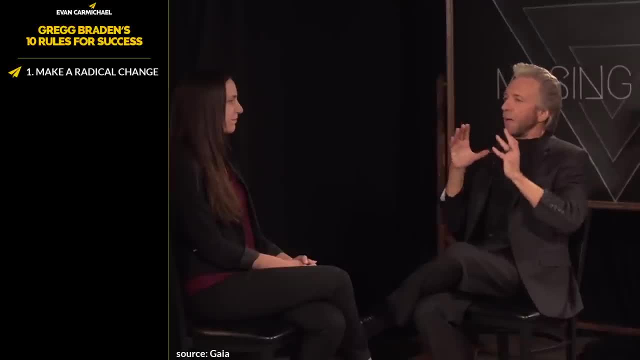 have to wait long to find out. So for me, simply backing up out of the minutiae momentarily to look at the big picture and to make that shift. And once we make that shift, when you go back into the minutiae, everything looks different to me. 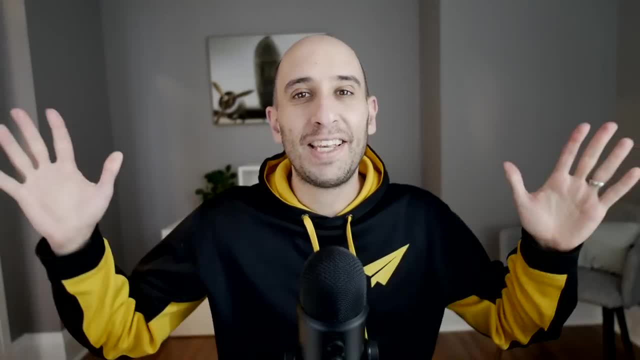 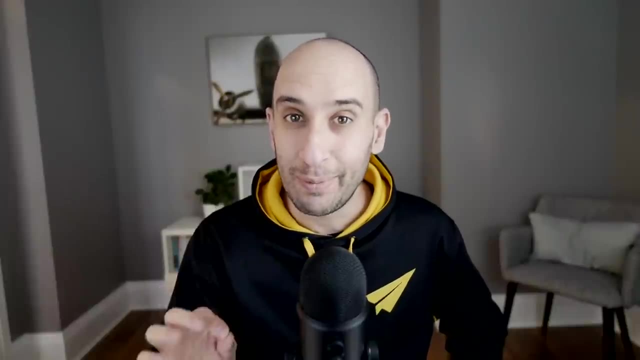 Need motivation? Watch the top 10 with Believe Nation. Hey, it's Evan Carmichael, and I make these videos because you are probably the most ambitious person in your circle, But you know you're capable of more, and you get that push by surrounding yourself. 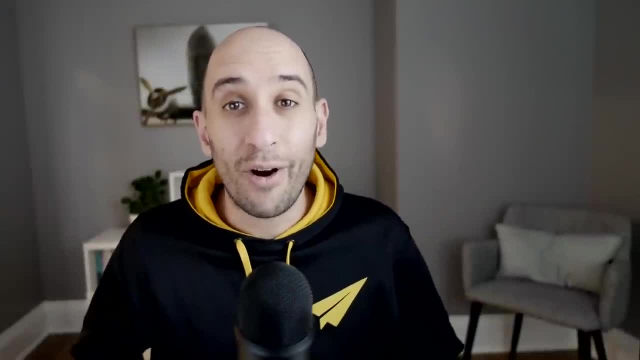 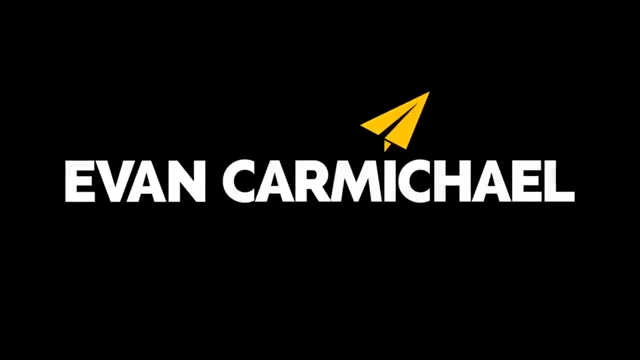 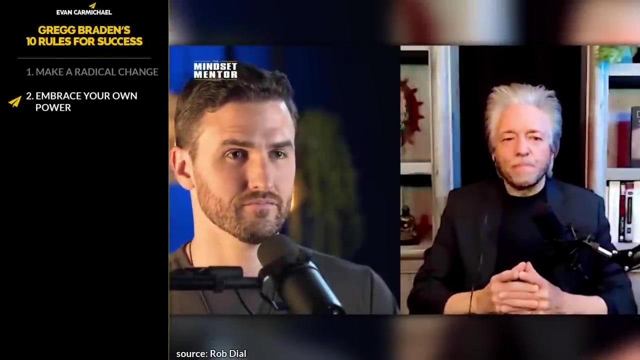 with the best. So today, let's learn from one of the best, Greg Braden, and my take on his top 10 rules of success. Enjoy Rule number two: embrace your own power When it comes to an affirmation. affirmations can be powerful, And for some people they're. 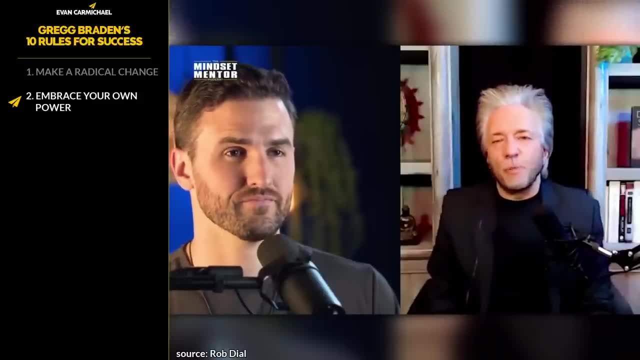 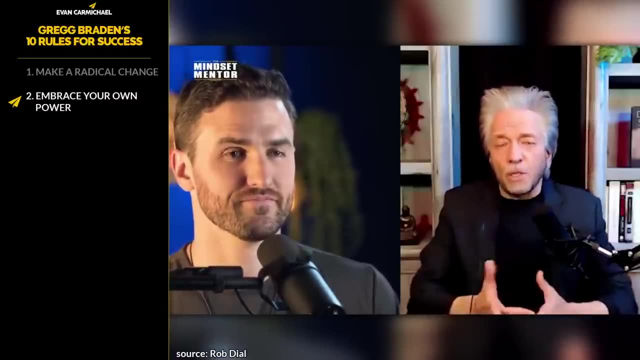 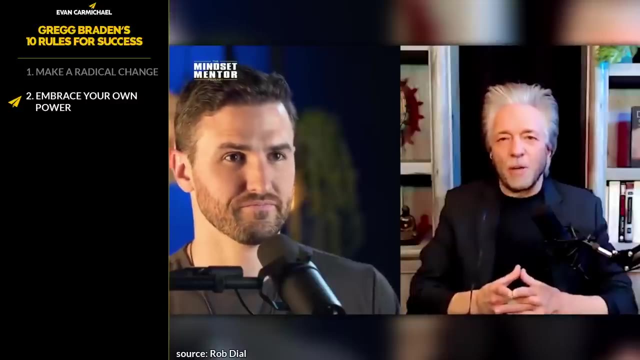 not. And a lot of people say: Well you know, if the affirmation is so powerful, how come I'm not experiencing the effect? The what scientists tell us is the average human speaks to themselves, consciously or unconsciously. we have thoughts spinning around in our brain, about 60 to 80,000 thoughts per day. Some of those thoughts: 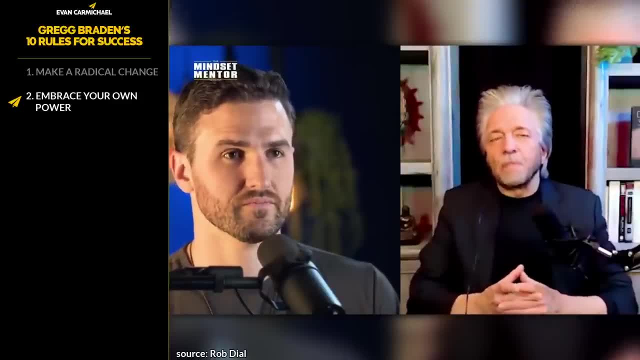 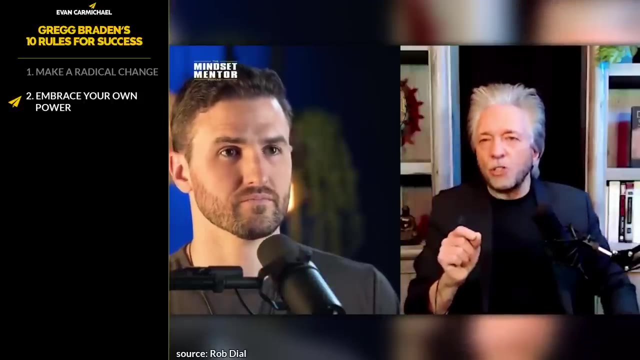 are the words to the songs and they are the affirmations Neuroscientist Andrew Newberg tells us- Newberg is his name, I'm sorry- in his work that a single word, a single word, has the power to change the genes that create stress or relieve stress in our lives. 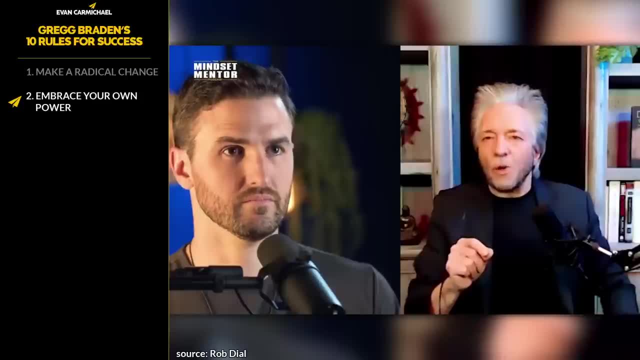 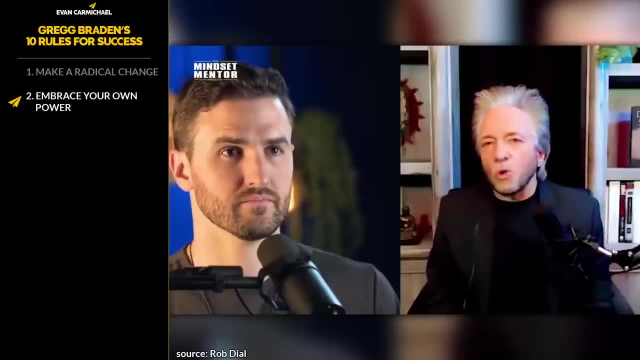 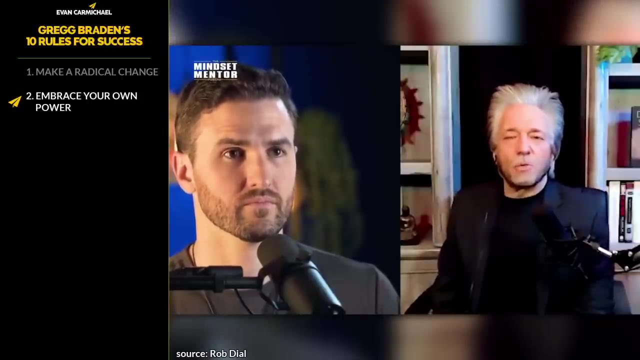 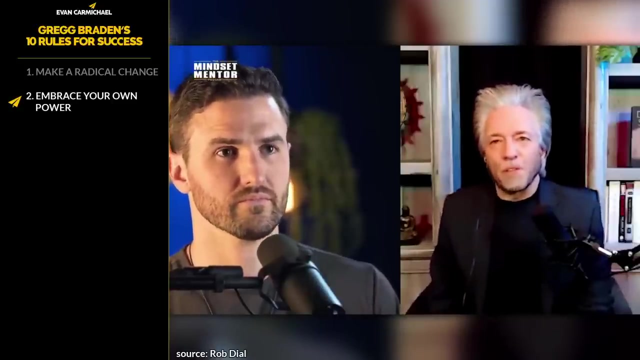 He's telling us that something within us has the ability to shift the very core of our expression. So we know that words are powerful. The key to a successful affirmation is that we must communicate with the subconscious part of our mind. number one. Number two: we must communicate in the language that the subconscious recognizes. 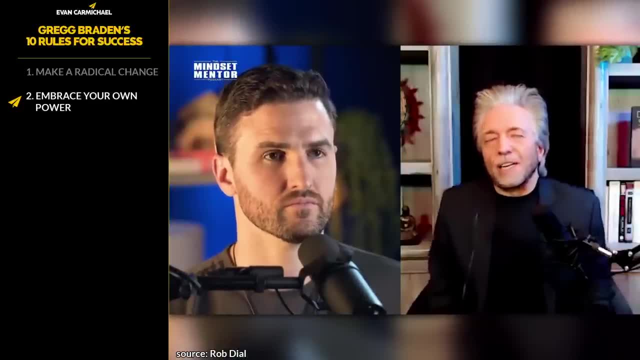 And this is where you know, you can say: I had a friend of mine when I was working in the corporations that had affirmations all over his office, all over his computer screen. They were on little post-it notes in the car. 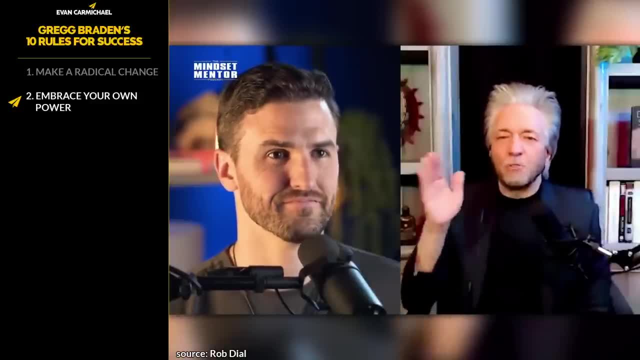 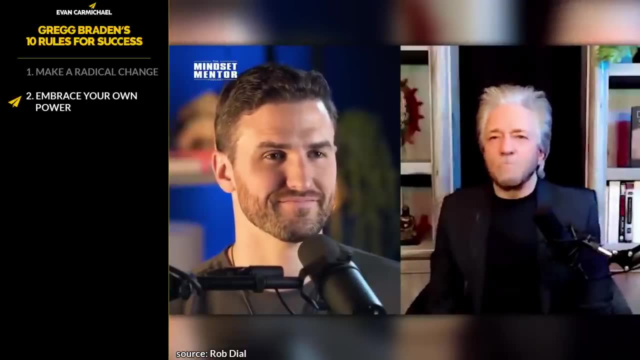 We would carpool in. you know, my perfect mate is manifesting for me now. My perfect mate is manifesting for me now. That was his affirmation. And I said: do you say these things? He goes. oh man, I say them about a million times a day. 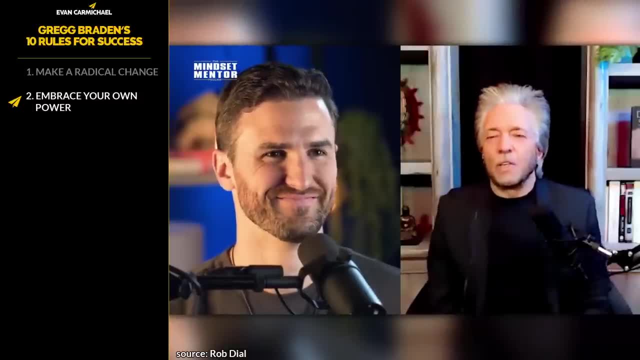 I said: do they work for you? He says: nah, you know these, these things don't work. And I said: why do you think they don't work? And he said: look at me. He says I'm an engineer. 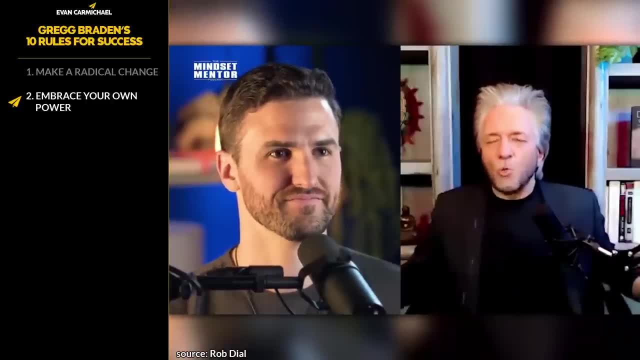 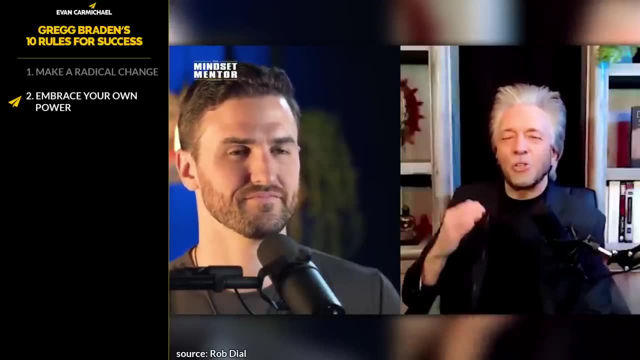 I'm a slob, He said. I wear the same clothes to work three out of five days during during the week, you know, and and the the bottom line. by the time he finished describing himself to me, even he didn't believe that he was worthy of his perfect mate manifesting for. 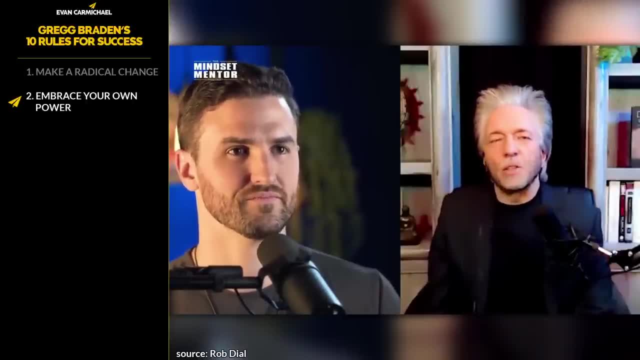 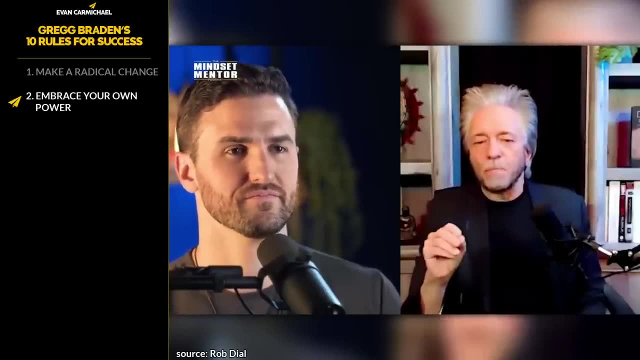 him now. So he was saying the words, but he was not. there was the, the underlying emotion, and what he was actually feeding into his, his system, was counter to what those words were saying. So it's it's not enough to say the words. 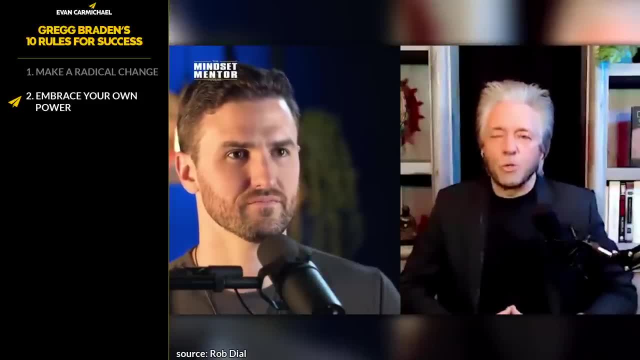 When we go into our most ancient and cherished spiritual traditions, those words are what become the prayers And for many people I have- and I know you've heard this as well- A lot of people feel that prayer is broken, that the world doesn't work today. 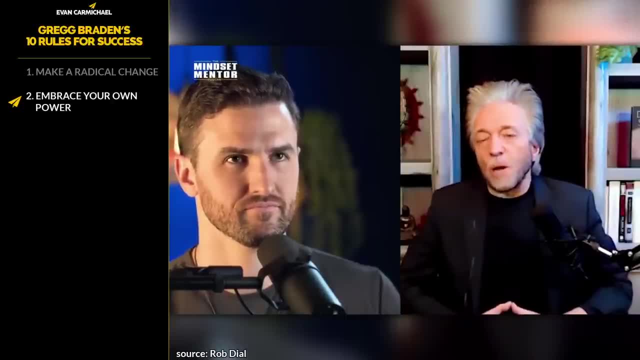 The way it worked in biblical times, that we have lost our power and that we have no ability to communicate with a greater power, with God, with the forces around us. And it's largely because the secrets, the deep truth of our, our relationship. 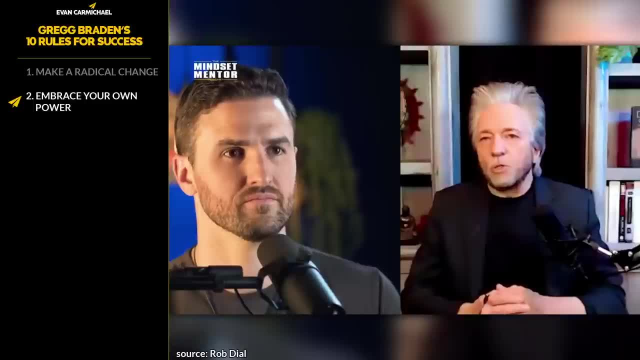 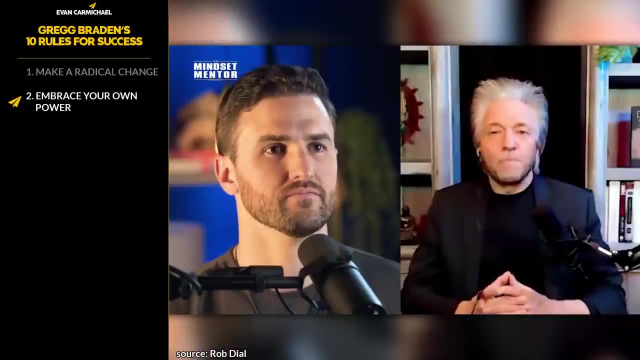 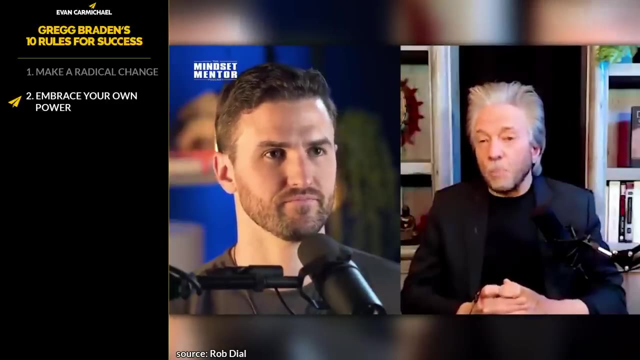 the fundamental physics of our relationship to our world uh have been minced and parceled And, in many cases, deleted from the texts, leaving us with a sense that we are essentially powerless beings, And if you are powerless then you are a victim. 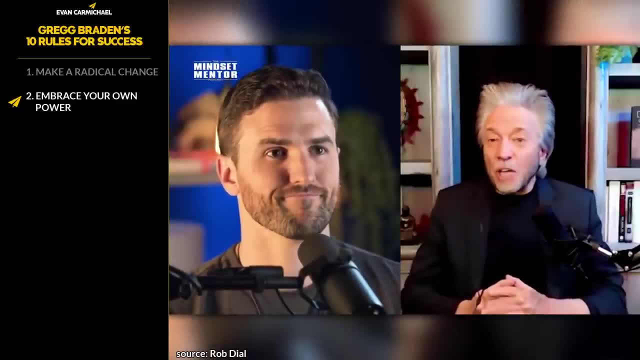 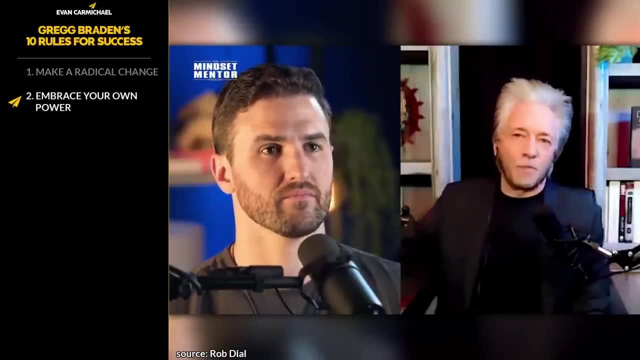 And if you're a victim, you need a savior, And that savior is coming to us on a silver plate in terms of technology, in terms of of political leaders. I will save you if you just do these things, And this is why I say: 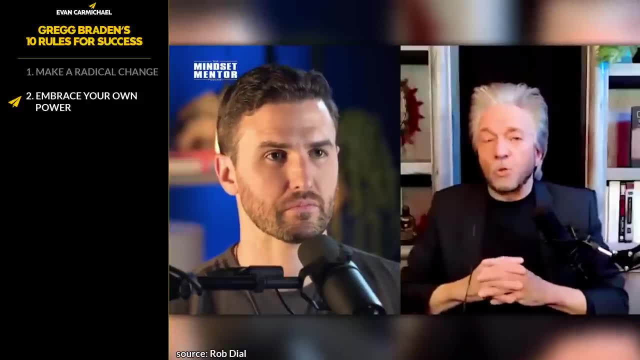 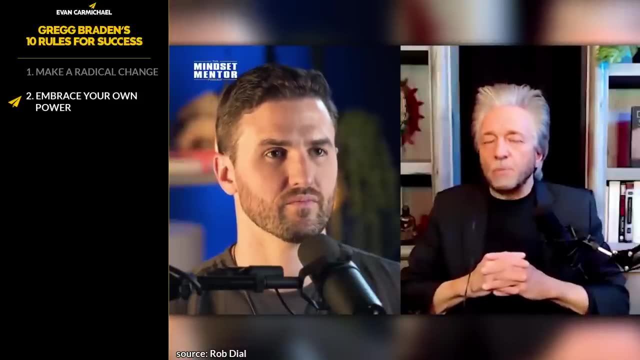 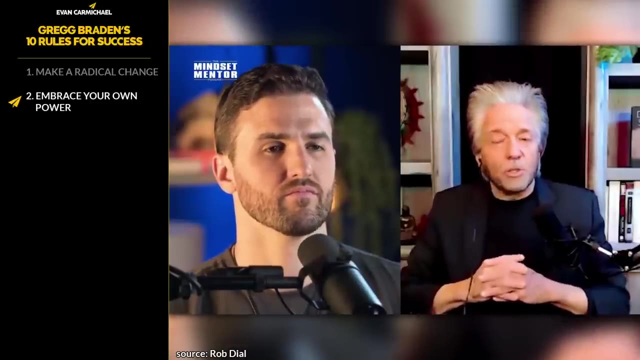 I think one of the most the most powerful acts and the most radical act we can do is to think for ourselves, uh, original thinking based upon the deep truth of our relationship to our bodies in the earth, not based upon the false assumptions of obsolete science that permeate our 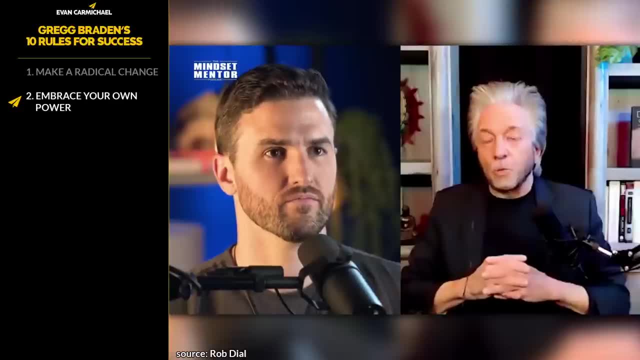 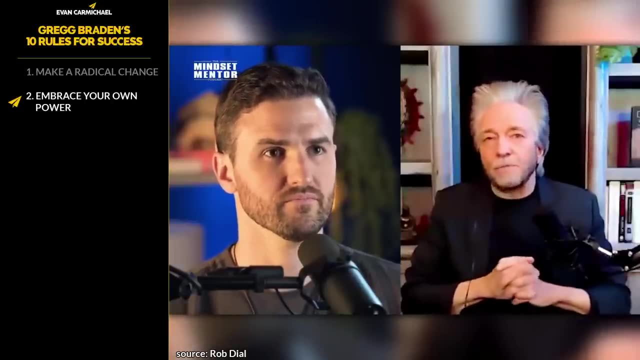 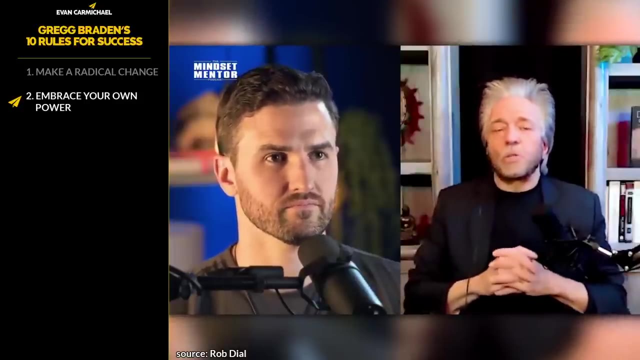 academic world right now. It's one of the reasons I left academia. It's one of the reasons many of my colleagues who are in this genre, who are very well respected scientists, have left academia, because they were not allowed to share with students and in their writings and their papers. 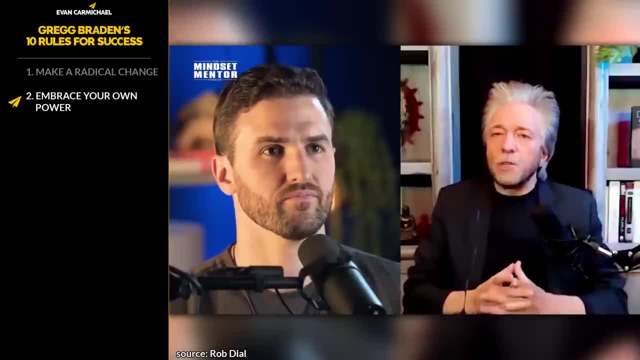 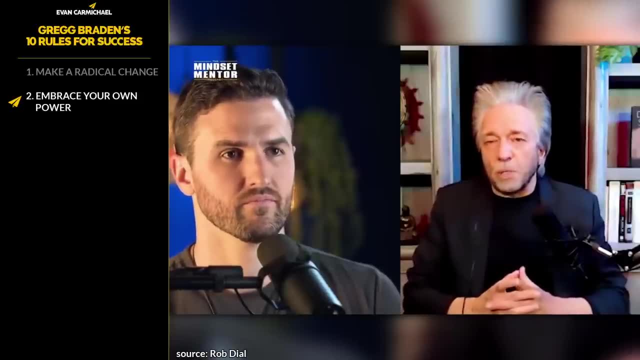 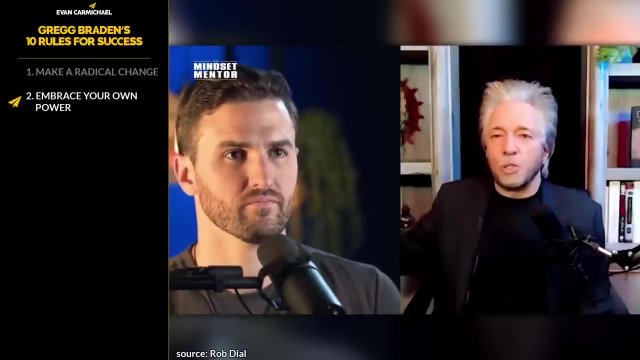 what they had found in their research. that reflects a very different reality. Now, for me, it's- it's- uh, it's good news. It's a beautiful message of hope and possibility, uh, as a sovereign biological being For a system that's based on centralized power and control. 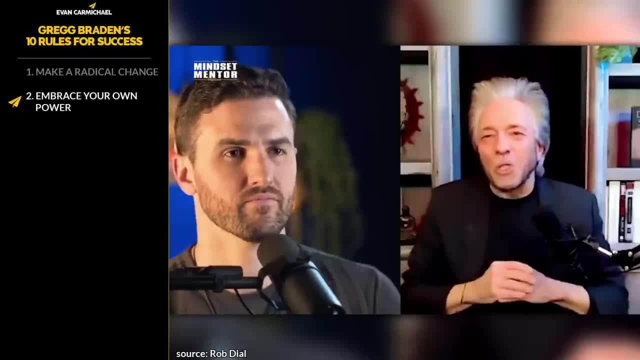 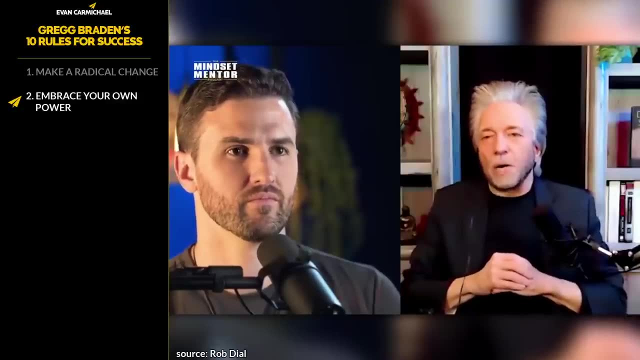 it's probably the worst news they could imagine, because it means we don't need the centralized power and control. I think, ultimately, we're all better off by embracing our own power. uh, because it frees us from the fear of a changing world, And we all know our world. 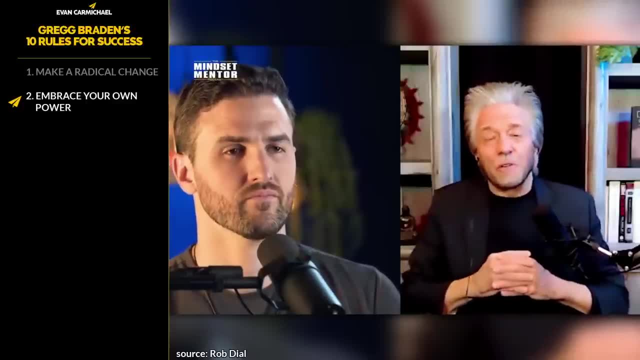 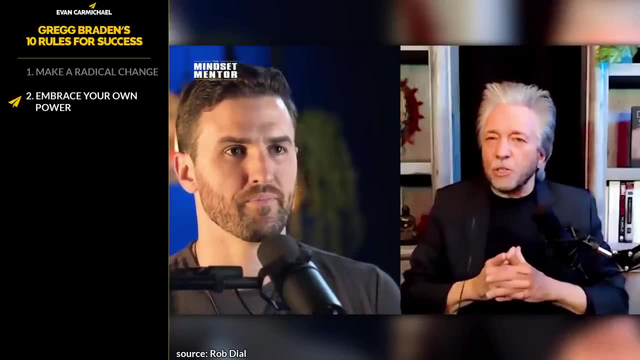 my world is changing. Your world is changing. Uh, noise it ever faster than we can document it in our classrooms and textbooks. But the the change isn't necessarily bad, uh, until we compare it to what we've known in the past. 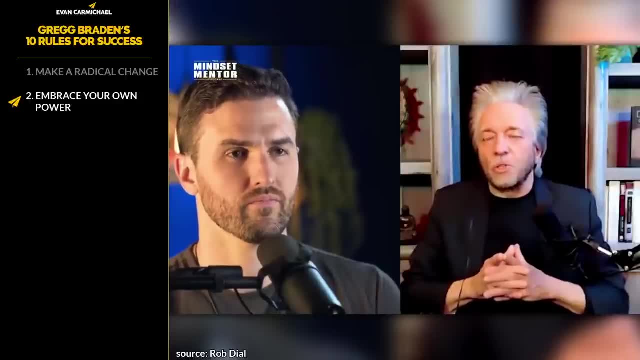 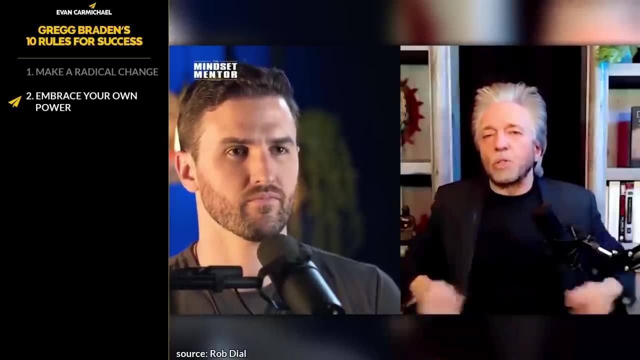 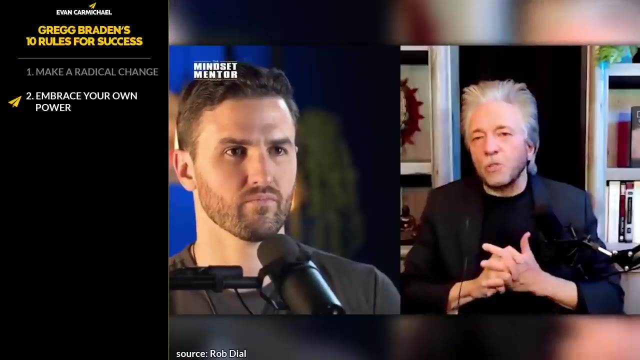 And this is where the fear comes in. So the the new discoveries helping us to understand we are part of, rather than separate from, our world, And this is this is where the affirmations come in. So in um, I was at the CERN superconducting supercollider in Geneva. 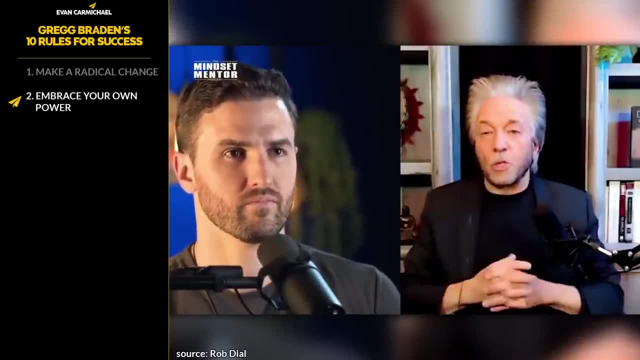 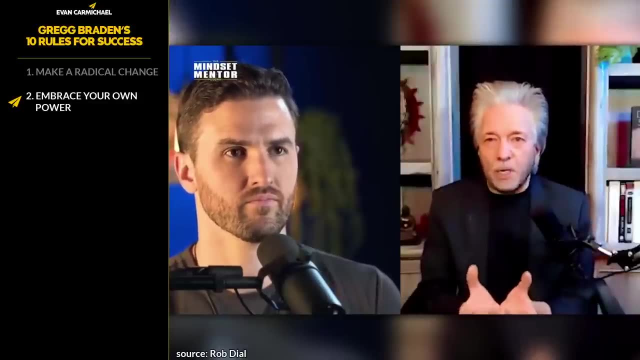 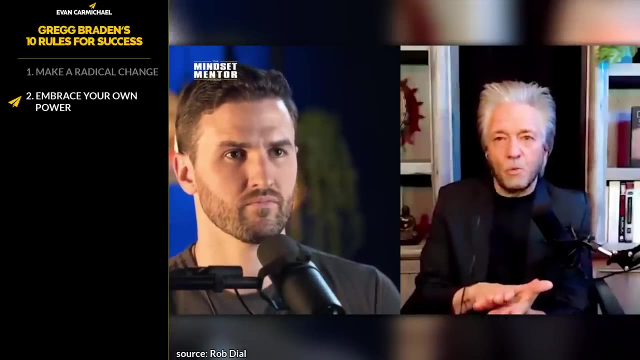 Switzerland, where the the physics experiment, experiments that are revealing what happened moments after our universe began. they recreate the beginning of our universe And then they're able to document what happened then, to create the laws of physics that we are experiencing, that we're living under right now. 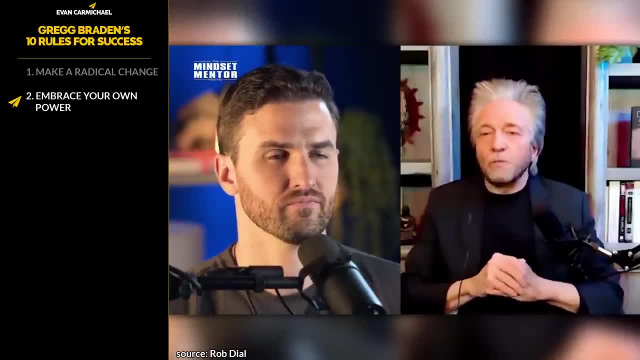 And what they announced in 2012 is that there is in fact, a field, an intelligent field of energy. It's a subtle energy that underlies all of creation. Um, before then it was a metaphor, or a lot of people felt like it was a new age concept. 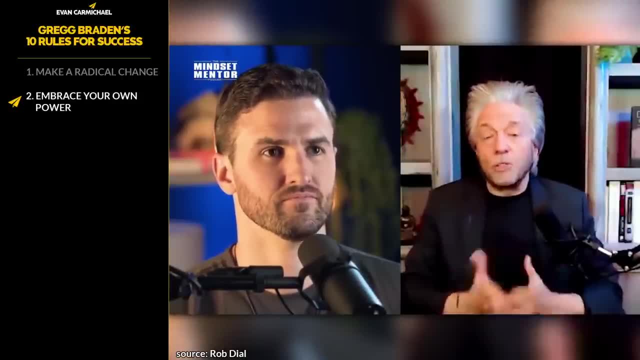 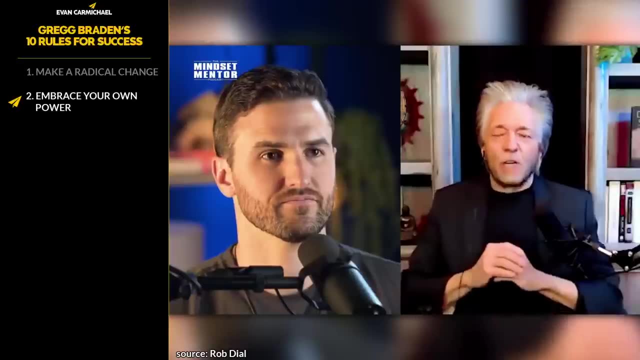 You know, we are all one, Everything is is connected, or an indigenous. you know, a lot of indigenous elders talk about this Here's, here's where they got stuck, And I've gone to scientific conferences where they'll they'll take their hands and they'll say: 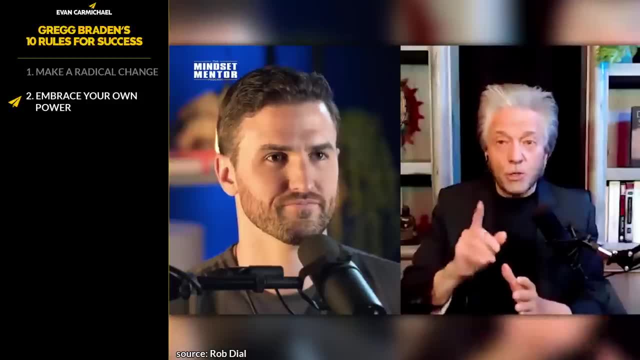 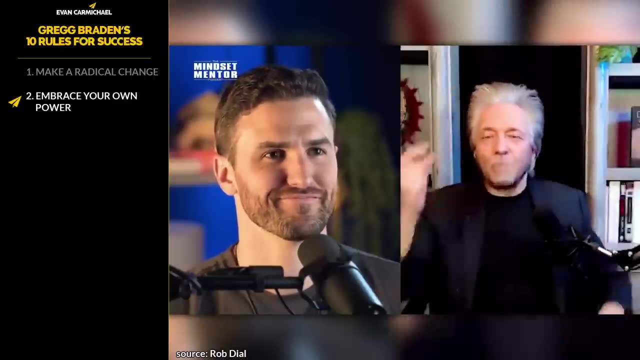 Oh yeah, there's, that's. that's no longer controversial. There is a field, There's a field out there that connects all things and their hands go like this: There's a field out there that connects All things because subconsciously, 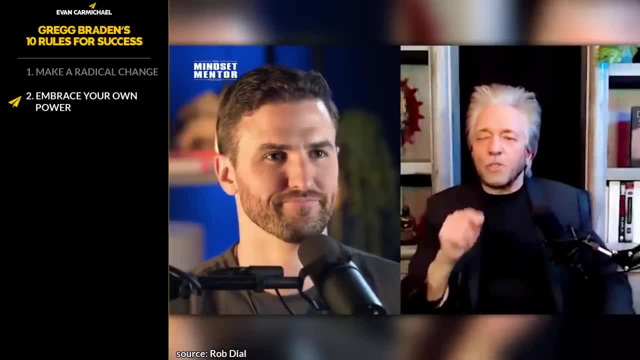 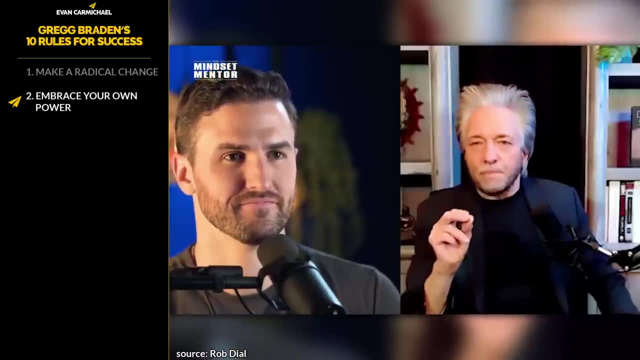 they're still saying we're separate from that field. Right, But here's what the science is showing us And this, this was a game changer for me, Uh, just a mind blower- that every Adam, in every molecule and every cell of our bodies, in this very instant. 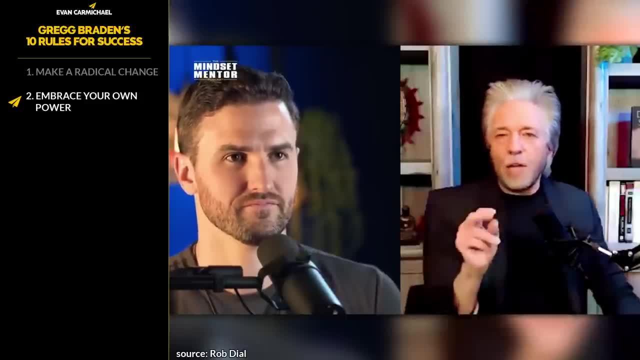 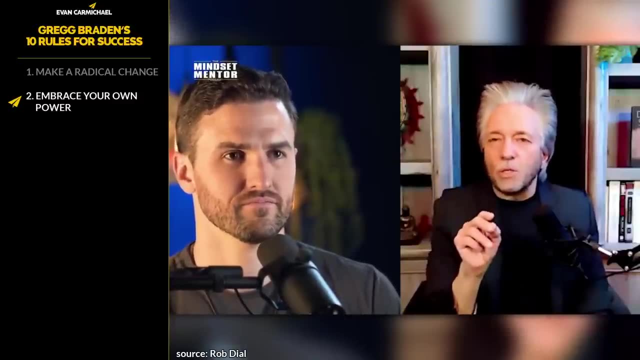 So it's not like it's about to happen. That's it's happening right now. Every Adam is constantly emerging and collapsing into that field, And what that says to us is that we are the field. Yeah, Yeah, Yeah, Yeah. 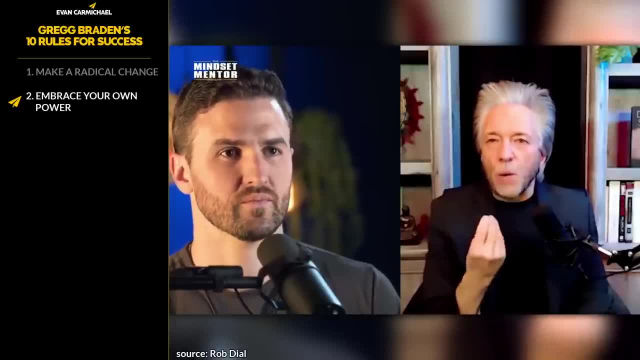 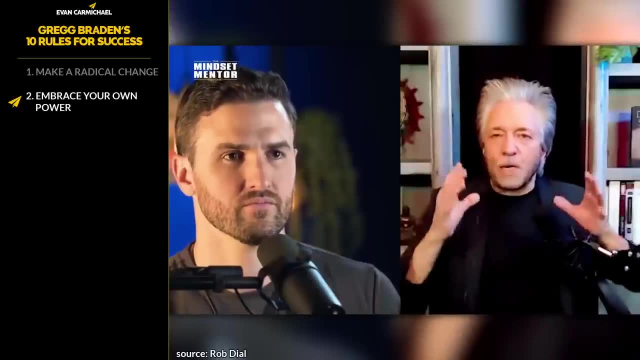 It's not the fields out there. We literally are wrinkles, We are disturbances in this field. This, this body that is held in place by a conscious awareness. As long as I'm breathing on this earth, I am a disturbance, I'm a. 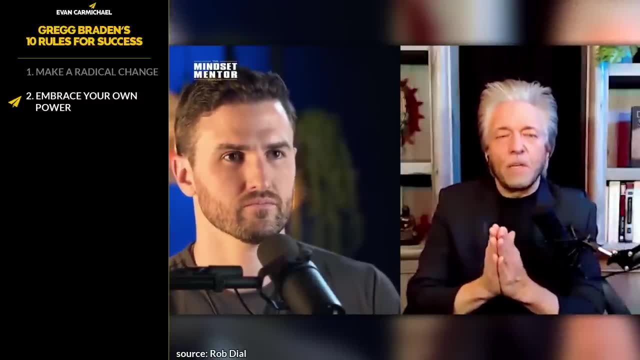 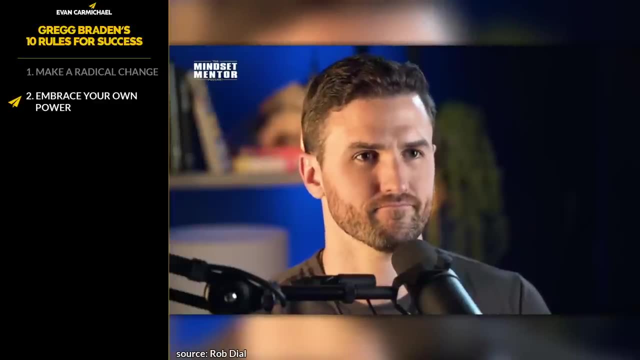 I'm a localized wrinkle in that field, And what that means is that if I want to bring about change in my world, I don't have to force a change out there. I become that change, And as I have become that change. 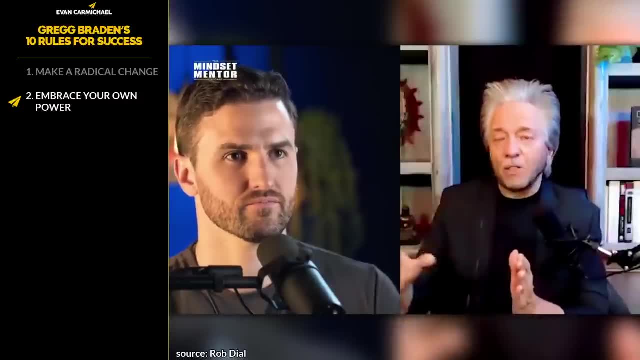 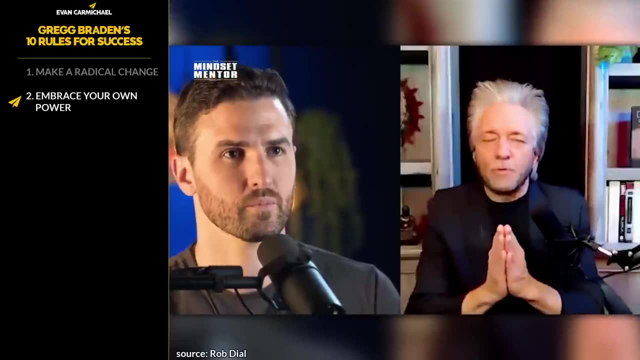 the field is now reflecting what it is because I'm part of the field. So it's a subtle but it's a very powerful way, very different way of thinking. You're not, you're not imposing change on the world around you. 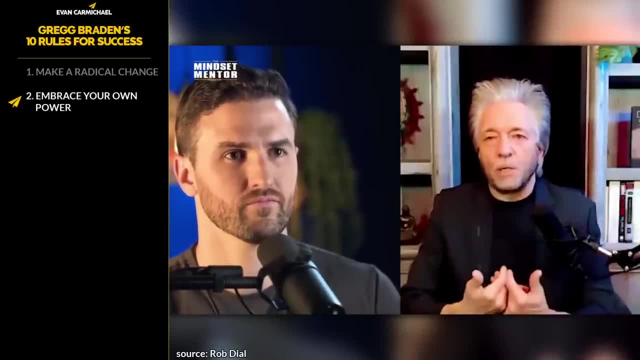 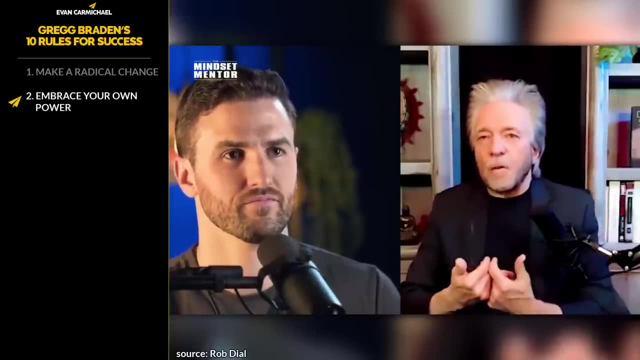 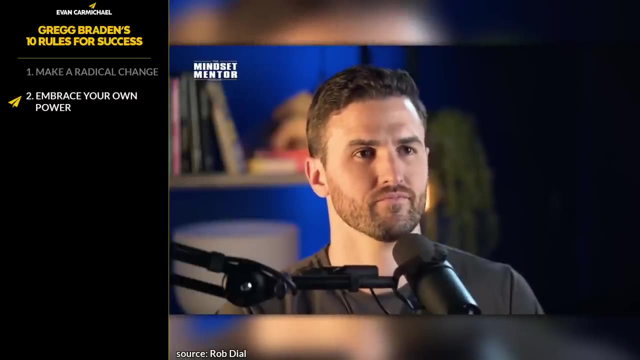 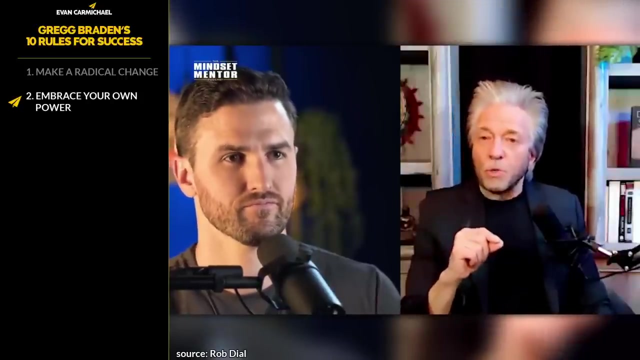 You are becoming the change, So you're becoming the abundance. You're becoming the love, the gratitude, the care, the healing. You're becoming those things, And that is very different. We're conditioned to ask for them, To plead for them, because we're led to feel powerless in our lives, when in fact there are modalities of ancient prayer that were edited from the religious texts in the fourth century by the church. 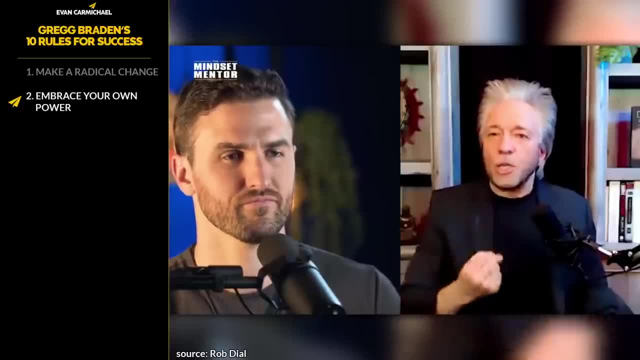 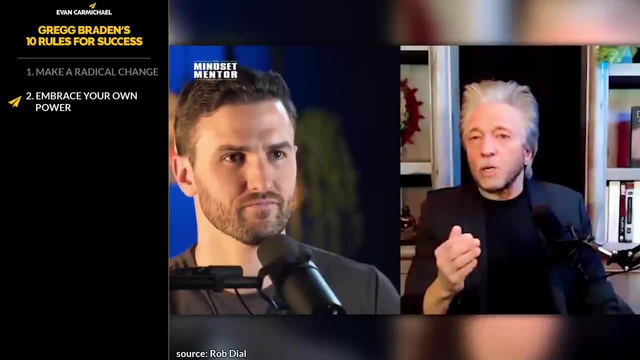 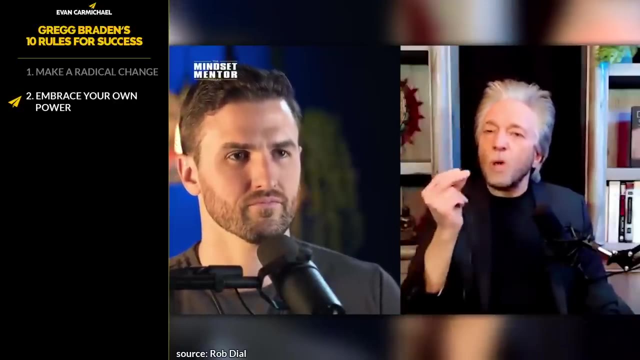 They took. they took out the information helping us to understand that this, this deep relationship, leaving us powerless and and affirmations are essentially a form of prayer, or prayer as a form of affirmation, However you want to look at it, where we are communicating and I want to be really clear. 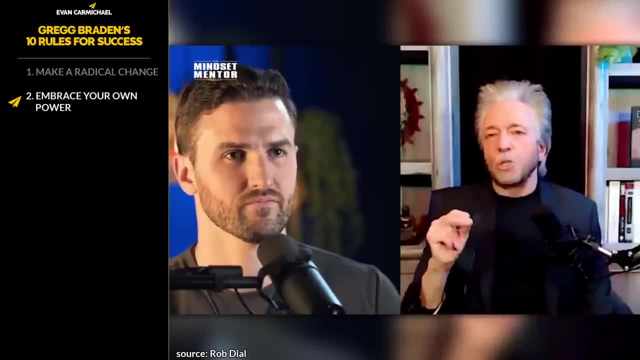 It's not about control, It's not about manipulation, It's not about imposing our will. It's about participating in the way that this field unfolds and expresses in our lives. And when you really begin to get that shift, it's it's subtle and it's powerful. 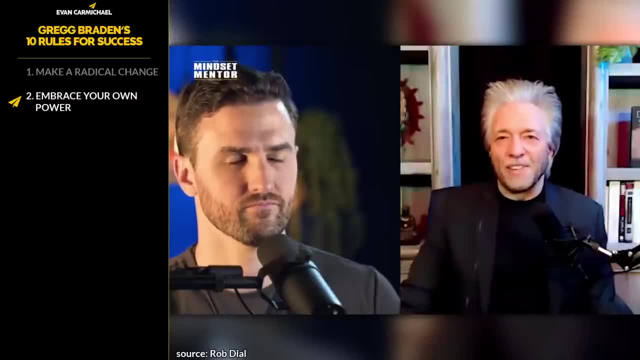 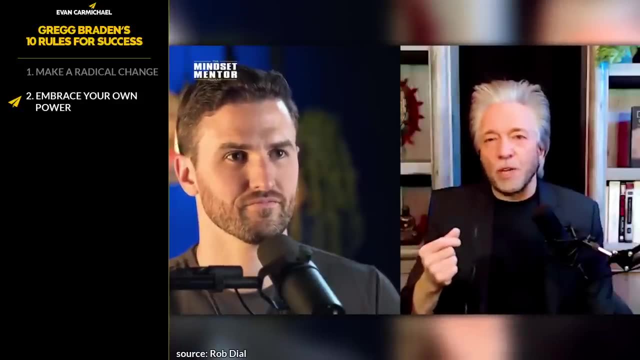 It's not making something happen out there And that means you can't blame what's out there for your, your experiences I I come from a very dysfunctional, broken family and I had to make a choice early in life as to whether or not I would and community, as to whether or not I would allow that to define my 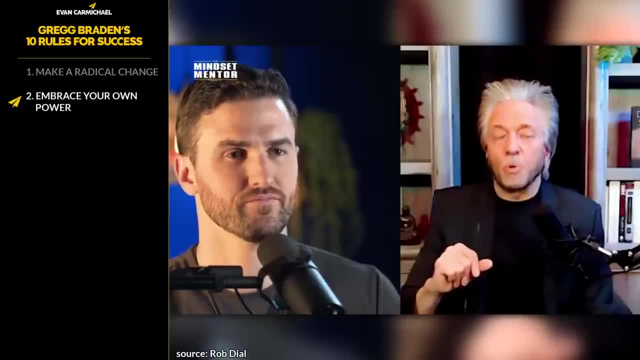 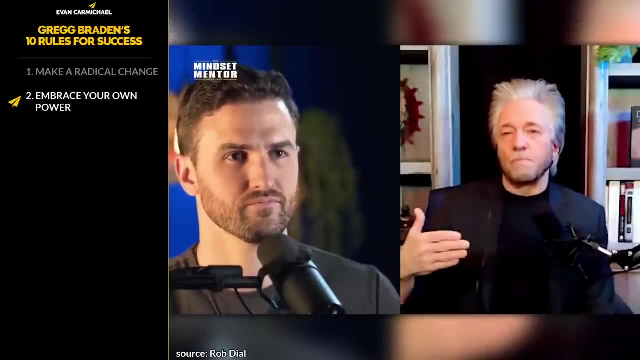 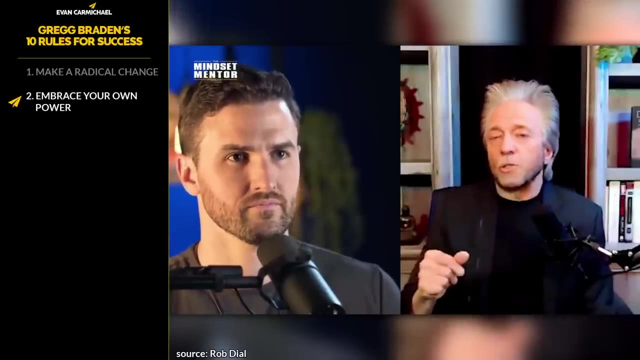 my experience to define my existence. Other people around me had the same experience and they made very different choices. They today continue to blame their environment, their parents, their family, their upbringing, for the sad and unfortunate things in their lives, And that's a path. 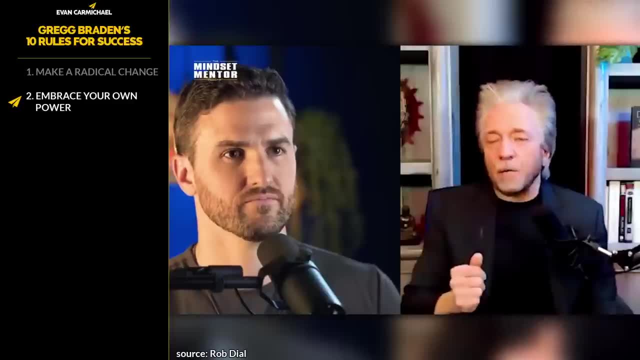 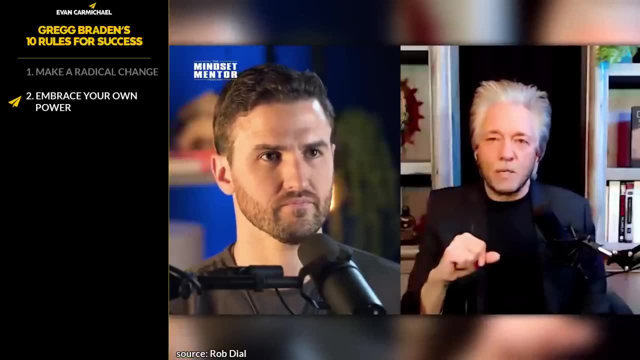 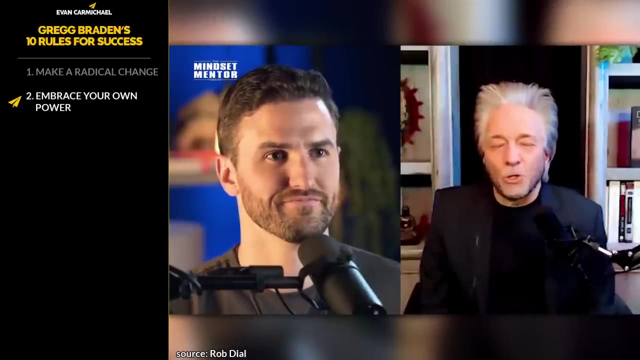 It's not right, wrong, good or bad, but we have a choice to make another path, And when we began, as a scientist, beginning to understand these relationships gave me the reason to think differently, And it also gave me the reason to test in my life if those thoughts are really true or not. 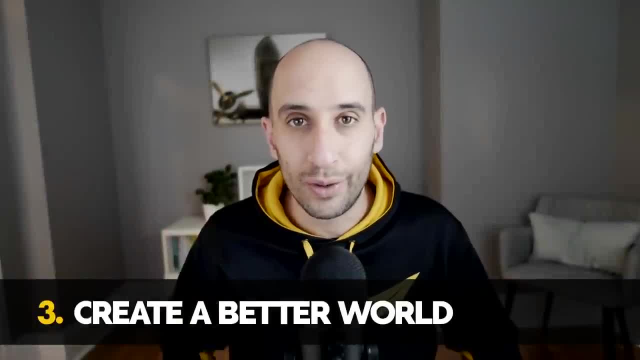 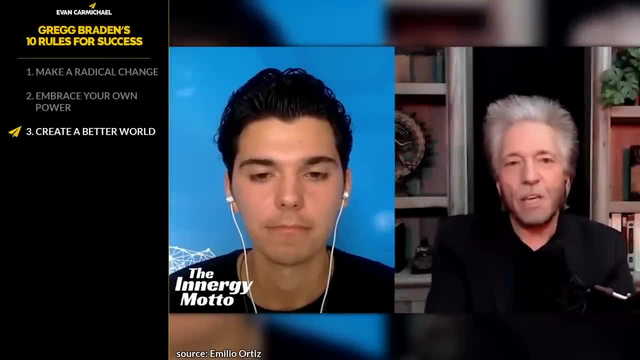 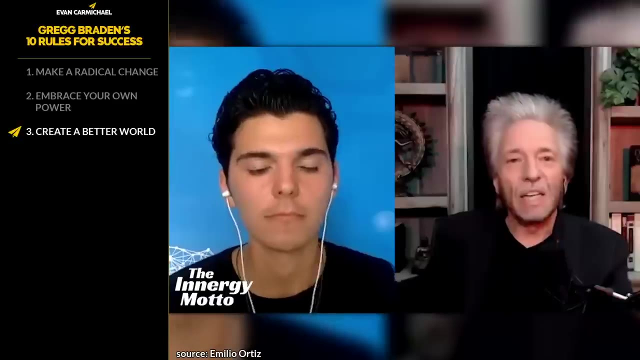 what works and what doesn't. Rule number three: create a better world. What would it mean to have a generation of young people, from the moment they begin in school and kindergarten, from the moment they begin to understand their relationship to the world and the kids around them, to think in terms of cooperation and working together? 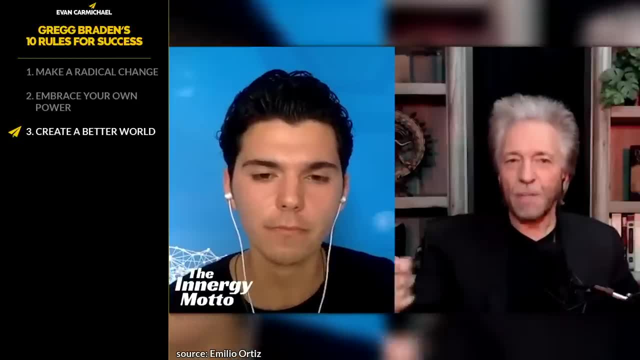 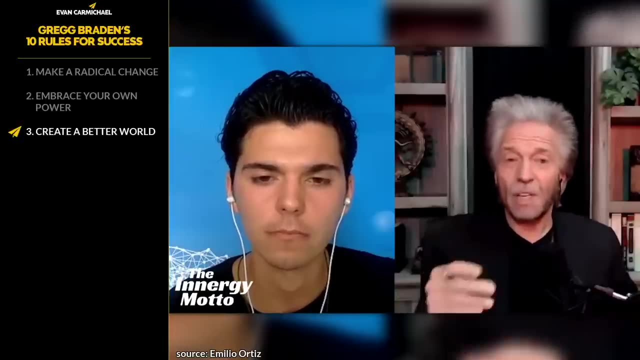 In other words, what can I offer, What can I give, What can I share? How can I contribute, Which is very different from what we're led to believe of. what can I get? What's in it for me? How do I benefit? 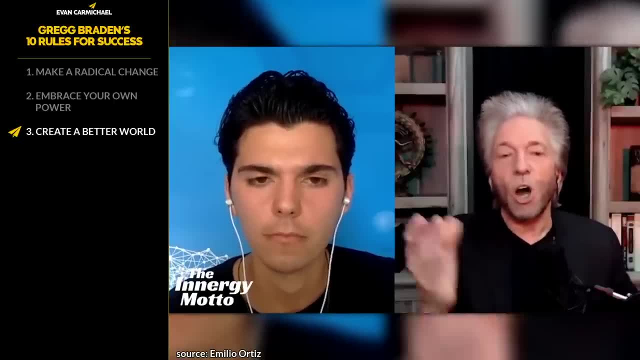 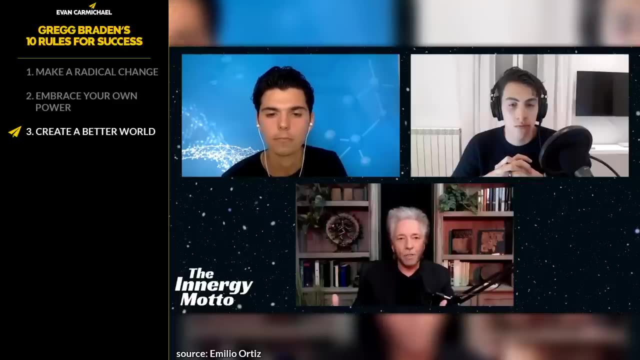 All right, And this is. we are all steeped in this story. So our economic model that's struggling is based in the false assumptions of competition and conflict. Our corporate model is based in everything, everything. So it's up for us right now. 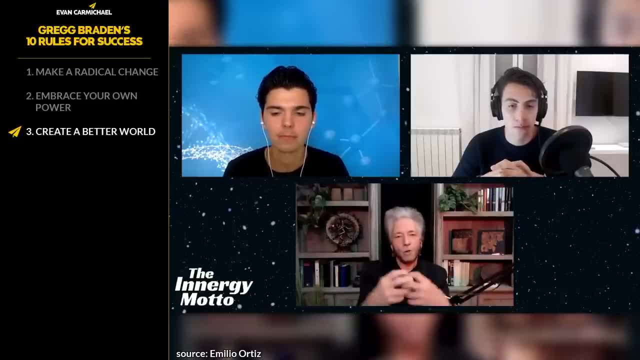 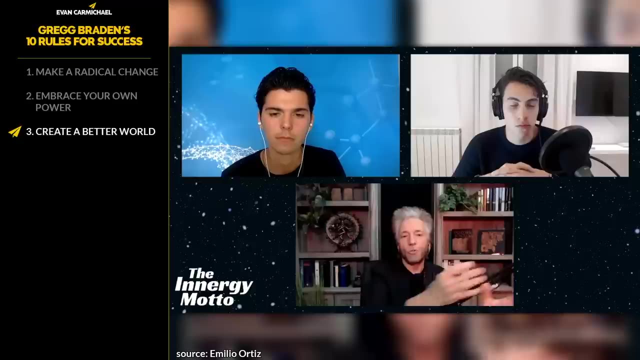 So this, this right now, we're living this rare convergence of the cycles that have changed the world as we have known it and the new world that's emerging. the struggle and the suffering comes from us trying to embrace that world through the old thinking of false assumptions, of an obsolete science. 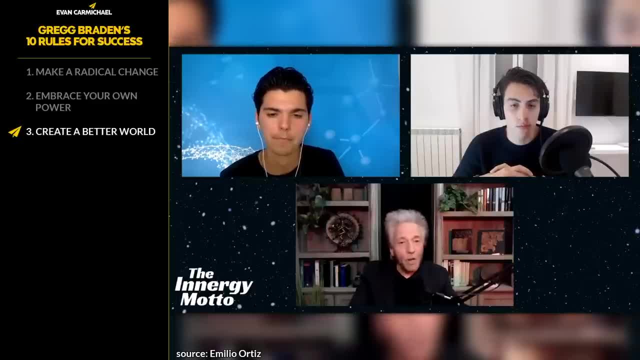 Now we've asked science to tell us who we are, and science has done a really good job. There are a lot of scientists that don't like the answer. Yeah, Science has been hijacked by corporations. They cherry pick the data by politics. 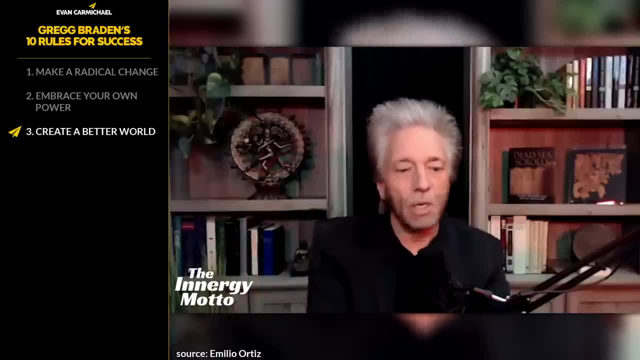 They cherry pick the data. Climate change is a perfect example of how that's happening. Science- Science has been hijacked by corporations, by politics, by religion and by academia for reasons of money and power and ego and habit, And this is where we find ourselves now. 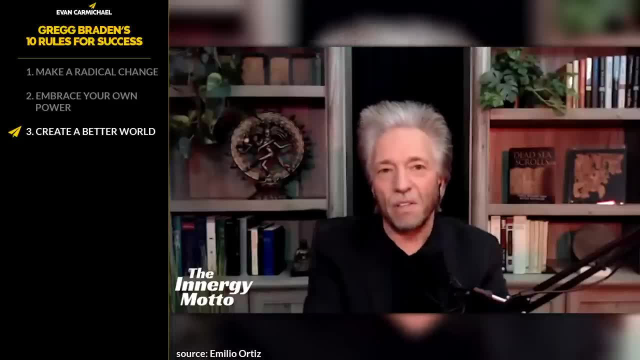 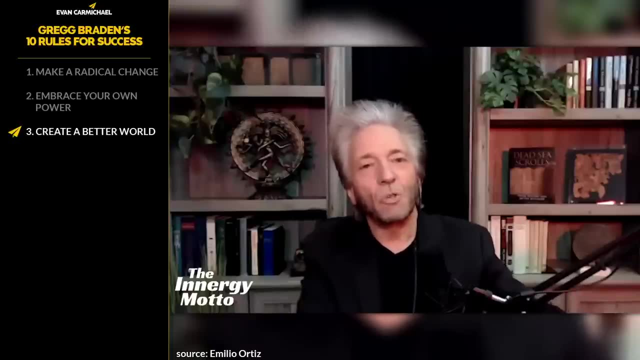 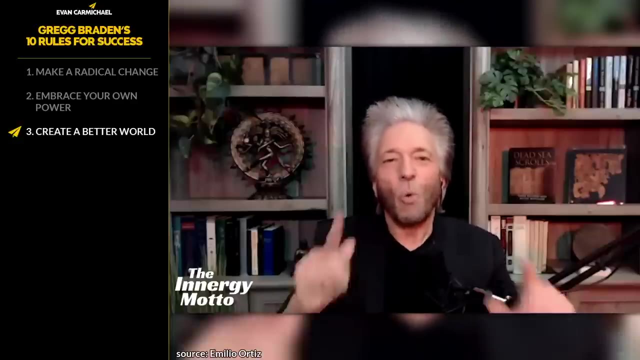 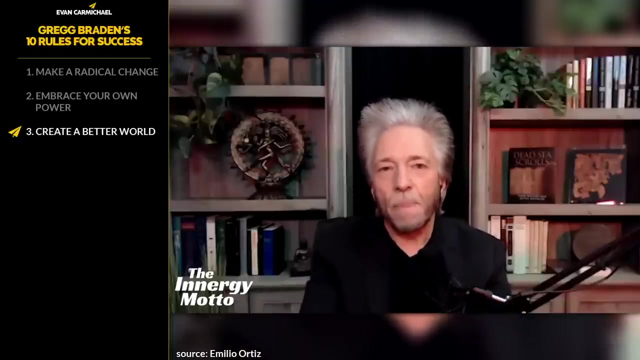 And I believe that we're witnessing the breakdown of these old structures, these old ways of thinking, because we're living in a new world And this is- and then I'll stop here- It takes one generation. One generation has to be the generation that lives the old world that is crumbling and 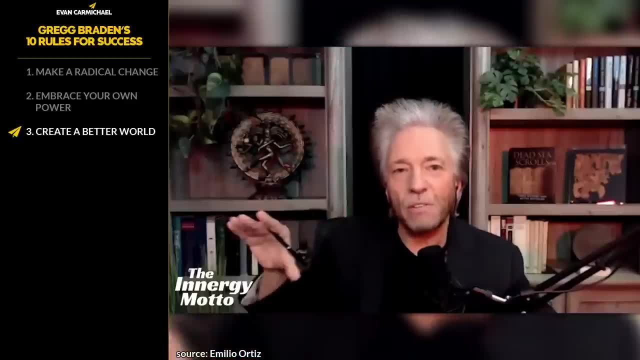 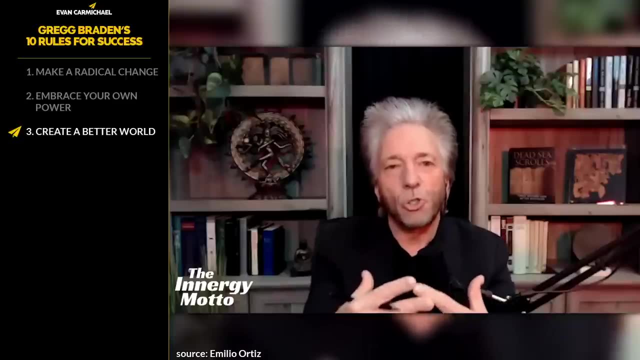 also lives the new world that's not quite fully developed yet. So you're living in between these two worlds and it takes a really strong person or a strong family Or a strong community or a strong nation or a strong planet to live in this in-between. 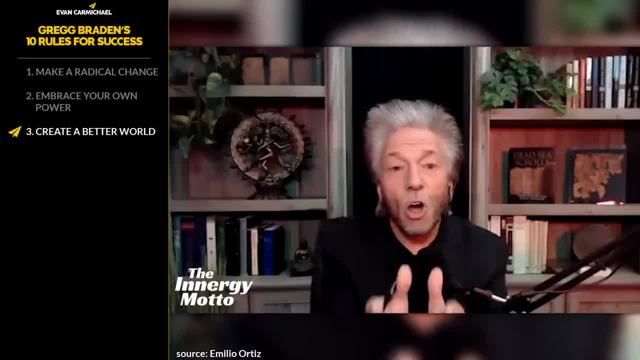 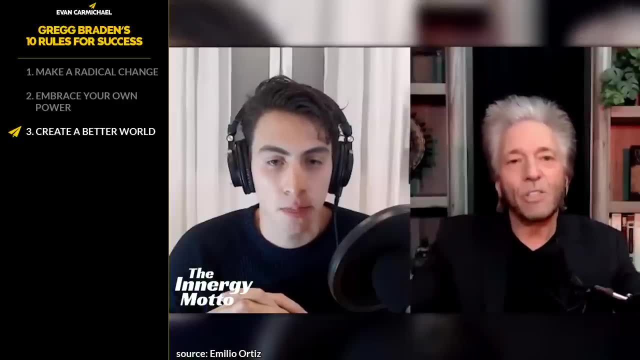 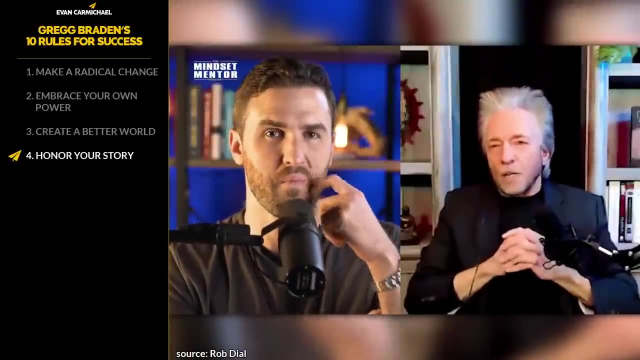 time without getting lost in the fear of the unknown. Yeah, This is where the new human story comes in, because the new science is giving us the reasons not to fear. Rule number four: honor your story. I went to my first rock concert, Jefferson Airplane, the original Jefferson Airplane. 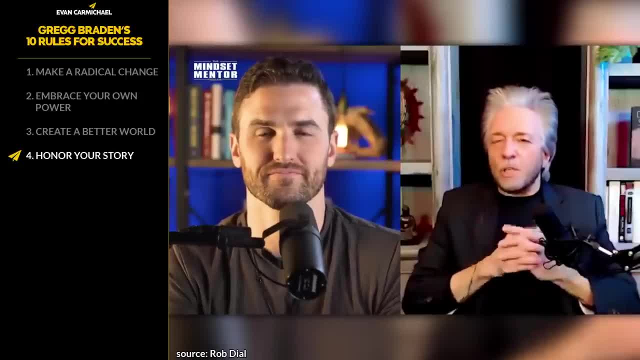 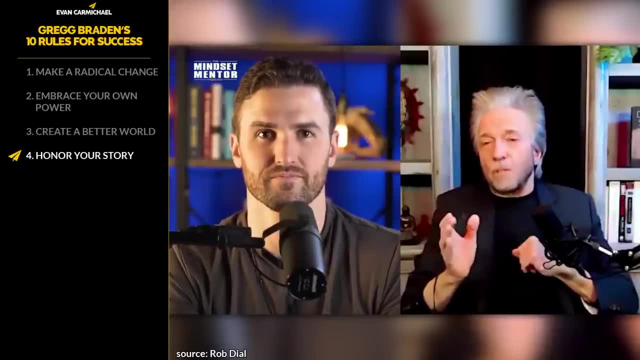 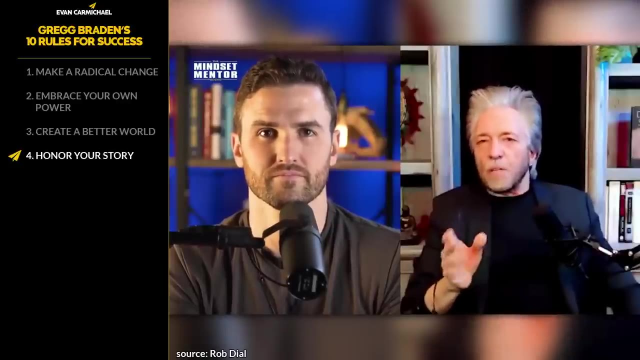 And what I saw, Rob, I'd never seen anything like this. I saw this group of people on a stage influence the way that in that venue it was about 30,000 people, So they influenced the way that those 30,000 people were feeling in their lives. 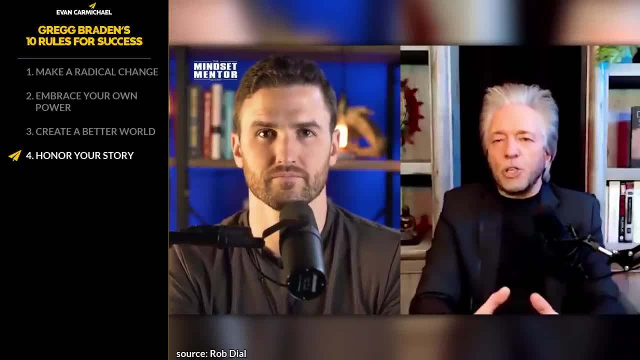 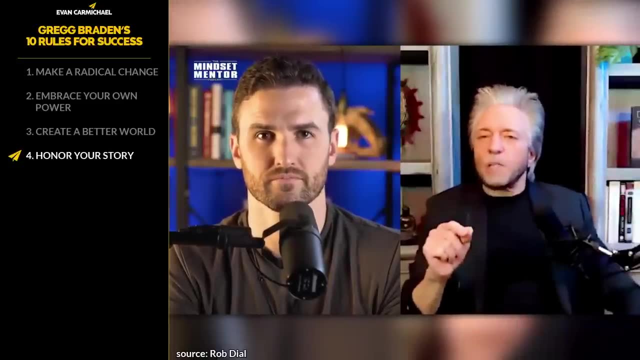 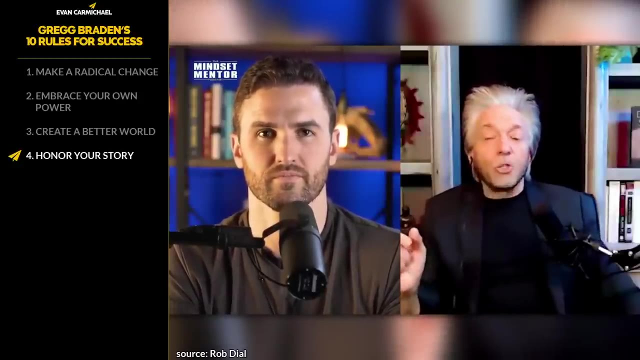 That group of people had the ability to shift the emotion and the feeling inside of the people that were in that room And I recognize that. but I also recognize that when the concert was over, when we left- we weren't outside- that feeling began to wane very quickly. 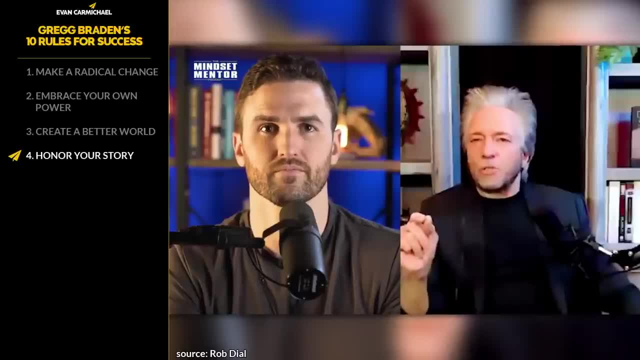 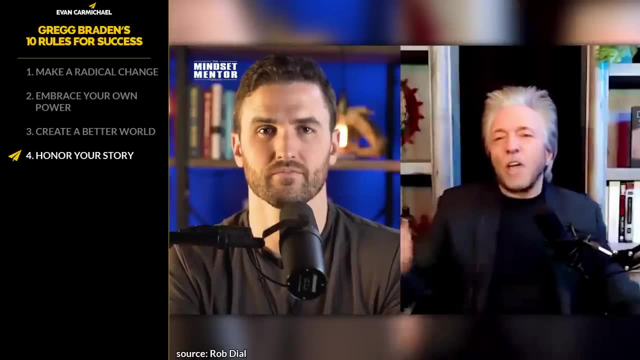 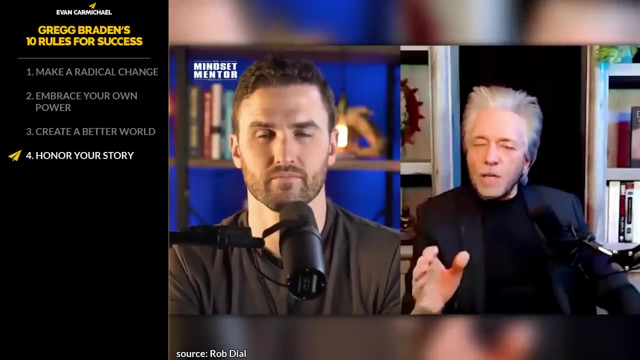 And the people needed something outside of themselves to create that feeling again. In that time they were vinyl records and cassette tapes. They needed to have something to respond to for them to have the experience. Well, in the same year I also had the opportunity to see another. 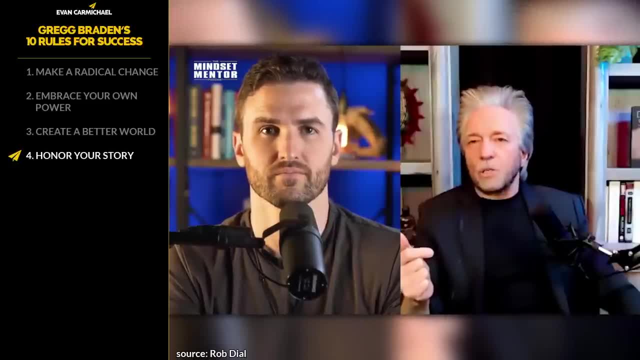 It was an event in a stadium. It was an event in a stadium with about 70,000 seats and a speaker named Billy Graham, And it was a religious-oriented talk And I have to say honestly, I wasn't totally into everything that was being said. 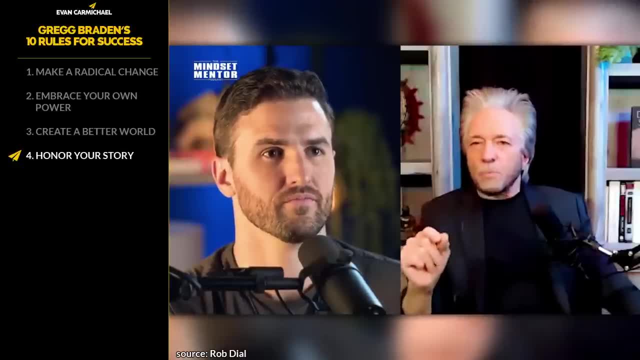 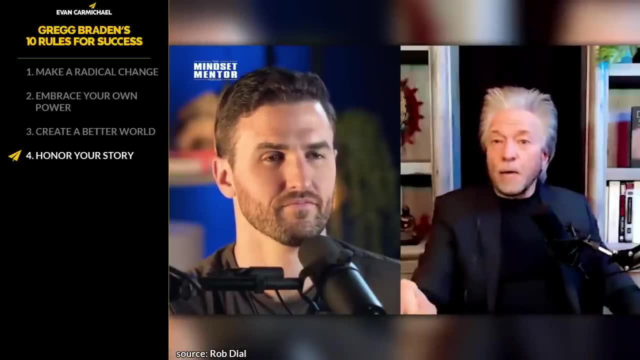 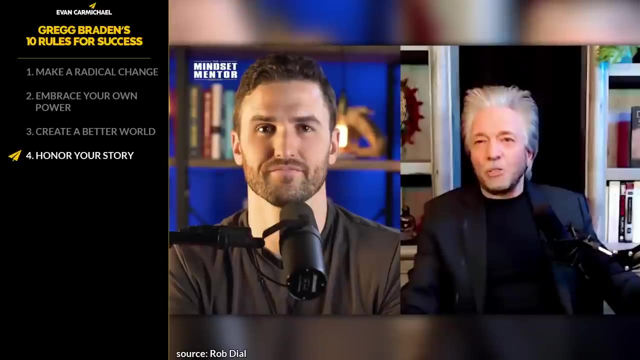 But what I saw was a stadium of 70,000 people And they were being moved on a deep level by the words of one man on the pitcher's mound in this outdoor stadium. It was amazing. It was a Kansas City Athletic Stadium, the A's Stadium in Kansas City, Missouri. 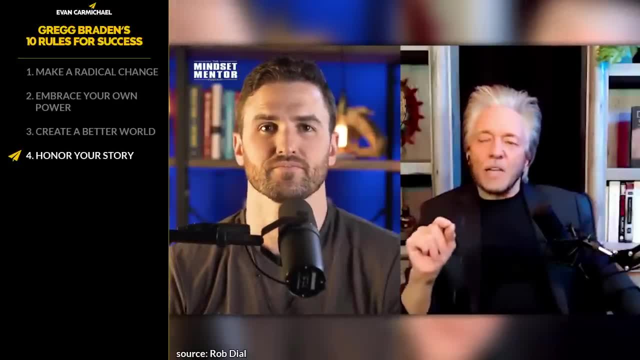 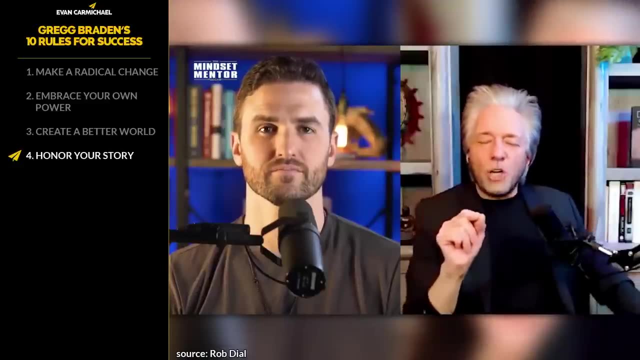 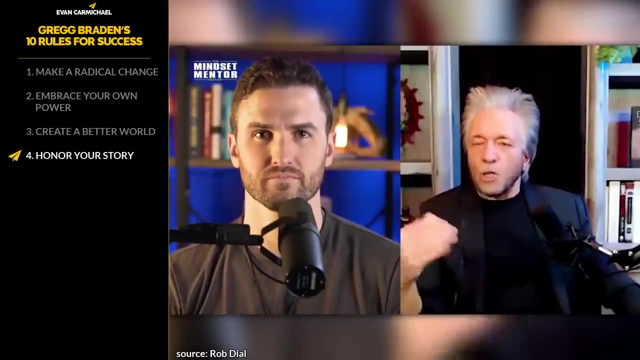 But here's the difference: When we left, they did not need something outside of themselves to maintain that feeling, because his words had changed the way they felt about themselves and their relationship to the cosmos, to God, to one another, to the earth, to their communities. 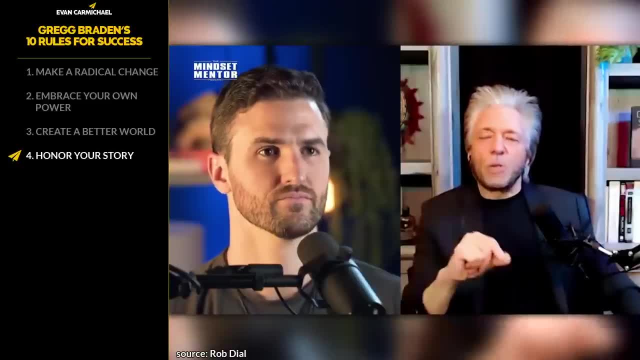 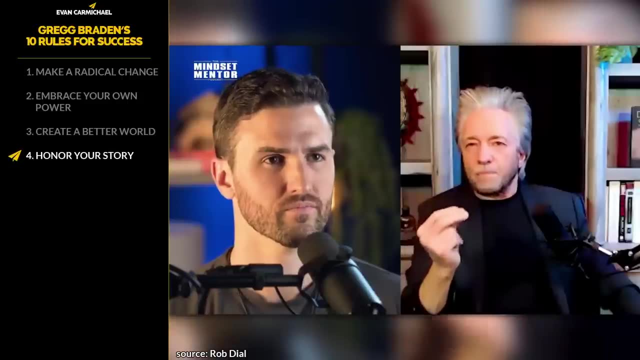 And it stayed with them because they were changed in the presence of his words. Hmm, And I recognize that. I recognize both those In early age, and I thought there's got to be a way to combine these two, the music and the sound. 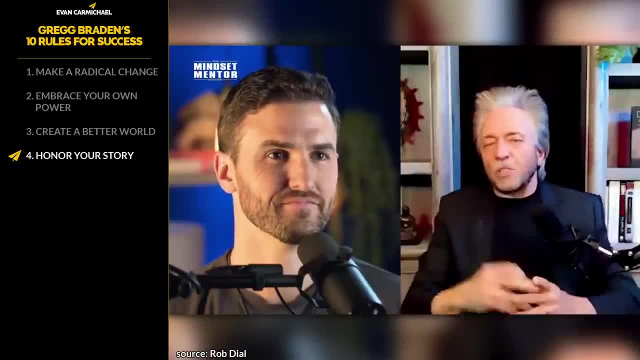 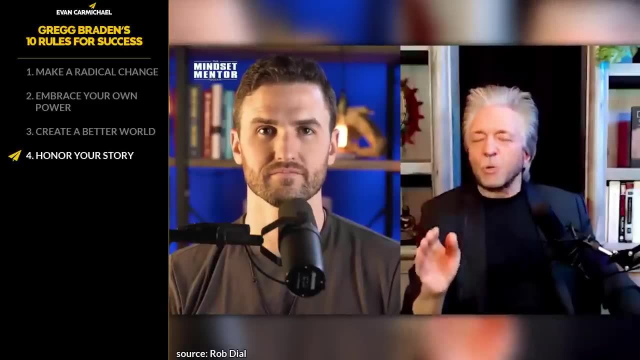 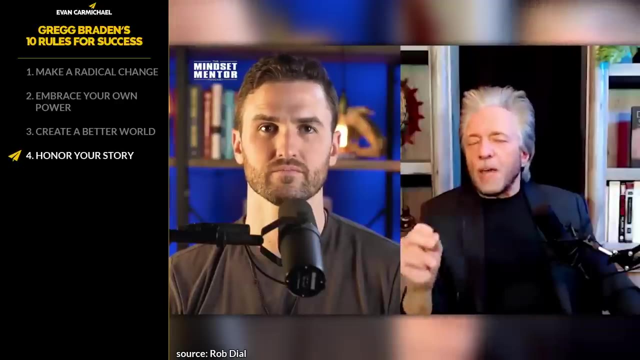 I'm still searching for that. But the science? the science gives us a reason to think differently about ourselves And it's based on honest, truthful, factual information. if it's good science, Mm-hmm. And from that we begin to think of ourselves differently and we are changed in the presence. 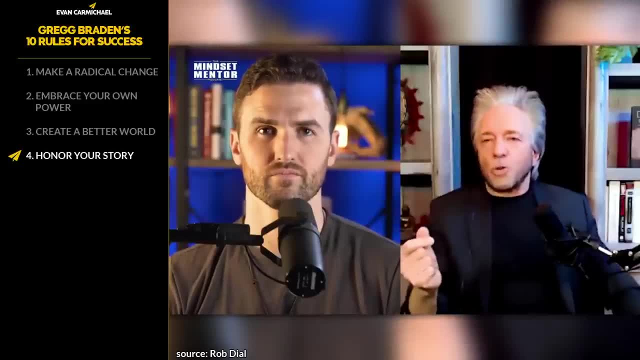 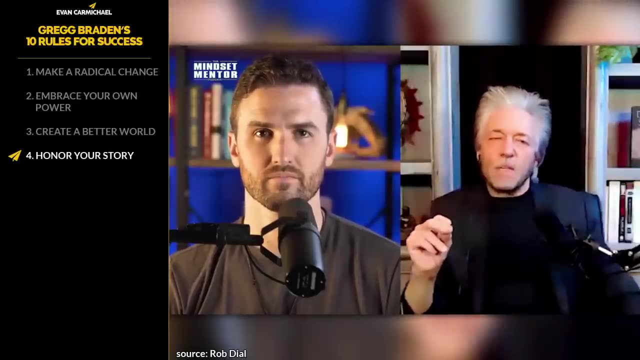 of new understandings. It all comes down to our story. What we're talking about is our story. It doesn't have to be technical, but our story, our lives literally, are based upon our story. We solve our problems, We choose our relationships. 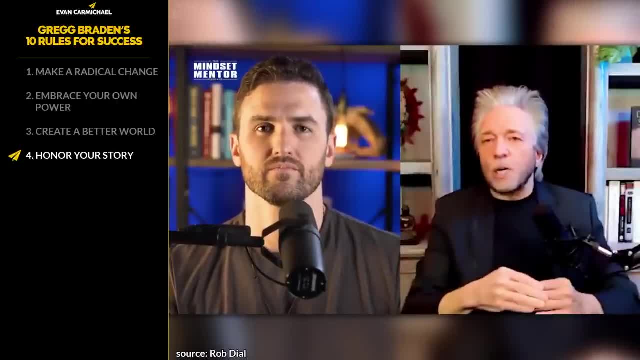 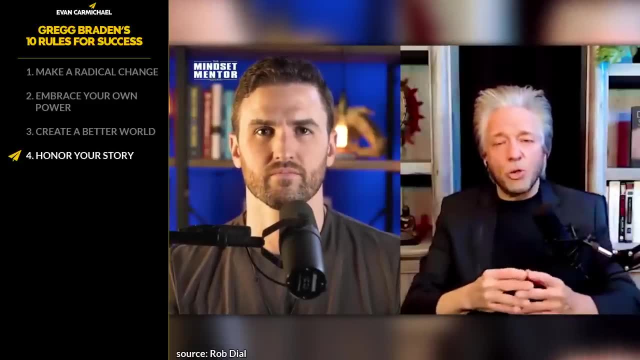 We heal our bodies, We choose our politics, We build our society- all based upon the way we've been taught to think about ourselves. And what's happening right now- and I think we all know this is our story- is changing Mm-hmm. 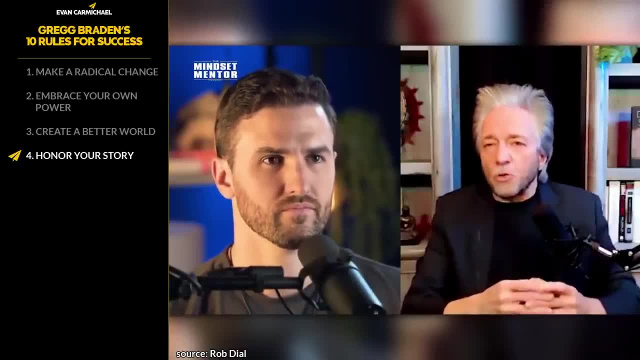 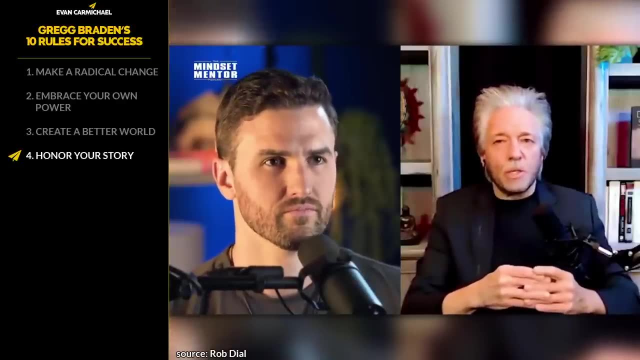 And it? There is a battle, Rob. There's a battle for our story. There's a battle for our thoughts, for our beliefs. There's a battle for our very humanness that is unfolding and it's happening right in front of us. 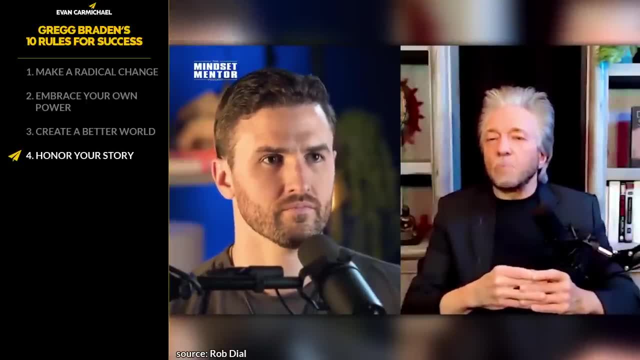 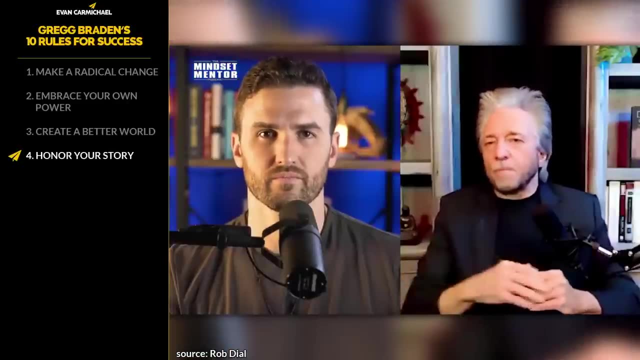 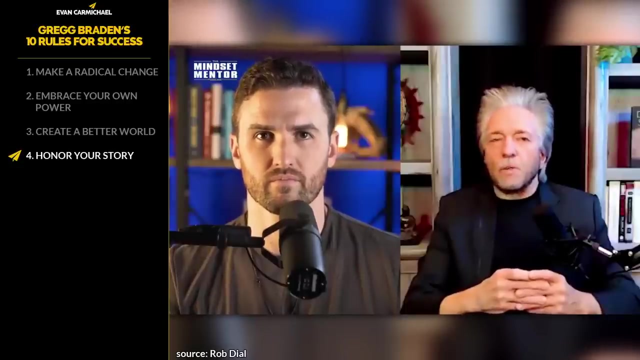 Many people don't recognize it because it is compartmentalized, but it is happening right now on the mainstream of the world stage. So I go back to those experiences as a scientist today, through the eyes of what I now know, and I know that the most fundamental act, the most radical act of empowerment that any 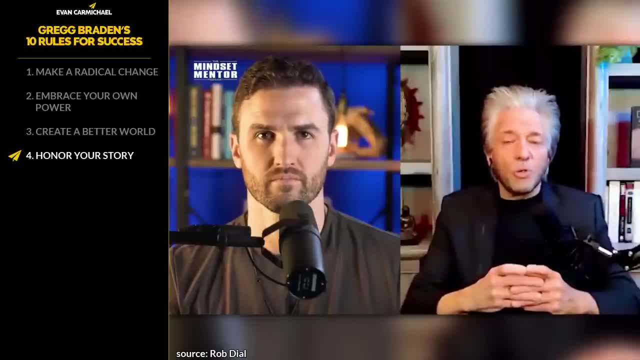 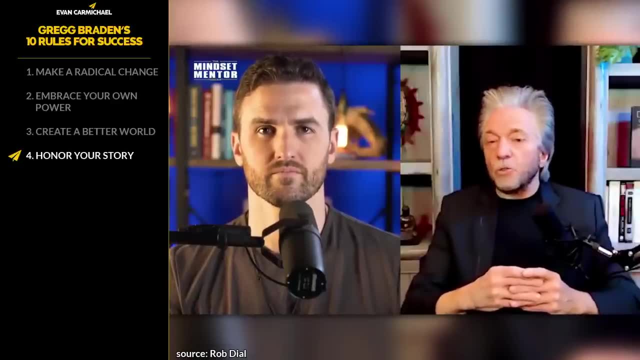 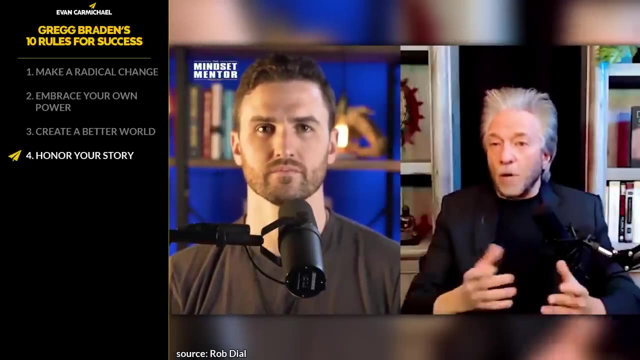 of us can embrace is to honor the deep truth of our story. not the story necessarily that we've been coerced into accepting or believing. not the story. maybe that came from our family or our religion or our education- you know academia- or our political affiliation. 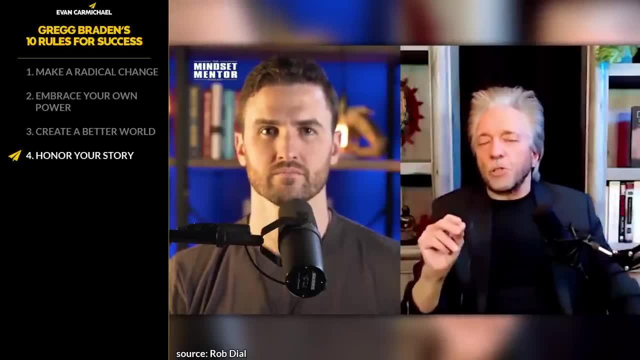 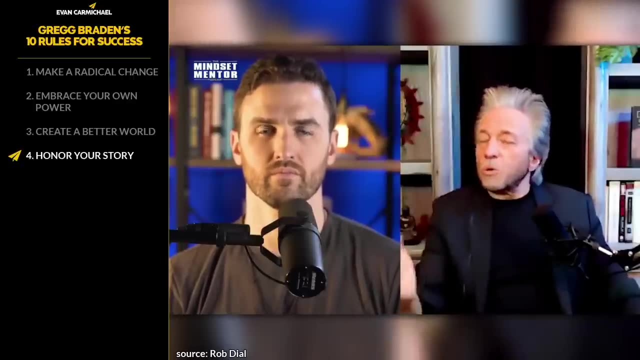 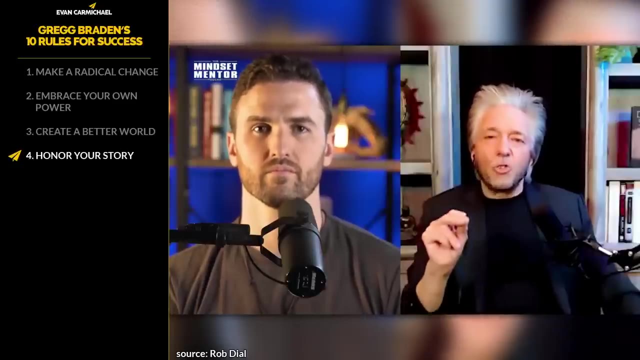 But the true story of our relationship with ourselves, with the world around us, with one another, with the past, with the future, with the cosmos. and if we believe in a higher power and in the presence of that story, we are changed and that gives new significance. 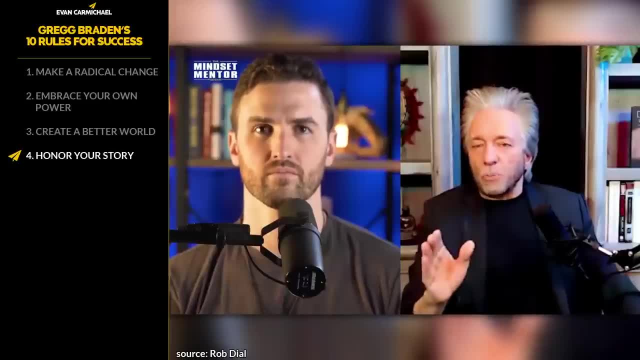 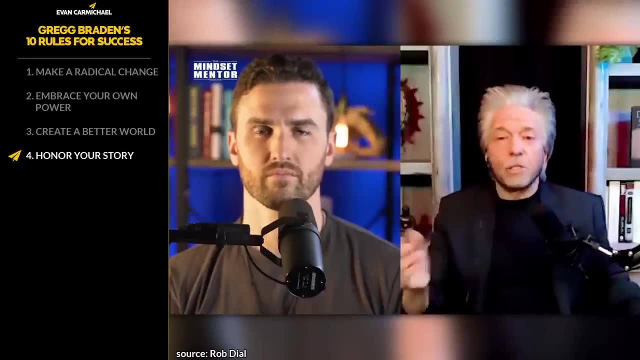 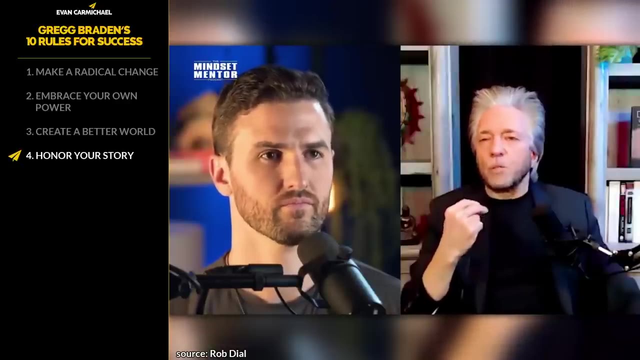 to what's unfolding in our lives. It's a celebration that moves us from the fear into the freedom of self-mastery, and the science is now telling us Literally the self-regulation of our own biology. What could be more powerful than to be able to self-regulate, up-regulate and down-regulate? 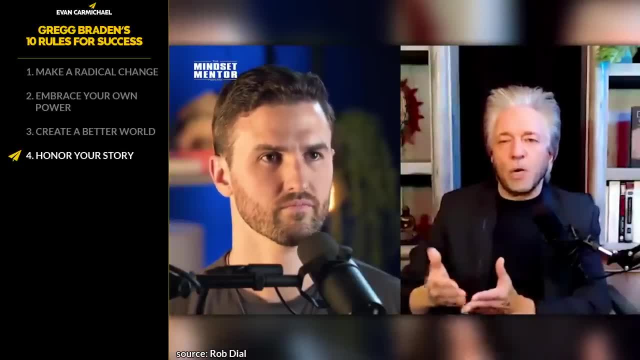 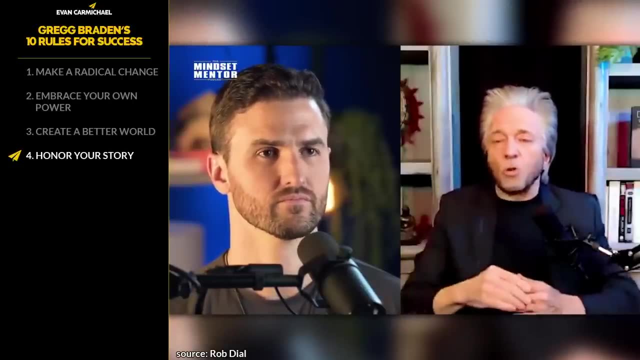 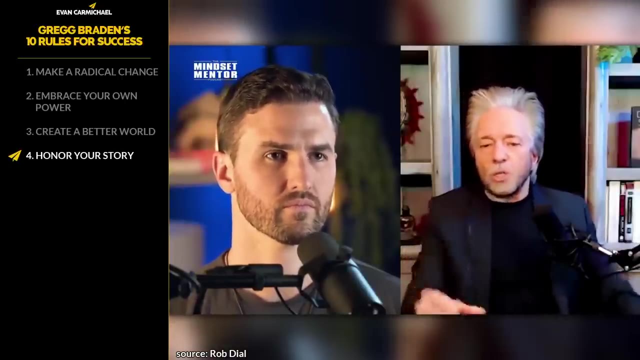 genes to enhance your immune response. on demand, to awaken longevity enzymes. on demand to create resilience to a changing world. on demand, deep states of intuition and so much more. What could be more powerful than to awaken to that possibility now, in the presence of? 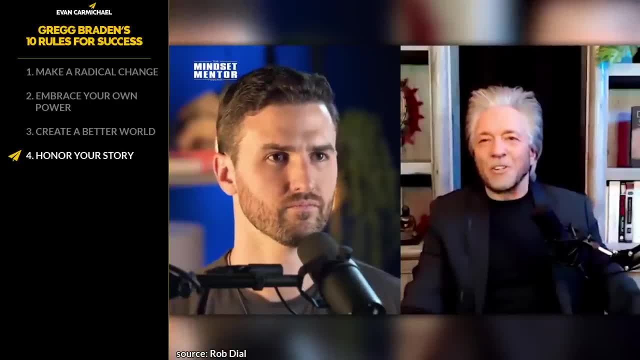 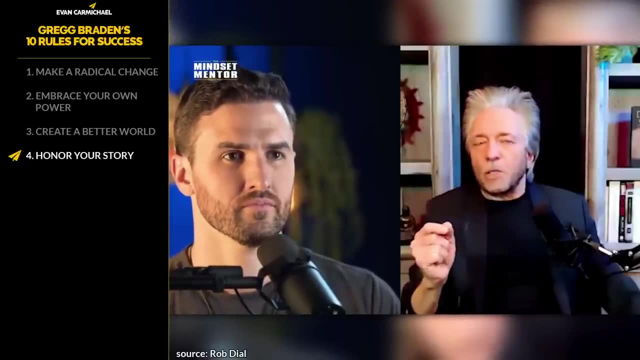 a world that is changing, A world that's changing faster than we can document it in our textbooks. So it's a long answer to a short question. but the science for me. I recognize in early age that it was a language that would help me personally to understand my relationship. 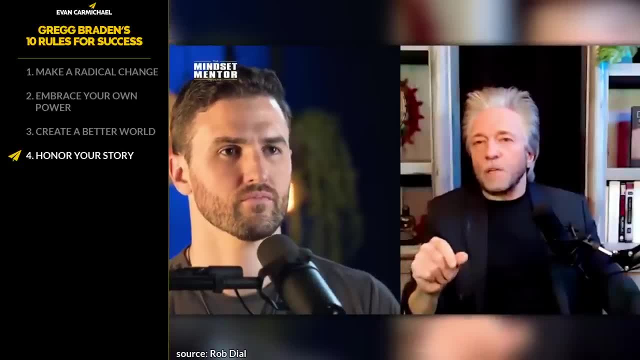 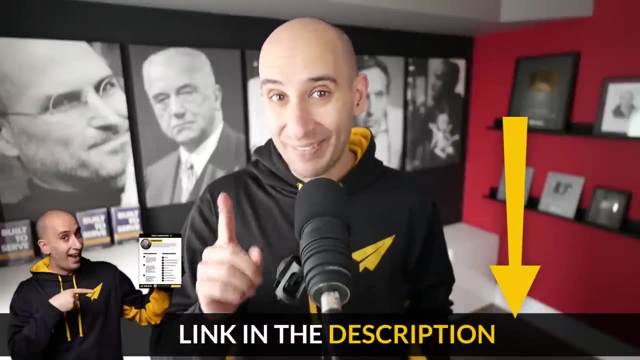 to the world that I was drawn to and it comforted me in times of extremes, and I think that's true for all of us today. Also, to make sure you're actually taking action after watching this video, I've designed a special free worksheet. 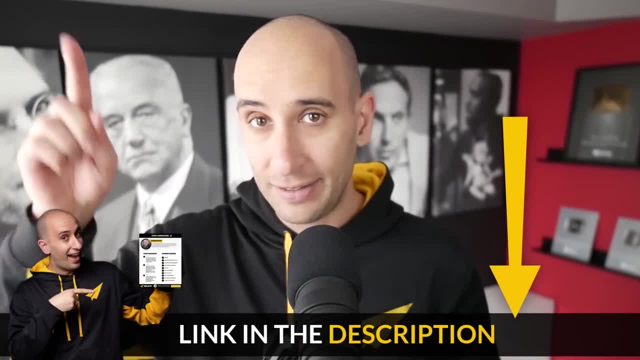 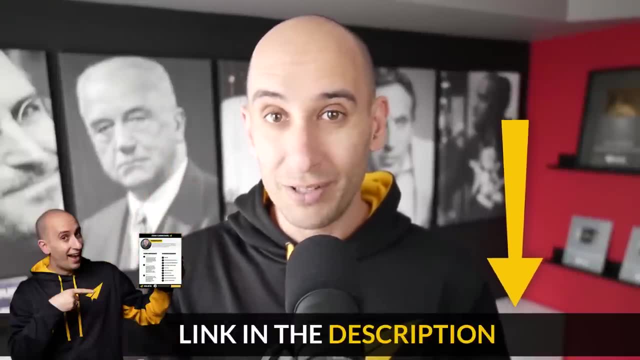 Just for this video. the worksheet will highlight all of the lessons learned in this video, as well as pull out our three favorite learnings and quotes that will inspire you to actually do something. The worksheet will also give you space to write down what your key takeaways are, and. 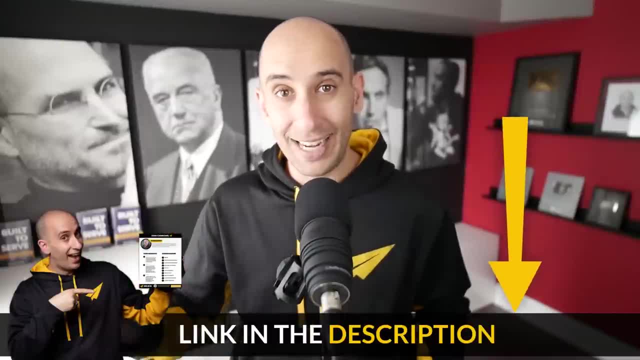 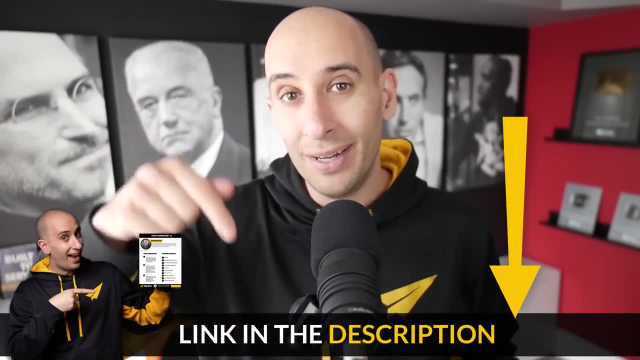 your specific plan of action to make sure you're getting results. If you want the worksheet designed specifically for this video, absolutely for free, there's a link in the description below. go click on it and start building the momentum in your life and your business. 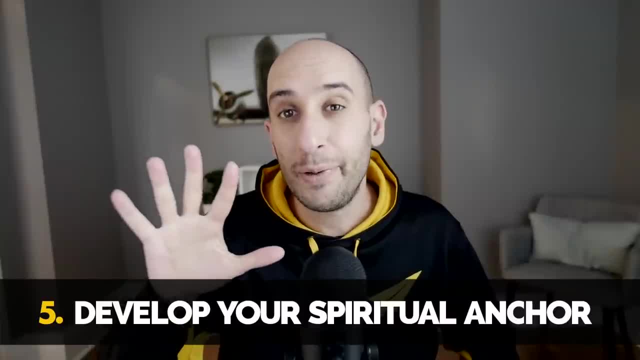 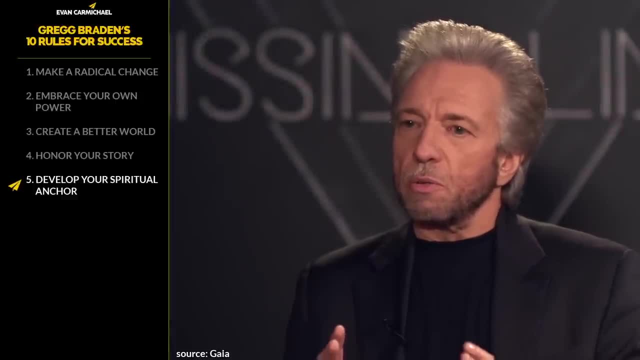 I'll see you there. Rule number five: develop your spiritual anchor. Every one of us, in our own lives, we have to develop what I call the spiritual anchor, the rock, the soul compass, and it has nothing to do with religion. 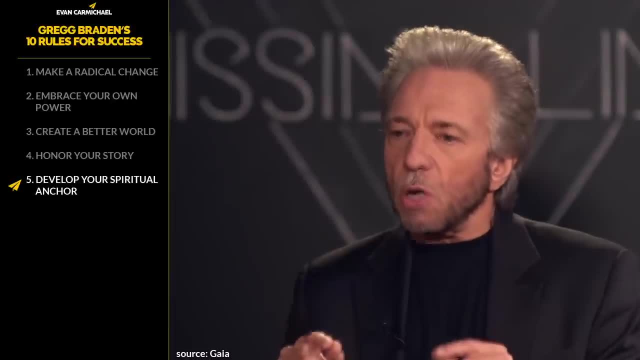 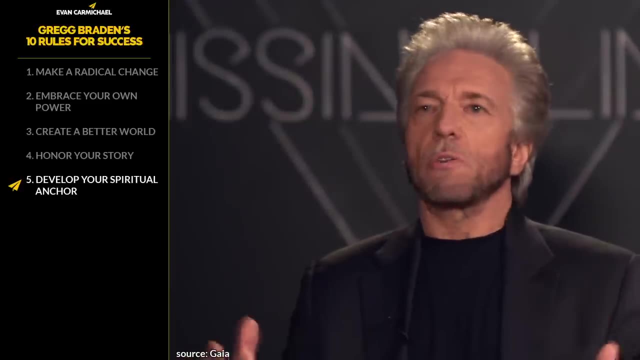 When I say the spiritual anchor, the spiritual anchor is when we know who we are in relationship to ourselves. We know who we are in relationship to the earth, to one another, to our past, to our future. We know how we are empowered and what our potential is. 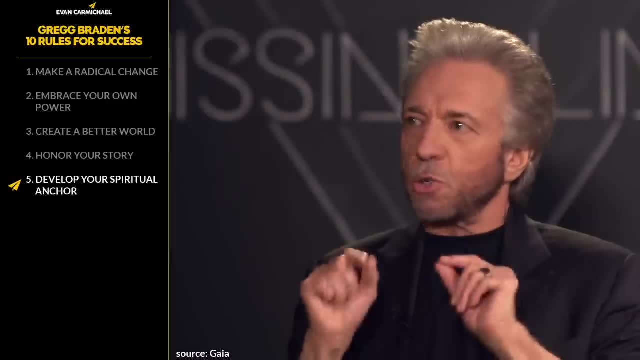 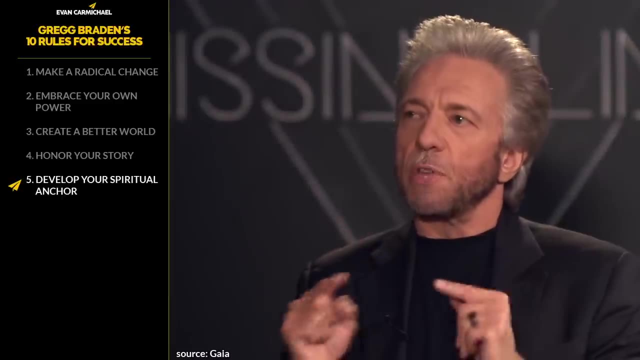 Once you know that, we then can live our truth in a world, whether other people support it or not. When we depend on other people for that support, that's where we give our power away and that's where many of us come from. 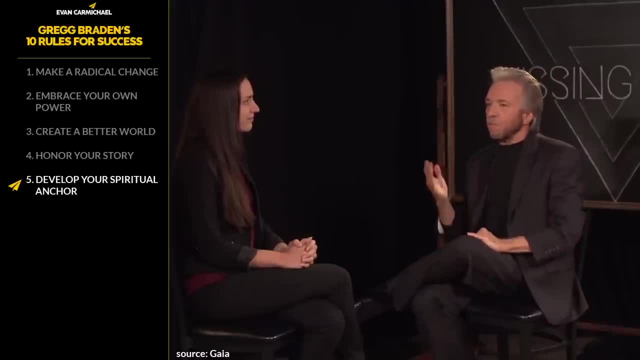 I'll just say to the young people listening: I come from a very difficult family background: dysfunctional, alcoholic family, full of criticism instilling self-doubt. I've been in the business for a long time. I've been in the business for a long time. 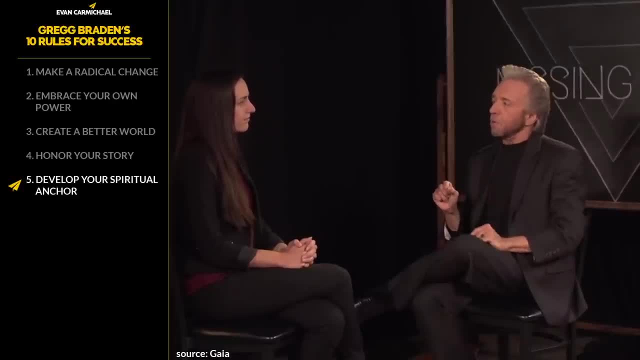 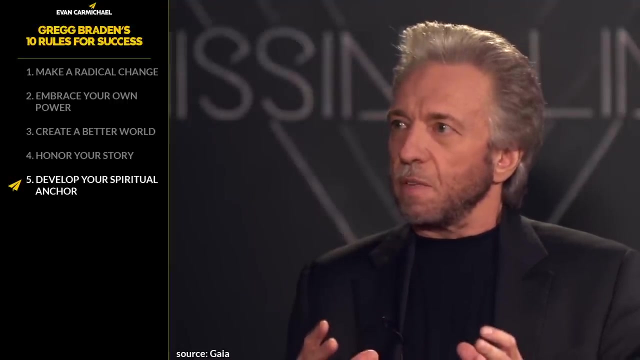 I've been in the business for a long time. That's very different from what I had out in the young people. I have a younger brother. We came from the same family and we had the same criticisms. I didn't believe what my father told me about my inability in life. 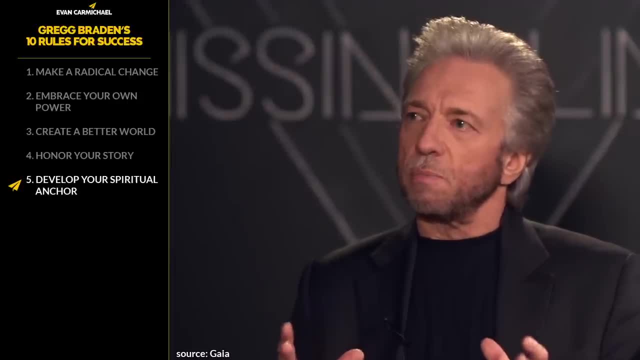 My younger brother. he did believe it, He embraced much of it. It's so interesting: two different people, the same family, same background, interpreting the information differently. I attribute— my ability to let that criticism roll off of me and the blessing I had very early on. 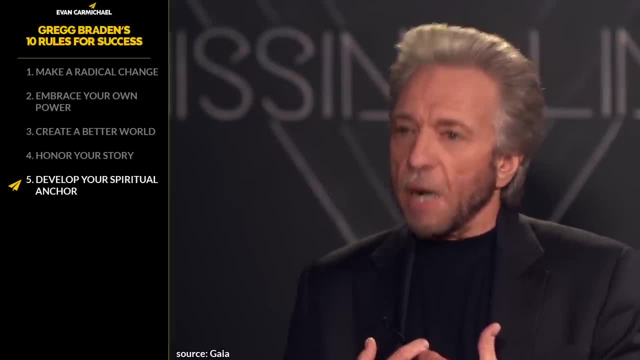 I knew who I was and I understood my place in this world at an early age. Not everyone has that, but I began looking at an early age. You know it takes a lot of work to explore the potential within every one of us. 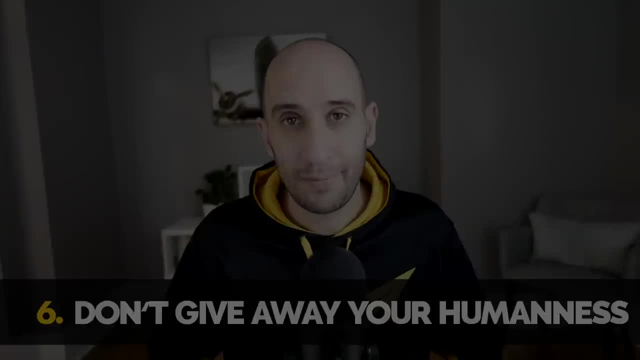 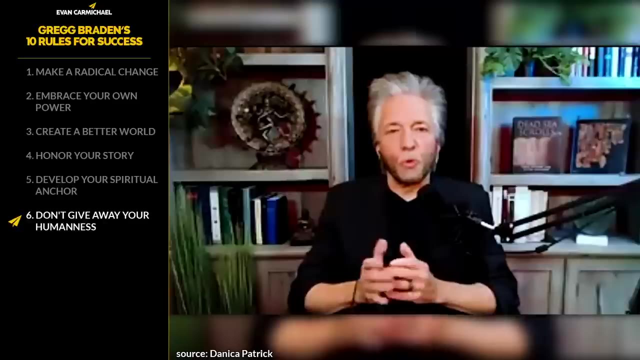 Rule number six: don't give away your humanness. We are holistic beings living in a holistic universe. part of all that is, and that is, the fallacy for the way that we try to approach so many of our problems, the fallacy that we are somehow separate from one another. 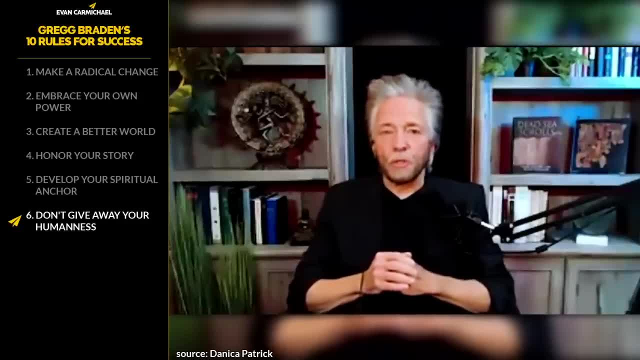 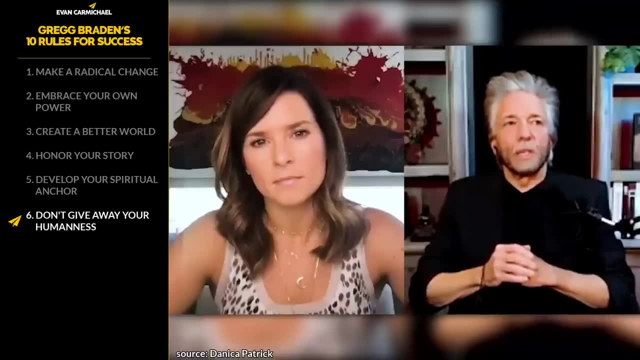 separate from our world and powerless victims of our environment, And I think one of the things that's happening right now, Danica, the, if you know, if you're gonna have a global pandemic, it's good to have it in the age of the internet. 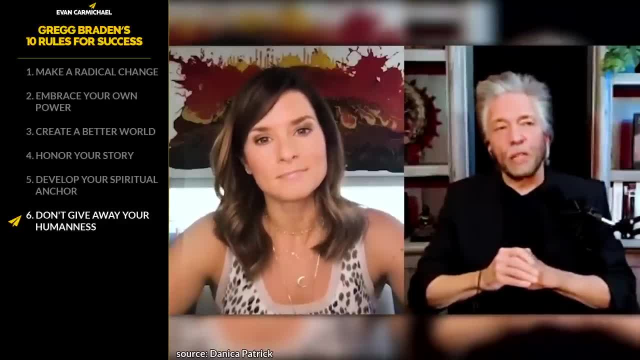 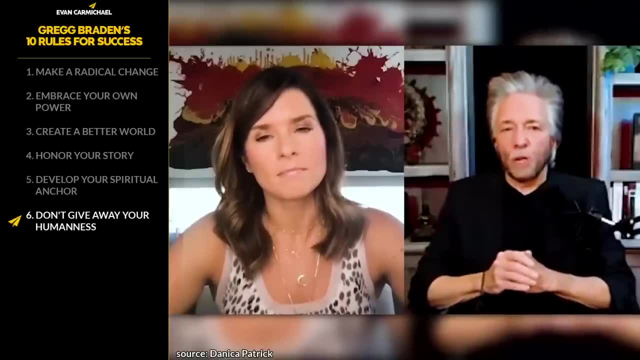 because the internet has allowed us to stay connected and it's allowed us to access information in ways that we never have in the past, And part of that access, I think, is the answer to the question that you just asked. So I'm gonna begin the answer by simply saying. 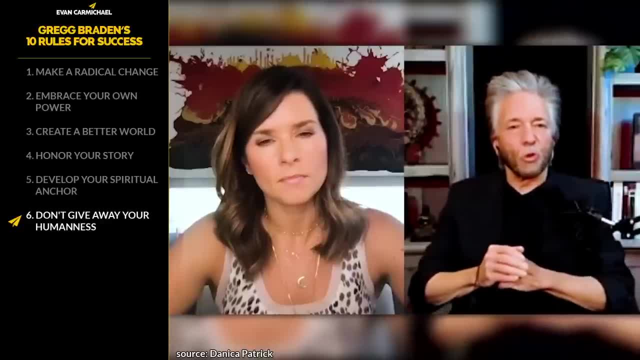 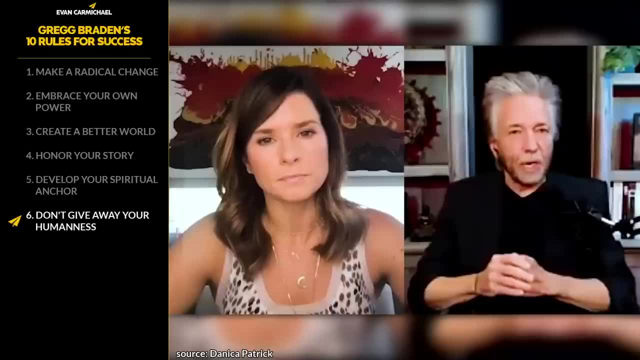 there's a battle that is unfolding in our world right now on multiple levels, right in front of our eyes. We all know there's a battle for our thoughts. That's a battle. It's very obvious. the media is battling to inform and guide the way that we think about ourselves. 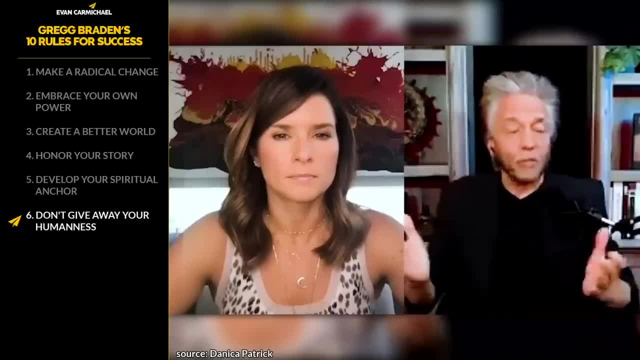 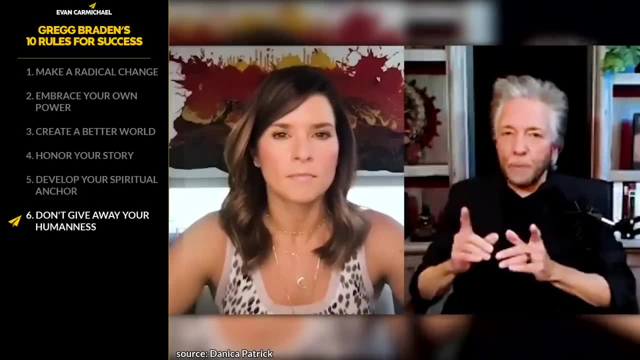 and our relationship to the world and how we respond to the pandemic and the economy and race and all the other things that are up for us right now. There's that battle, But that battle is based upon a battle for our beliefs And that battle is playing out in academia. 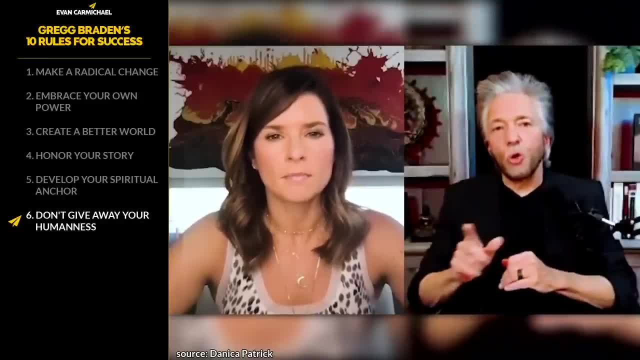 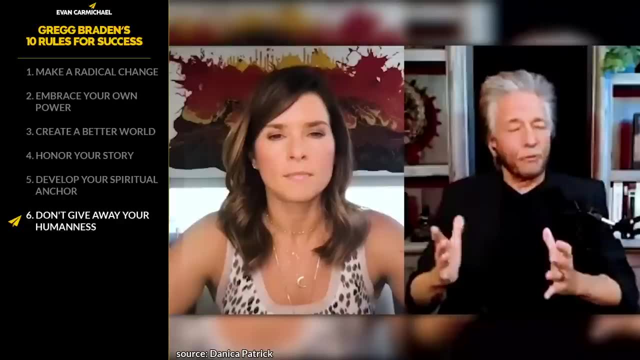 It's playing out with what we teach our kids about who they are and the way that they solve the problems of the world that come to them from from the time that they're very young: The battle for our beliefs. Where did we come from? 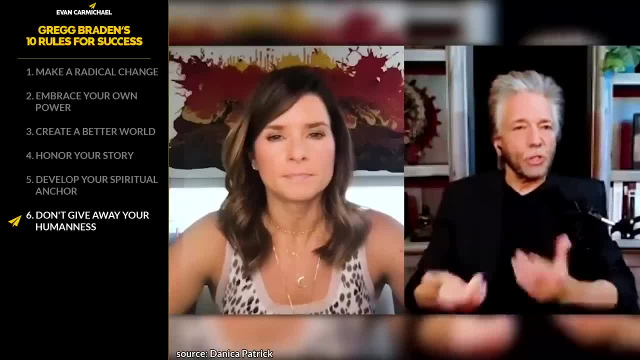 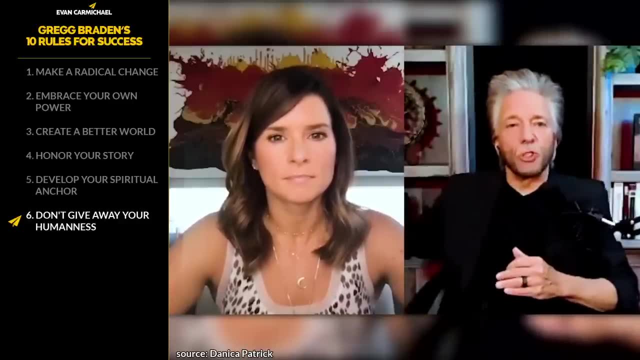 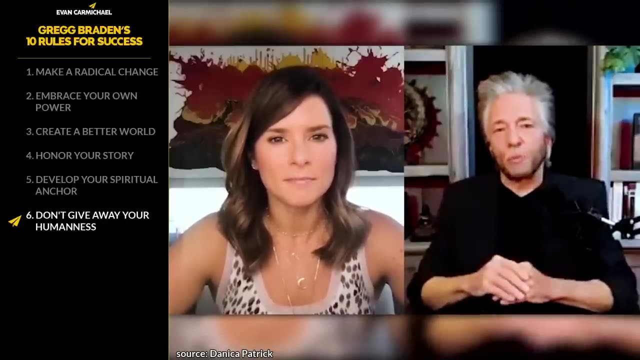 Are we an accident of lucky biology Or is there some intentionality underlying our existence? I mean, that's a huge question. Is the universe dead and unconscious and inert, Or is the universe alive and intelligent and connected? That battle is playing out. 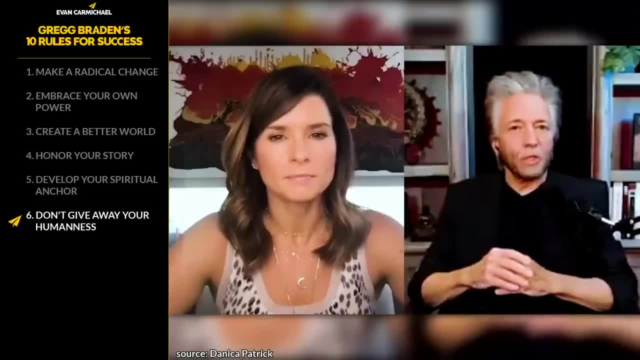 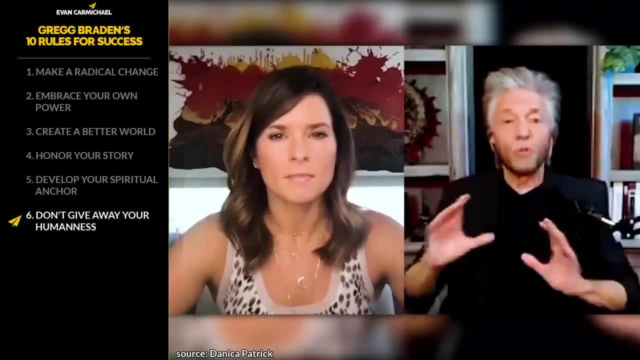 There's a battle for our bodies, And I think we're all getting that. What does it take to get healthy? What's it take to stay healthy? What do we have to give our babies within moments of when they emerge from the womb? 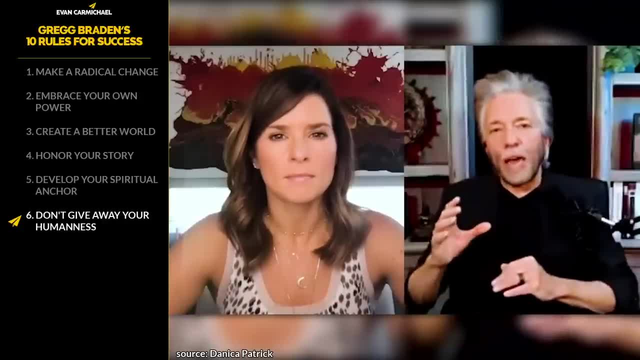 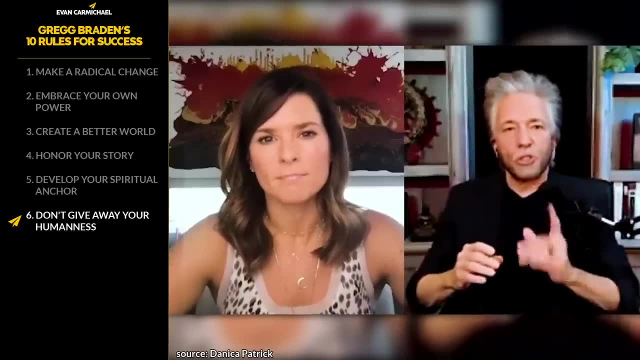 when they come into this world, we are conditioned to think that they have to have something outside of themselves in order to survive. All those battles are playing out, but I want to tell you they're all static, They're noise And they're covering what I believe. 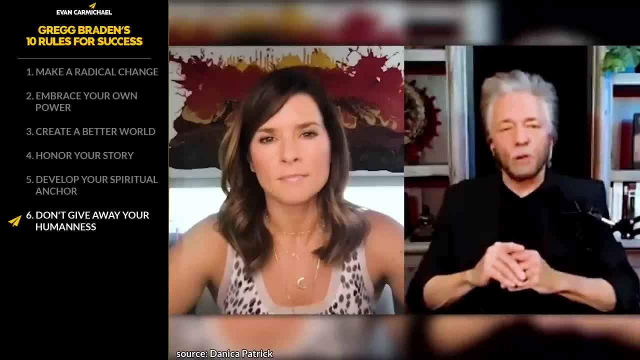 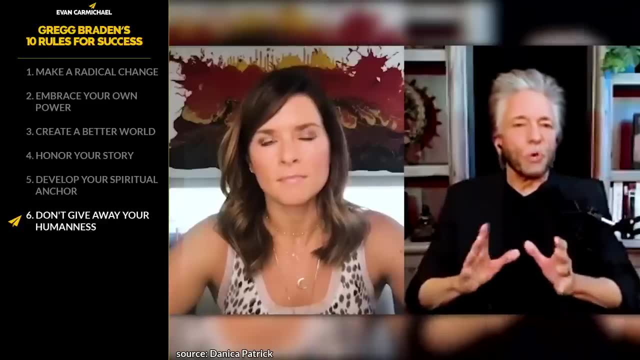 is the deepest battle of our time, Danica. it's a battle for our very humanness. Our very humanness is on the line right now Because, for the first time in recorded human history, we have the technology that can steal our humanness from us. 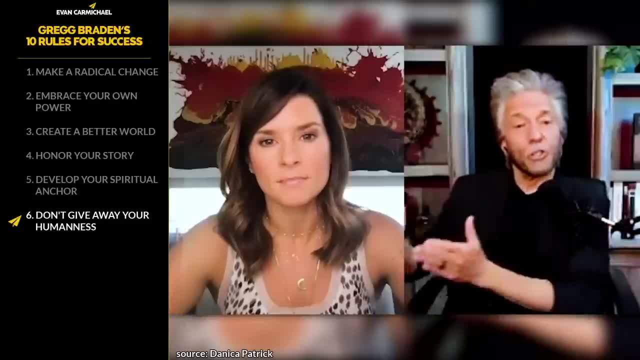 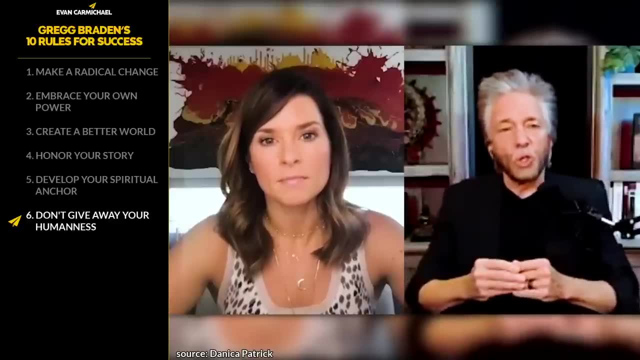 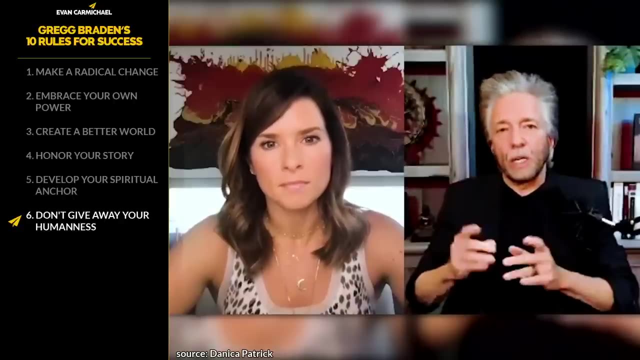 in ways that some people aren't even aware of and other societies and cultures are adopting very, very quickly. And I'm talking about computer chips implanted into the human brain and chemicals injected into the body and wires under the skin. And the problem, the problem with this technology. 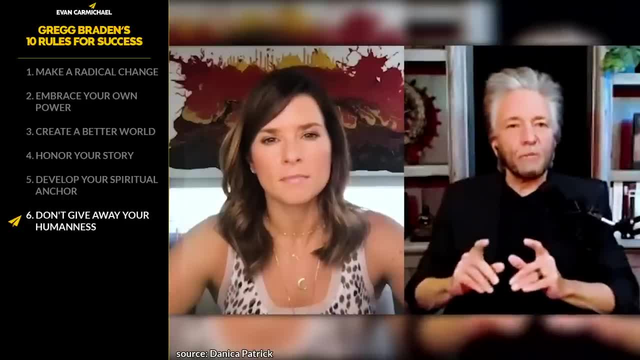 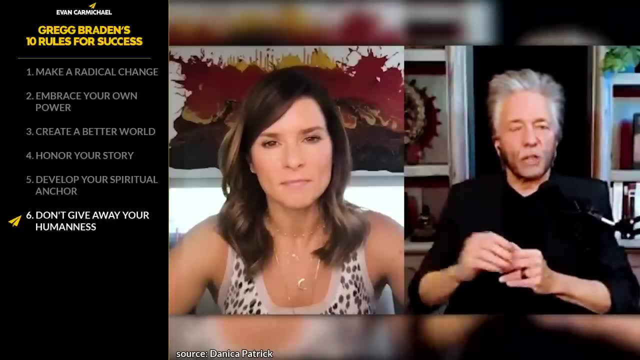 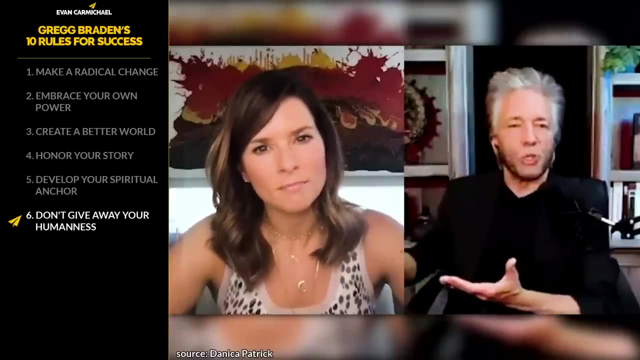 that's moving so fast. the problem with this technology that's moving so fast is that when we give our natural humanness away, when we give away our biological potential to technology, our body begins to atrophy with respect to those potentials. So if we're implanting chips in our brain, our neurons, 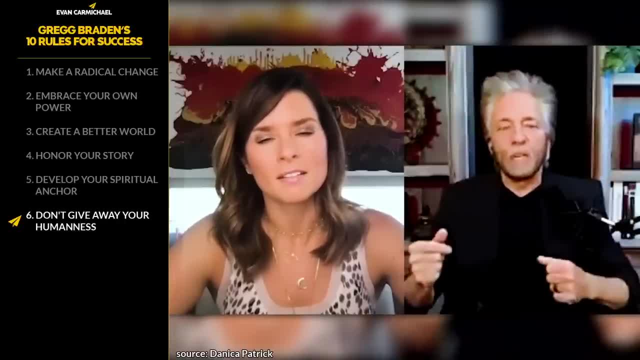 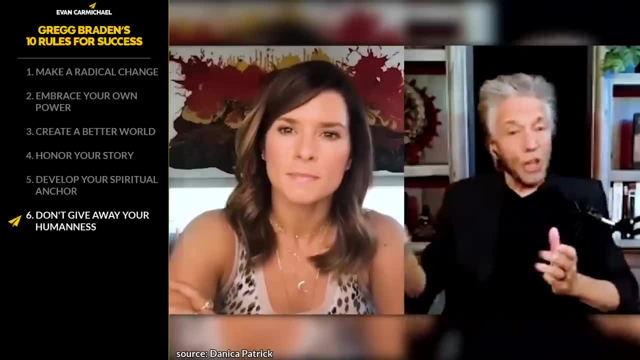 we've all heard this before use it or lose it. Biology: you hear this all the time. Our neurons begin to think they're not needed anymore, And so they stop producing. In one generation, the next generation, they become an appendage of something that used to be. 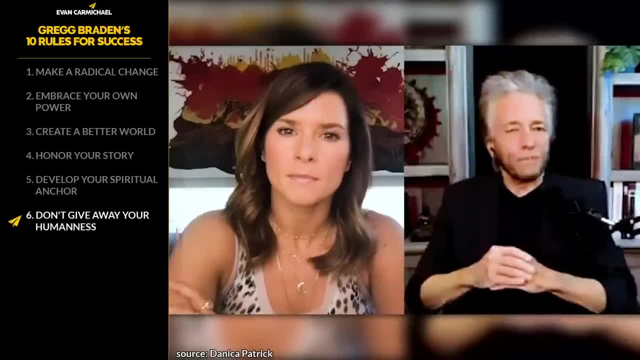 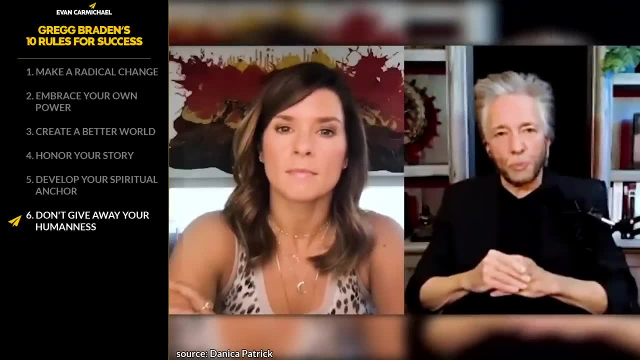 and we're not using them anymore. And for the first time in 5,000 years of recorded human history, the technology has the power to forever change our species. And the question- and I'm laying the foundation to answer the question that you asked- 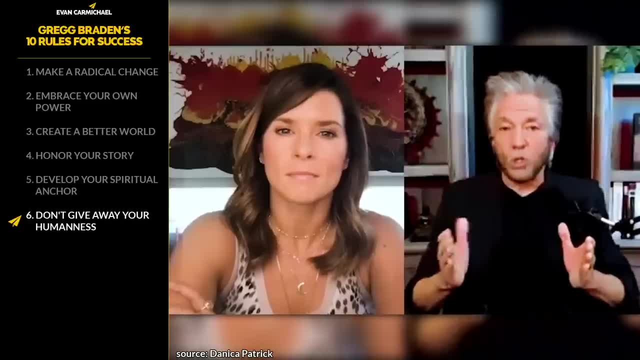 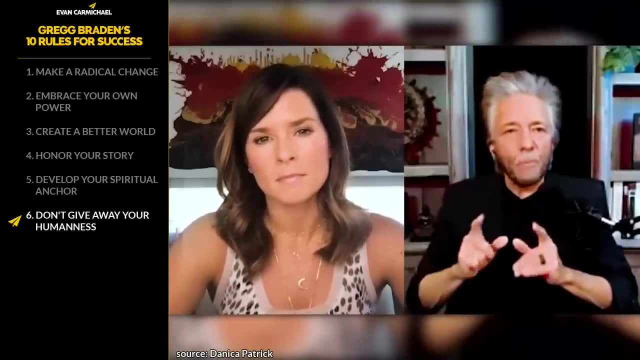 the question is- and I would never tell anyone or try to convince or persuade anyone to or not to use the technology. but here's the key. The key is: how much of ourselves do we want to give away to the technology and lose forever? 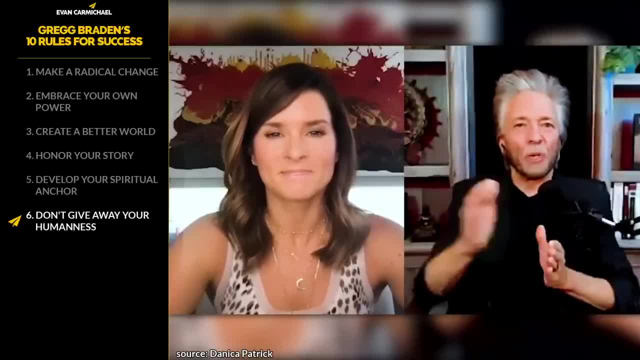 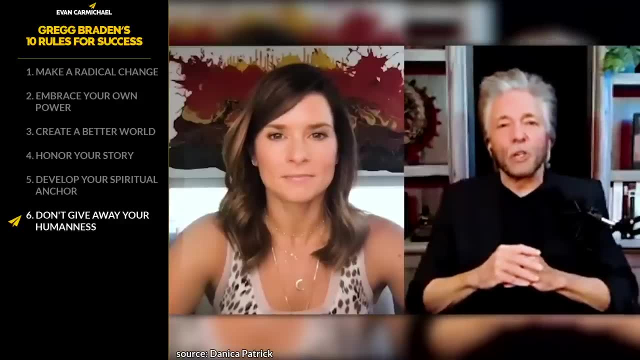 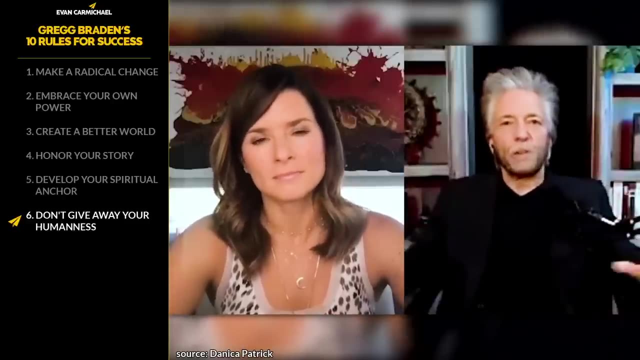 We can't answer that until we know who we are. And that brings us back to the very first question that you asked, And I gotta tell you it's where the scientific discoveries are coming so fast and furious in these obscure technical journals that very few people get to see. 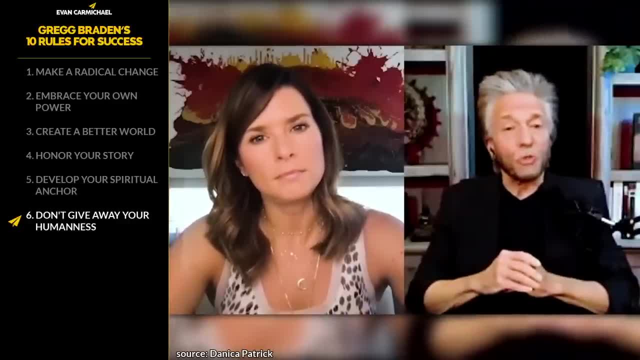 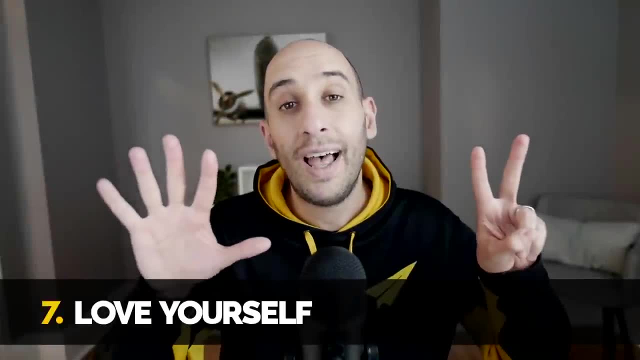 but they're based upon peer-reviewed science and they're writing a new human story, And that new human story is what the COVID pandemic is pushing us to understand. Rule number seven: love yourself. There was a very famous author and prophet in the early in the 20th century. 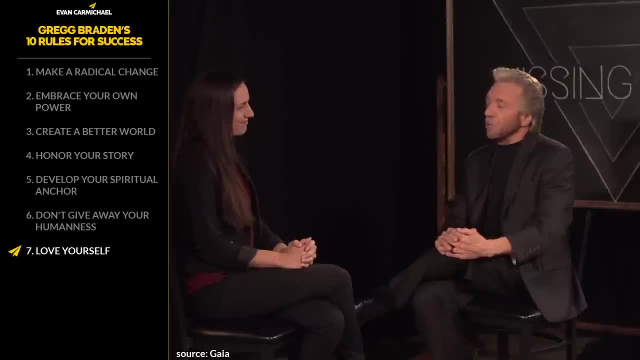 his name is Kahlil Gibran, And I began reading Kahlil Gibran when I was eight years old. and Kahlil Gibran, there is one sentence that has been my soul compass. It has been with me. I think of it every day. 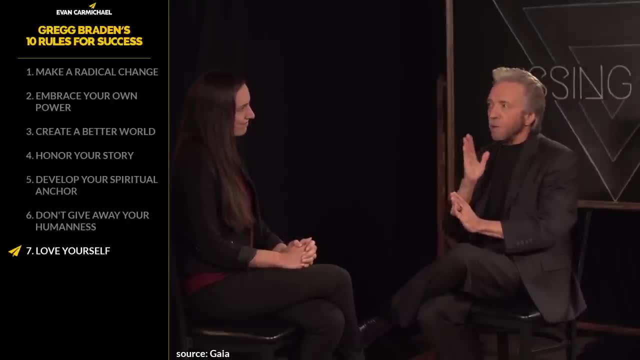 I apply it in every situation, every relationship, every job, every commitment. What he said is work is love made visible. It takes a lot of work to know who we are in this world and to demonstrate for ourselves our potential. That is our love made visible. 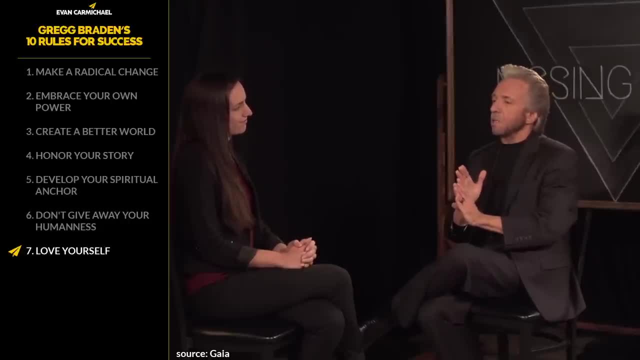 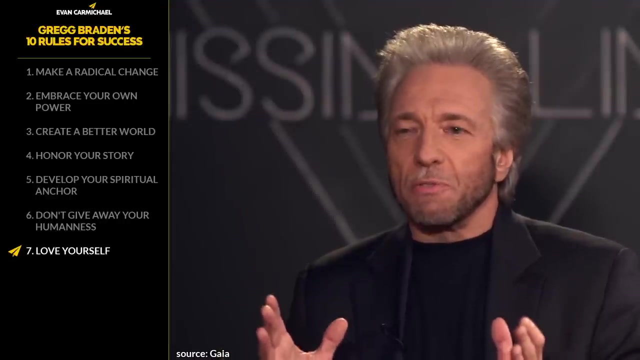 That is us loving ourselves in a way that empowers us to be in this world in a healthy, a healthy way where we thrive in the presence of all of the changes. So my invitation for any young people is: love yourself and your love made visible. 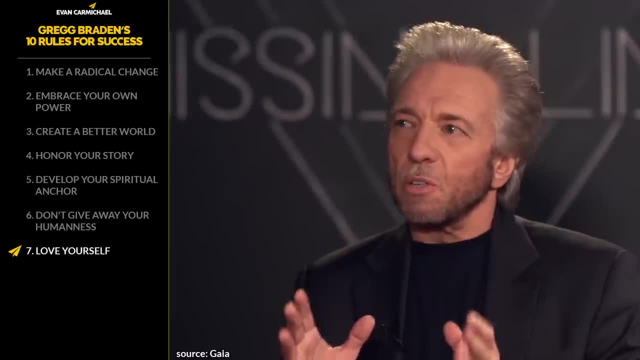 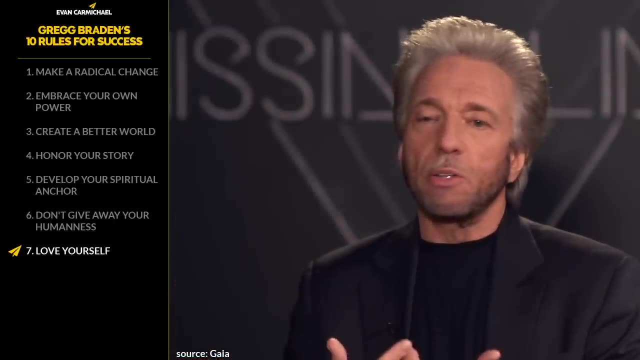 is you taking the time to understand your potential and who you really are? The good news is we have that information now. new discoveries, new science, indigenous wisdom married together. I think we owe it to ourselves to bring it all to bear on our lives today. 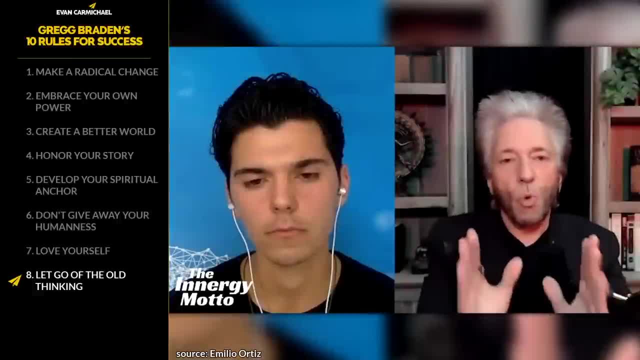 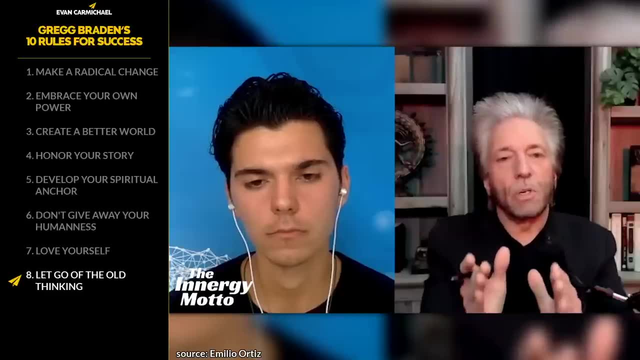 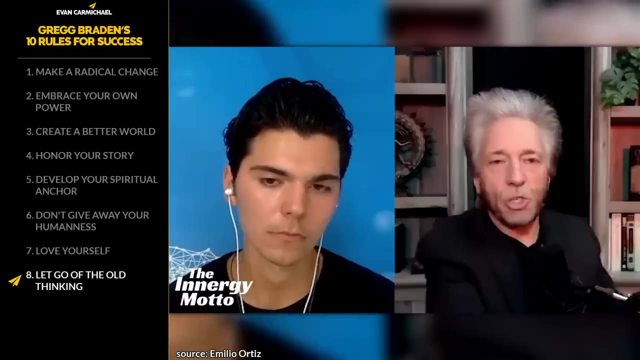 Rule number eight: let go of the old thinking. When the world begins to change, there's a fear, And in that fear, people, communities, people, people societies, governments, nations will try to cling to an image and an idea. 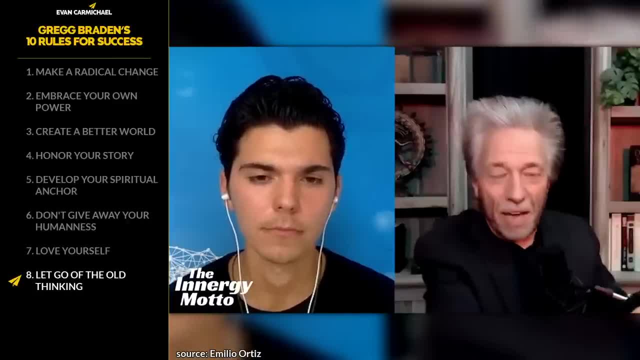 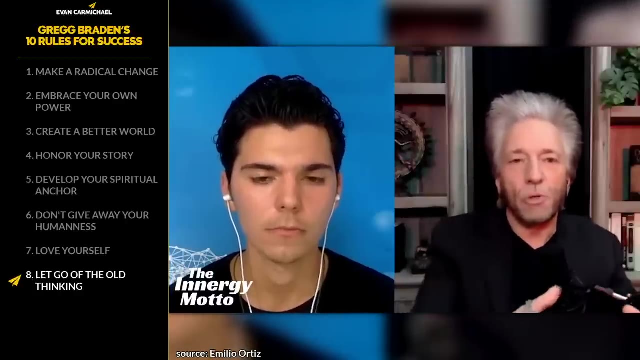 of the familiar world of the past. We can't go back to that world because it doesn't exist. That world is gone. And this is where the suffering comes from, because we're trying to apply the way we've been taught to deal with the past. 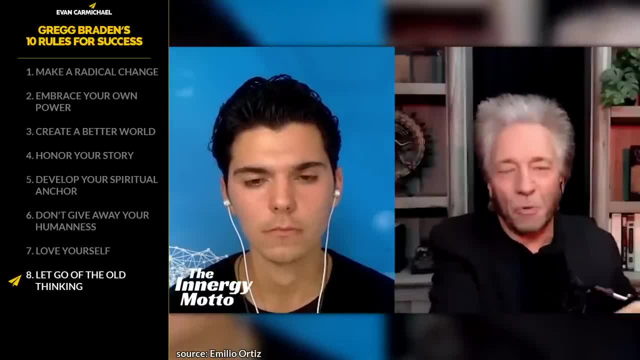 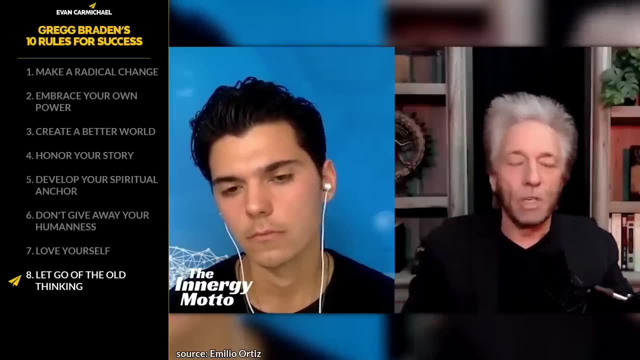 All right, we're trying to apply that in a new world, but the new world doesn't work. It doesn't work like the world of the past. So we need new ways of thinking, new ways of living, And it comes down to something very simple: two things. 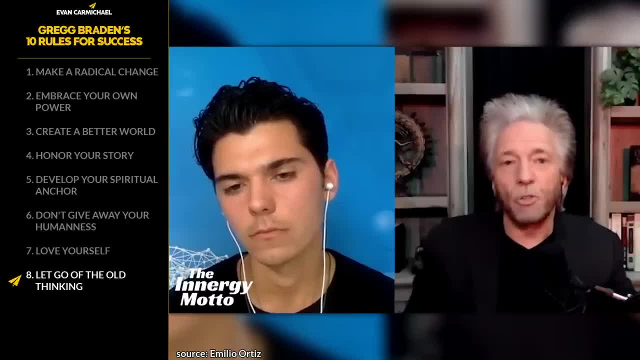 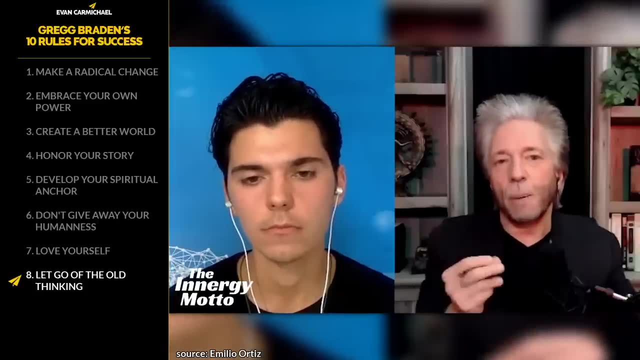 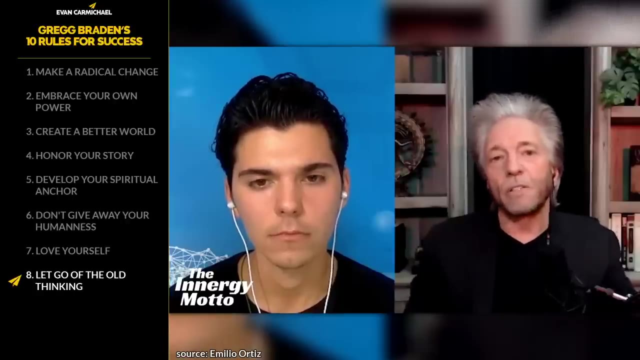 The most simple is about love, The bottom line. do we love ourselves enough to live our lives in a way that gives our bodies what they need to do, what they know how to do really well? Do we love ourselves enough to live and to think? 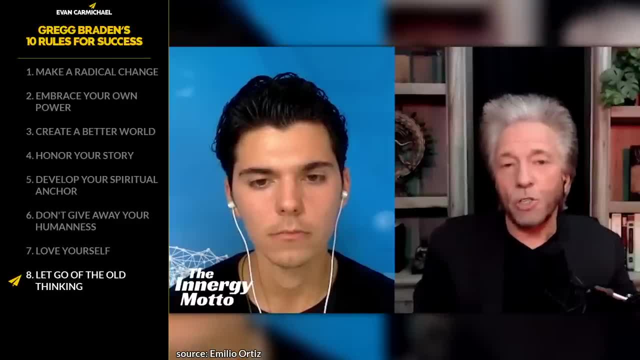 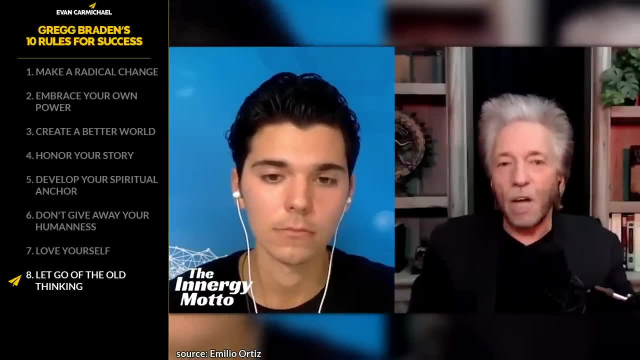 in a way that allows the best version of ourselves and the best versions of our families and communities to come forward, And the science tells us how to do that. Science is telling us what we need to do to self-regulate our immune system, And it's all the things we already know. 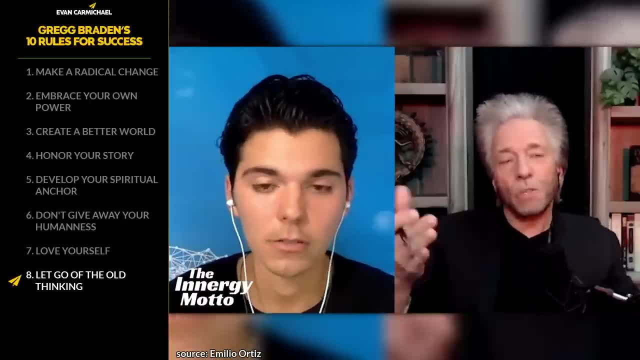 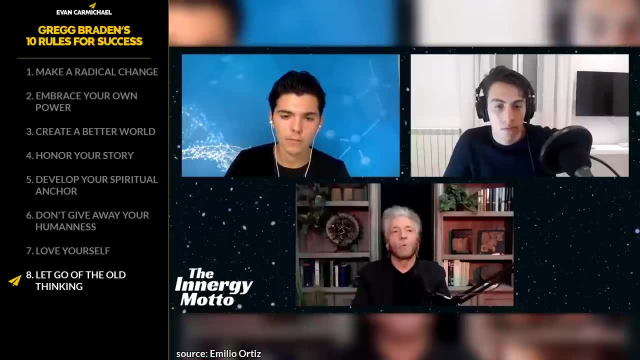 diet, exercise, nutrition. but there are new discoveries in terms of diet, new discoveries in terms of exercise and nutrition. I mean just, for example, when I was back in my 30s, 40s and 50s, back in those days. 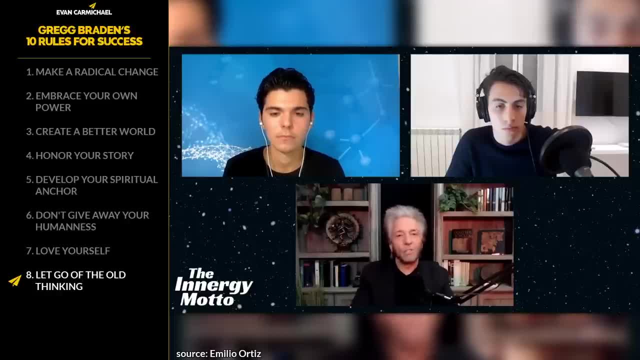 I was taught that steady state exercise was the key. So you go out and you'd run a half marathon or you'd run on the treadmill for an hour or whatever it is. Now we know that that may not be the optimum form of exercise for a lot of people. 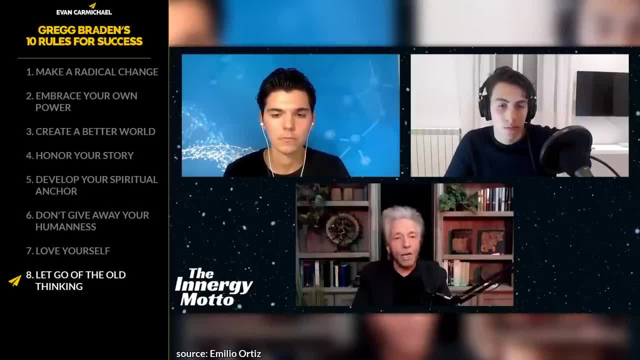 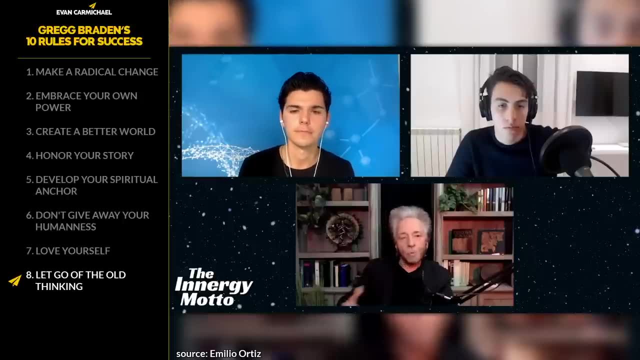 Now the human body is built for what's called HIIT- high intensity interval training. That's our biology is based upon that. When we optimize our biology, I mean that's about hormone balance. It's about testosterone in men and women. 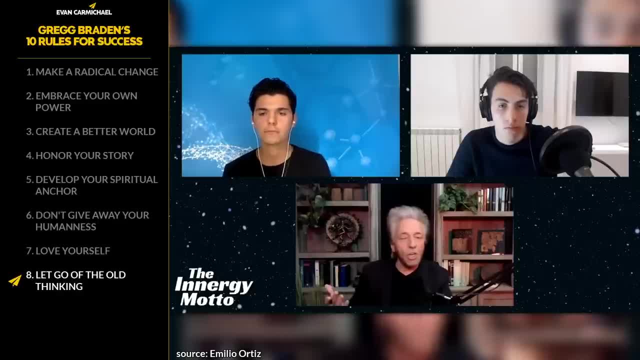 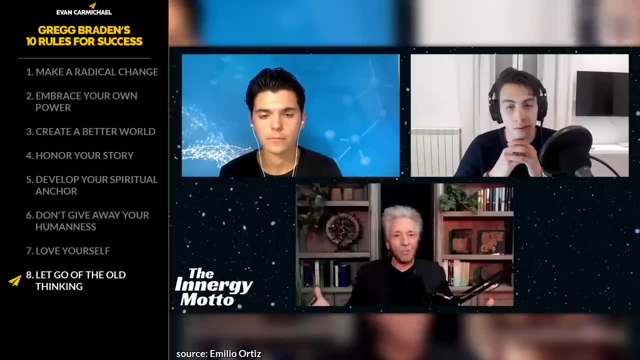 estrogen in men and women, DHEA levels and all of those things. We know that we have. a new class of stem cells has just been discovered. We used to think that people lose stem cells as they age, And we now know that you can be a hundred years old. 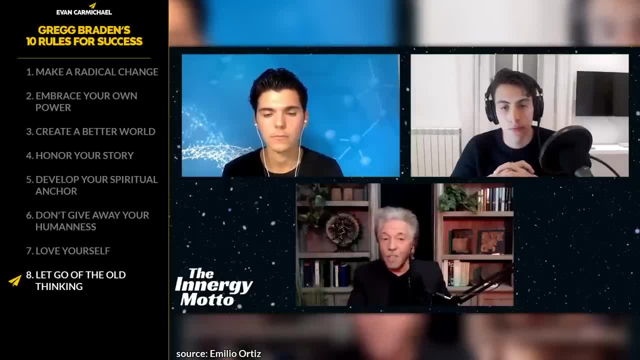 and have access to stem cells. Maybe not as easy, but they didn't disappear. It's how you get to them And that's- and nutrition and movement are keys to doing this. So do we love ourselves enough to give our bodies what they need to do, what they are made to do? 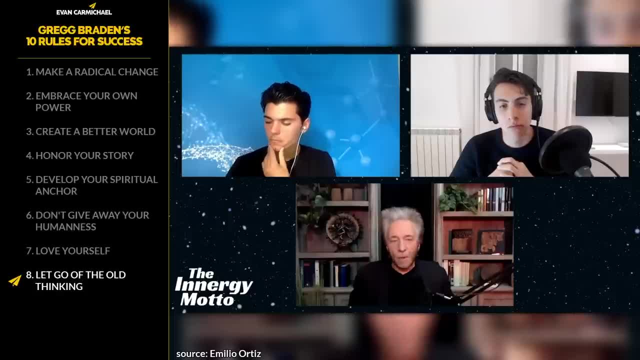 And when we begin to embrace that mastery, all of a sudden change looks a lot less scary. When we become the best versions of ourselves, we fear the outer world that change less. We fear one another less And, perhaps most importantly, we fear our own power. 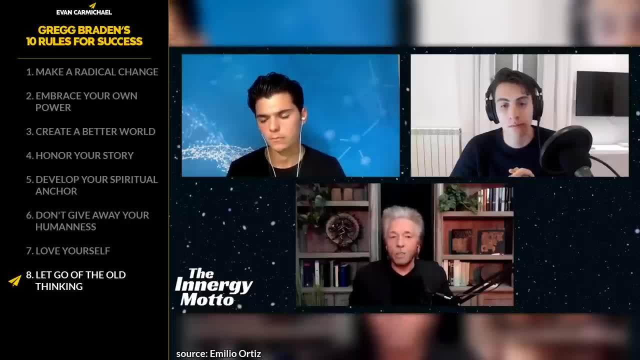 We are extraordinarily powerful beings and we're taught to discount and deny that power And in our powerlessness. this is what's happening in the world right now. There's a lot of hurt in the world for a lot of reasons. We typically are not taught how to heal that hurt. 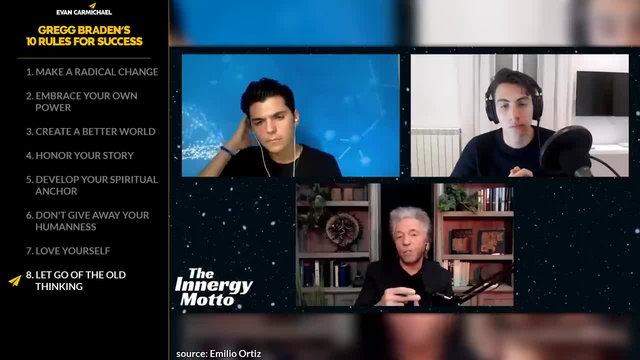 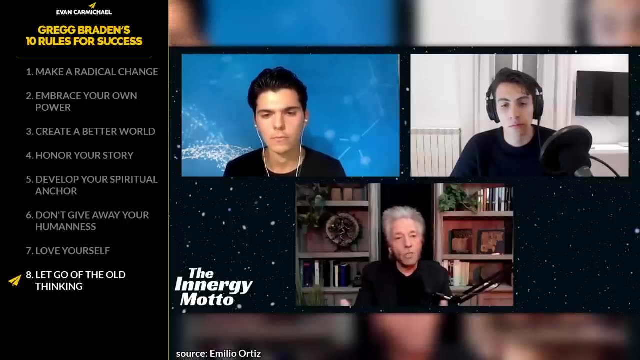 So what happens is the hurt needs to be expressed, and it's expressed as fear, And it's expressed as hate, unresolved hurt. It becomes the fear and the hate in the world, And we're seeing a world of hurt When we begin to resolve the hurt that we have within us. 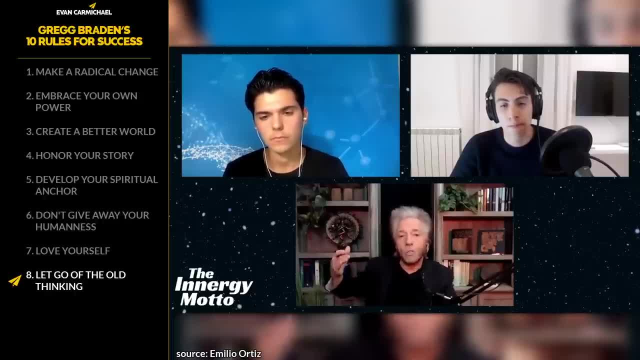 with a lot of reasons. we're all experiencing loss. We're mourning the loss of a way of life. Every one of us has lost something. We've lost freedoms, We've lost family members, We've lost jobs and careers. If you don't know how to heal that, 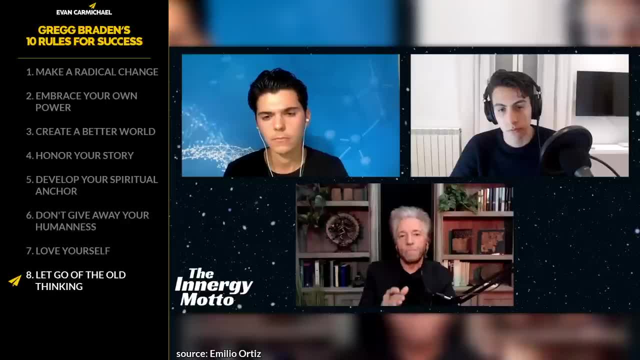 there's a lot of hurt that comes with that, And that hurt can be expressed As fear for what, the unknown, and as hate for those that represent something other than what we're familiar with. So all of this is up for us right now. 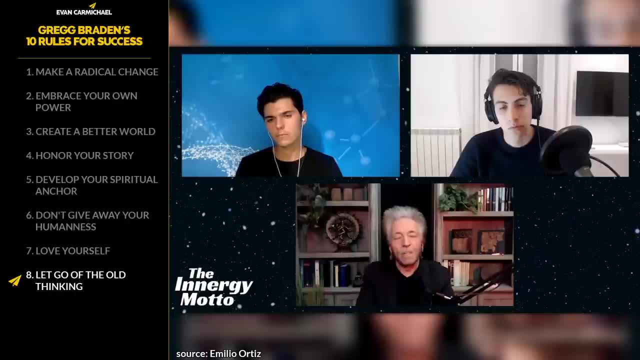 And the science is giving us the tools that allow us to transcend- not just survive, but to transcend. But to do it we've got to let go of the old ways of thinking, And I think that's probably the hardest thing Absolutely. 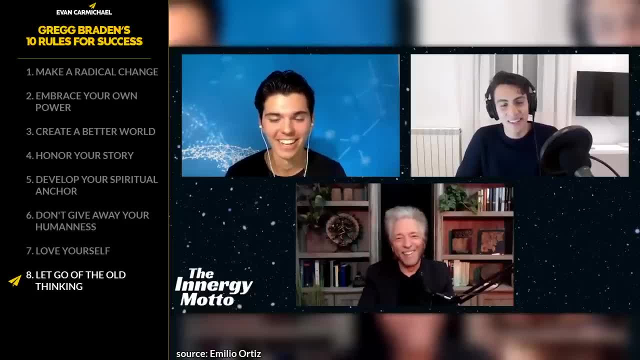 Yeah, we just covered a lot of ground there, didn't we? A lot, a lot. That was amazing. Wow, Thank you for saying all those things. Thank you so much, Greg. Sorry about that, Emilio. So well, let me ask you guys. 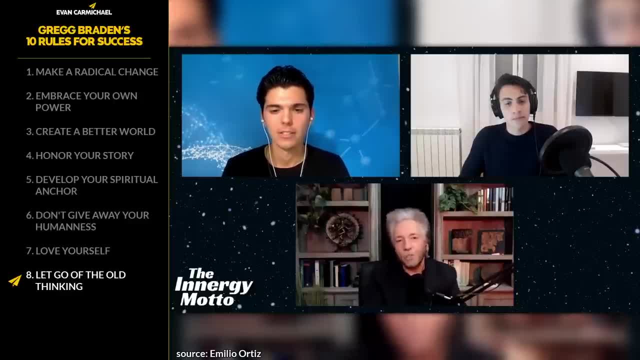 I don't know what your ages are. I'm closer to 70 than I am to 60 right now, And I think you all probably represent a very different generation. How old do I look? Let's say I shaved yesterday To me. you guys look ageless. 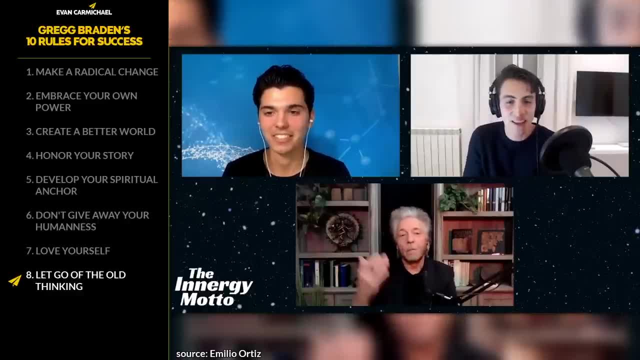 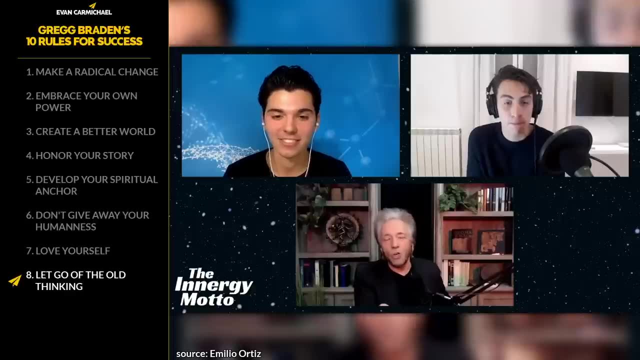 You're my brothers. You look ageless. I don't even think about age when I see you, But I know that we're probably talking about different generations. So let me ask you: We're Gen Z, It's your program, But I'm just going to ask you: how does your community 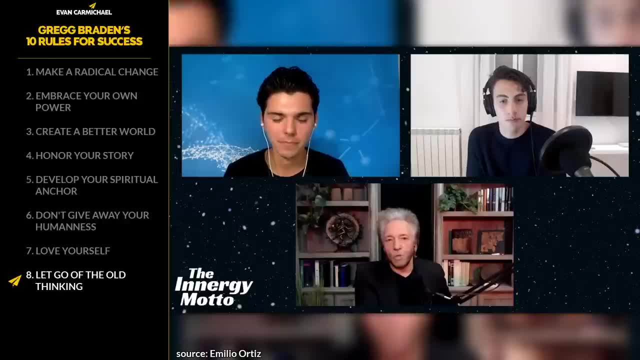 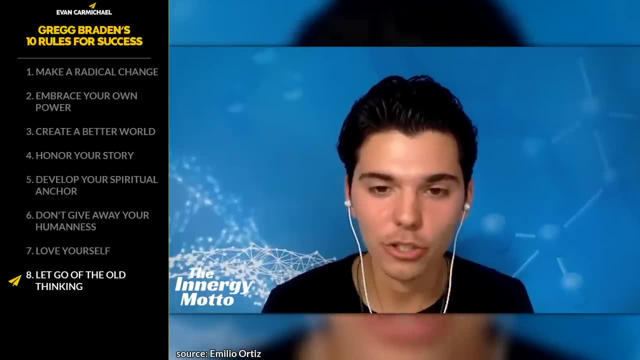 see the people that you associate with in your community. How do they feel about what's happening in the world? I think it's a lot of mixed emotions. I mean, as you said, there's a convergence of cycles, So there's the cycle of the climate. 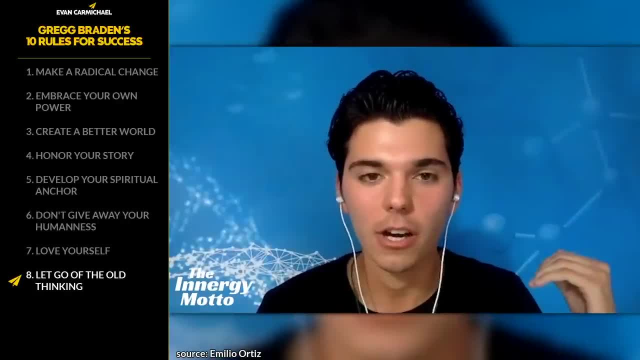 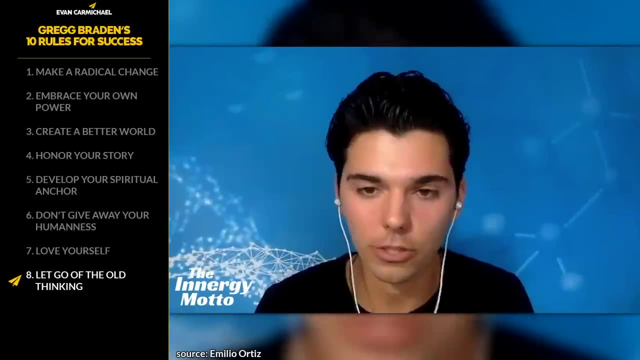 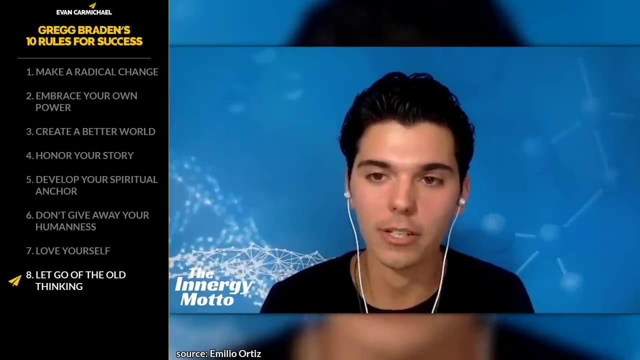 For that and that area, I think our generation is extremely moving forward. A lot of their purpose, a lot of their conscious and energies is towards helping that. There's also the cycle of innovative technologies, as you said right, And that's a difficult one. 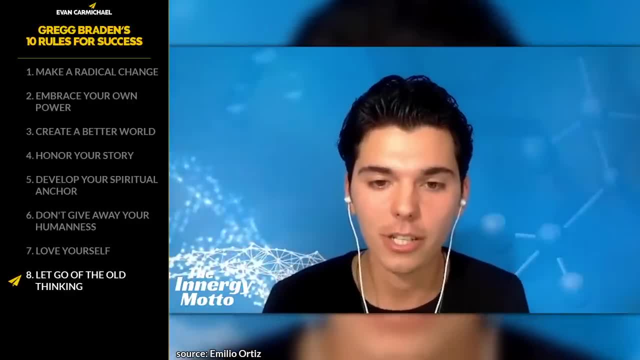 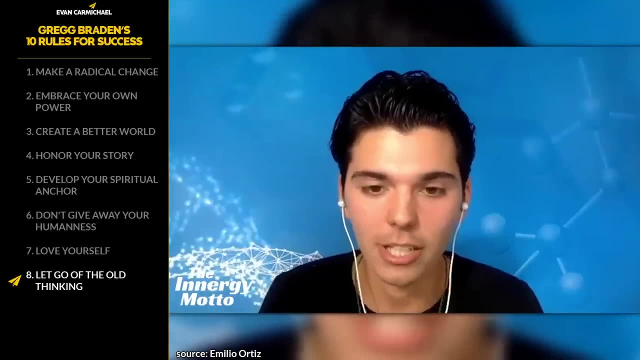 I saw one of your interviews talking about the neural link with Elon Musk. That's one of those things where it's you never know what can happen with that And it can be such a transformation in our humanity. So there's so much that I mean to answer your question. 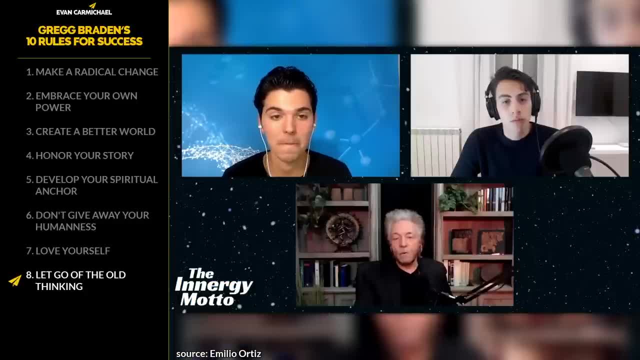 there's mixed emotions. mixed emotions, Yeah, well, you know, and this is the key. This is the key: How can we solve the problems if we're not honest with ourselves about the problems? And that, I think, is probably the biggest hurdle. 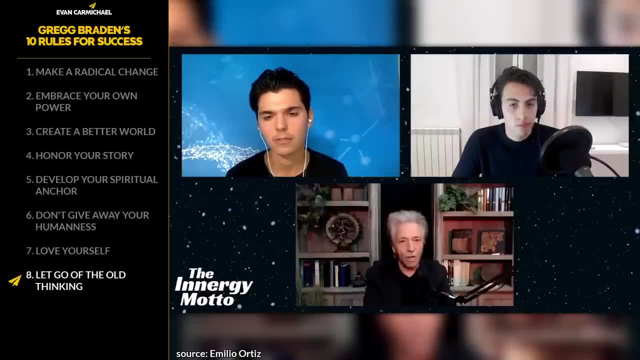 because there are so many competing agendas that are out there right now. So many competing agendas. Climate is a huge. I've been talking about climate. as a geologist, I love to talk about climate because I was studying this back in the 70s, you know, when I was in the corporations. 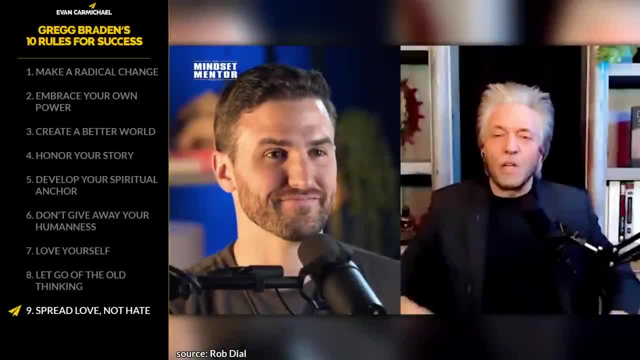 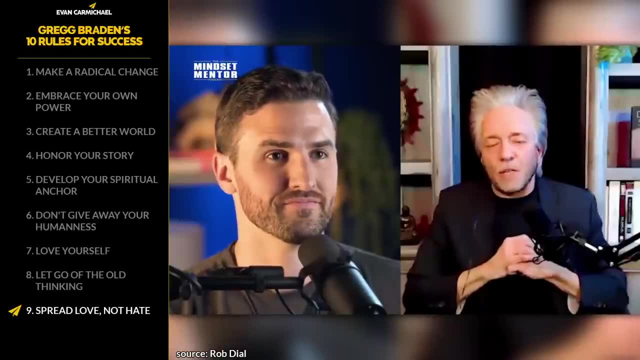 Well, number nine: spread love, not hate. The idea of love means different things to different people, And that's where the answer is: yes, You know, we do need to have that, And this is why I say, even before COVID: 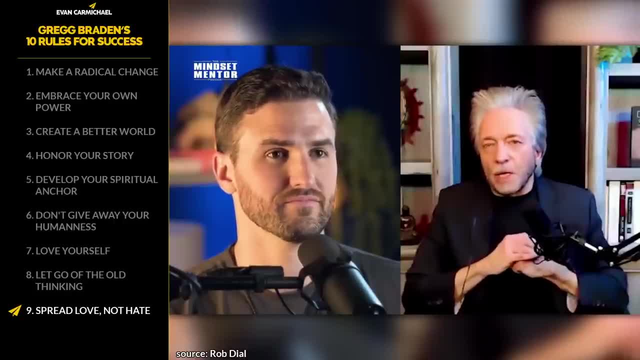 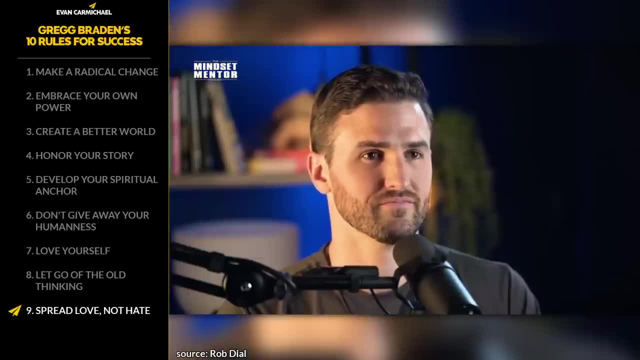 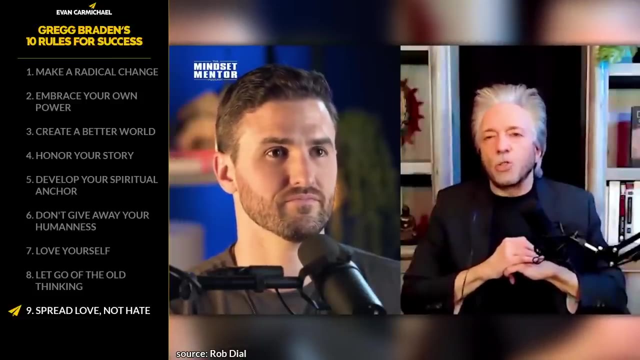 this was happening, we as a society and in some cases, as a planet, as a global society, we were already primed for the fear, Our part of a very dangerous game and an ancient trap where we are taught, And we are taught- to hate and fear the things that prevent. 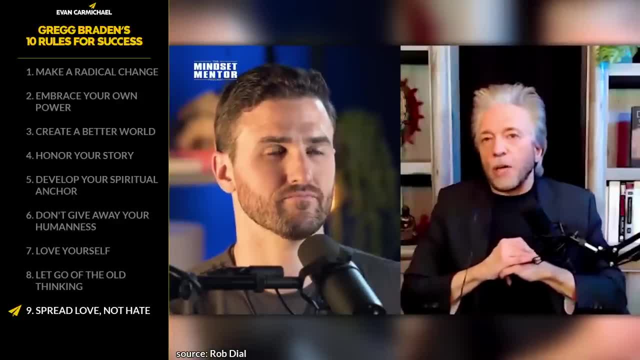 the world from moving in one direction or another. So we had the 1% and the 99% And the inequities, and that taught people to hate prosperity and wealth. And we have men against women and we've got Muslims against Christians and Jews against Muslims. 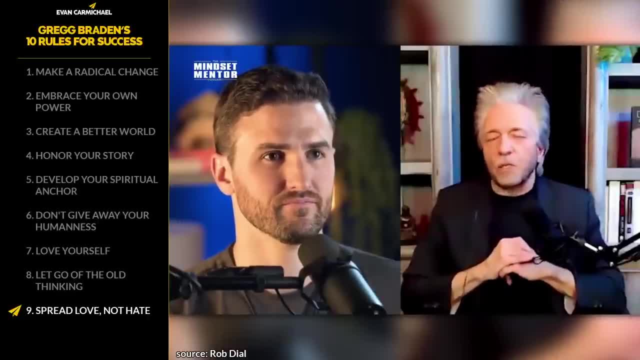 And we've got Blacks against whites and Hispanics against whites and Asians against whites. And if you look back, if you look back, if you look back, if you step back and look- it's about every six months or so you know- there's a new division. 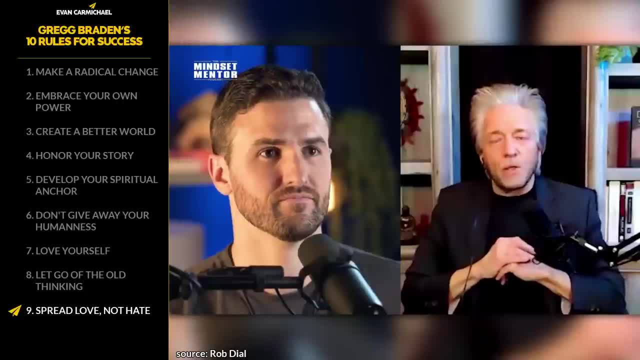 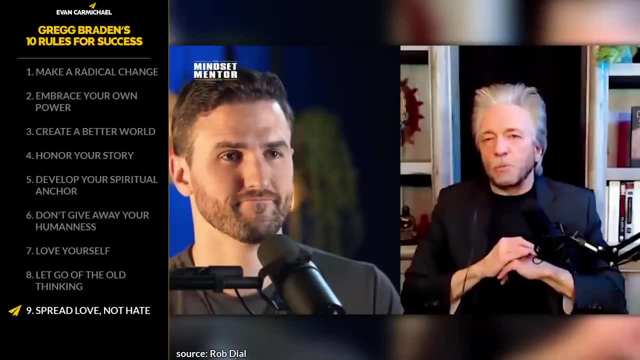 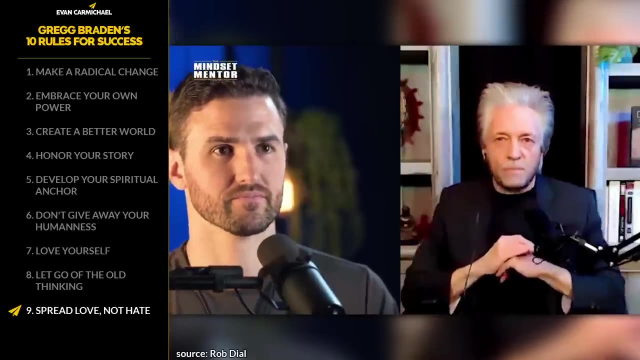 that is introduced and it's supported in the mainstream. And I'm not saying that there aren't problems. We've got a lot of problems but we've always been able to work those problems out in our societies and our communities. But when people are influenced through media- and there is a lot- 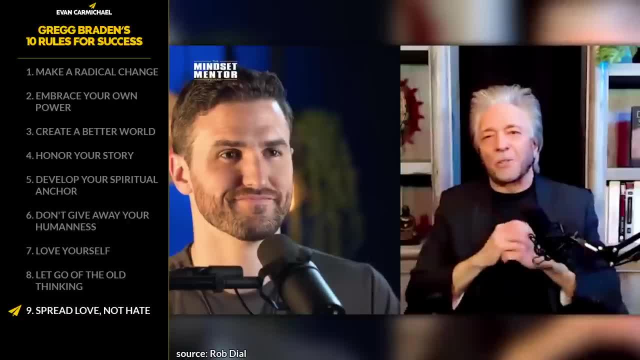 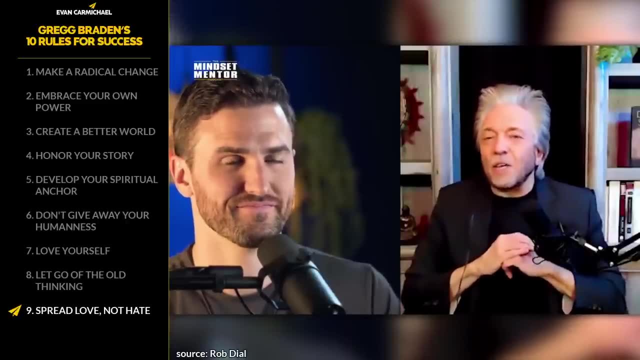 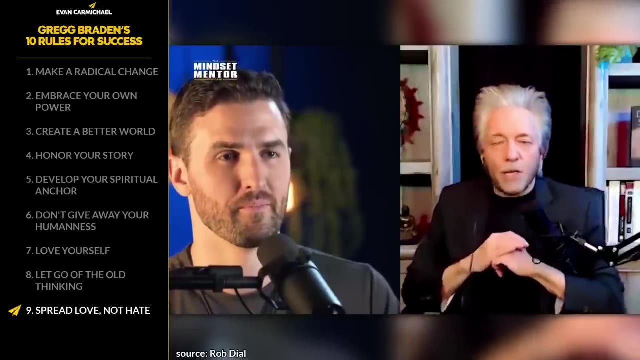 of influence. I remember when I was a kid, you know, when I went to that Jefferson Airplane concert back in the old days we had three television stations And they were actually news: ABC, CBS and NBC- And they were news stations And the broadcasters would as objectively as 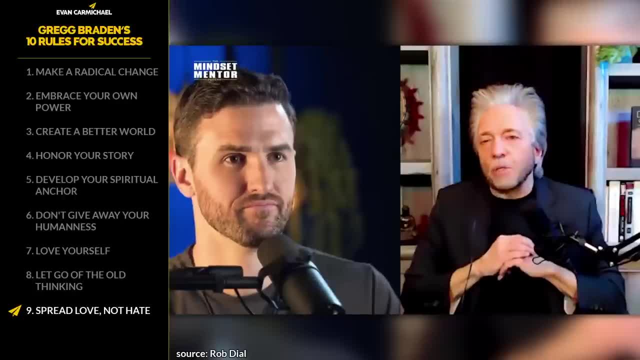 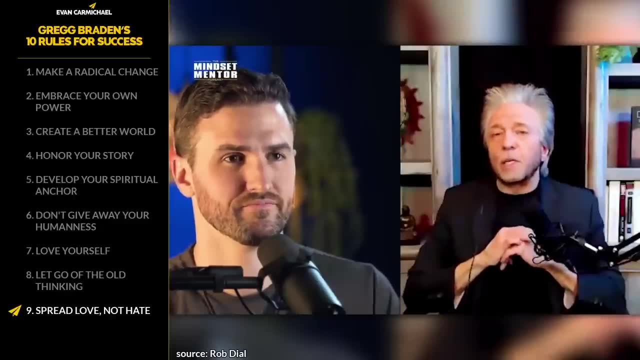 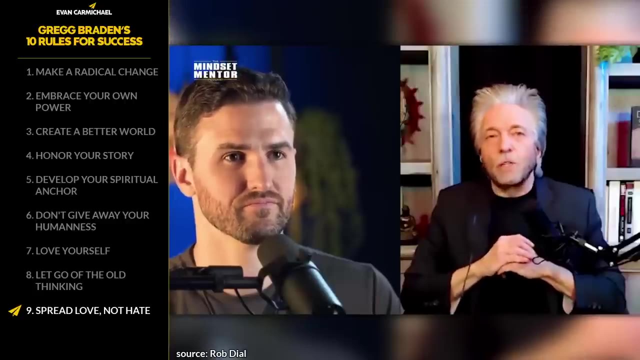 they could, they would inform us as to what had happened without showing any emotion. They tried not to. They weren't showing any favoritism in one way or another. And I remember the exception. I remember when Walter Cronkite, I was in school. I was in grade school when Walter Cronkite announced the 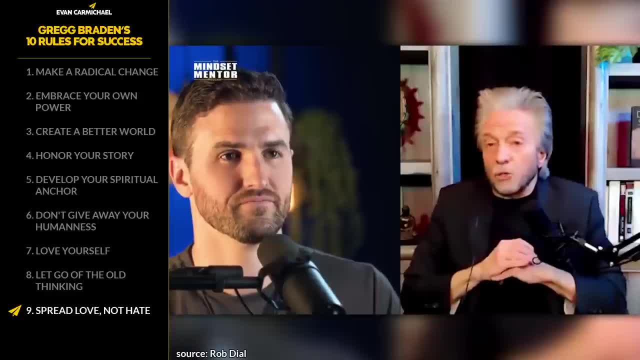 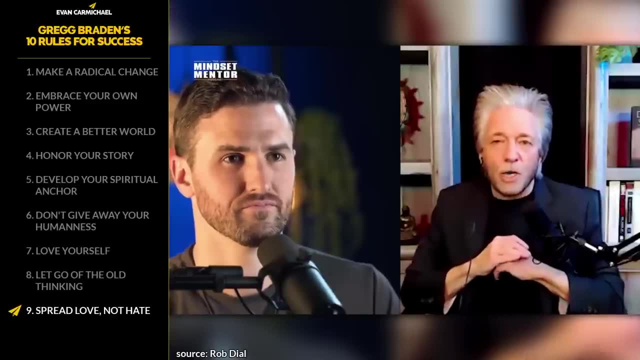 assassination of John F Kennedy And they let schools out And we all went home and watched in horror the events that were unfolding. And it's the first time I'd seen a news broadcaster cry. He cried, took off his glasses and he held his hands in his eyes and he cried. 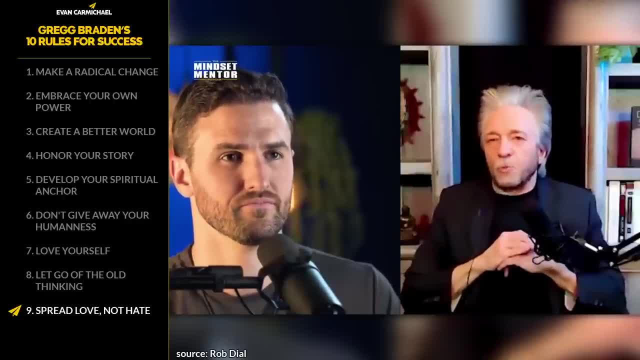 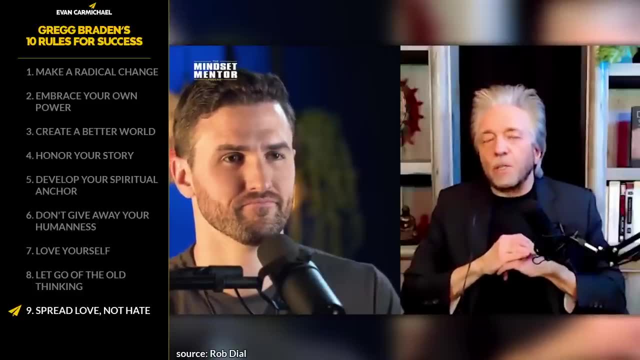 which was very atypical for a news broadcaster. We've come so far from that. We don't get news anymore. What we have are opinions, And the opinions are, for whatever reasons they are, dividing us as a nation. But it goes so deep. 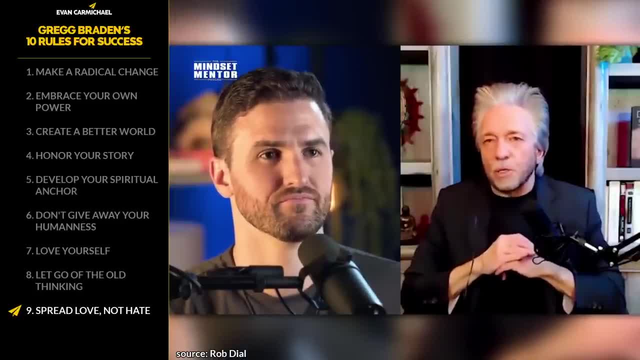 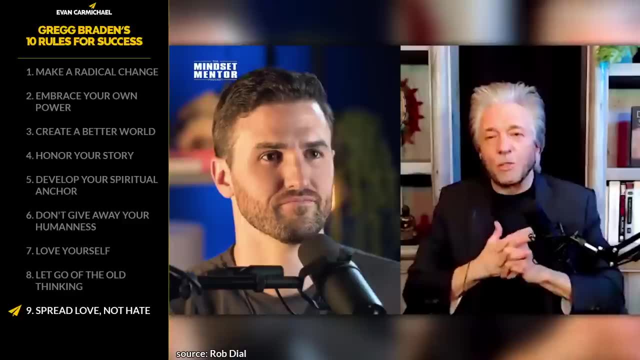 It's actually dividing us, the very fabric of our families. It's tearing our families apart. I know right now I have friends who have. I've never had any children, never been blessed with children. I think I'd be a good dad, It just never happened. 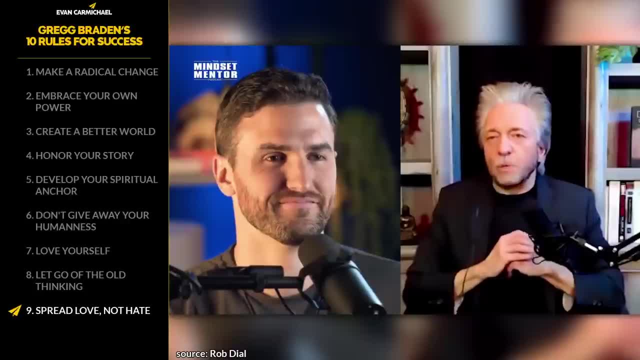 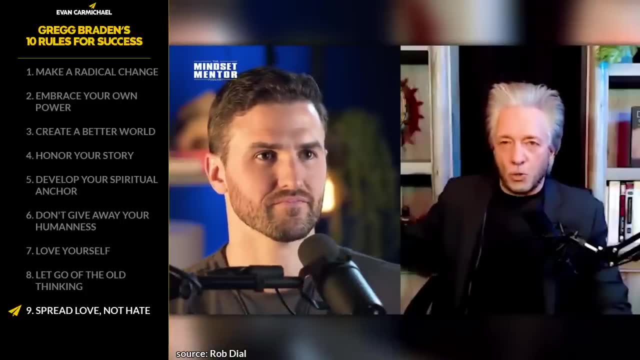 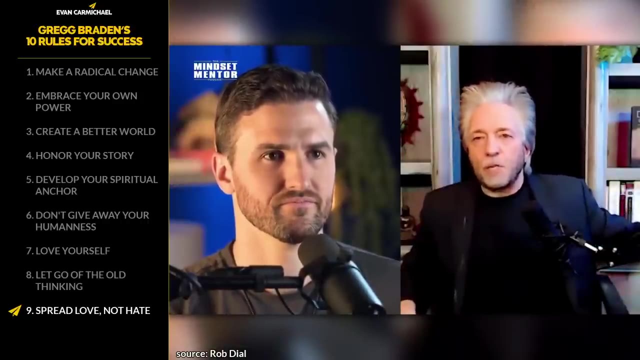 But I have friends that are- And even at the dinner table with their kids in high school and college- who get their information from one source in social media, and the parents are getting their information from another source. it's very, very different information And it clashes so much at. 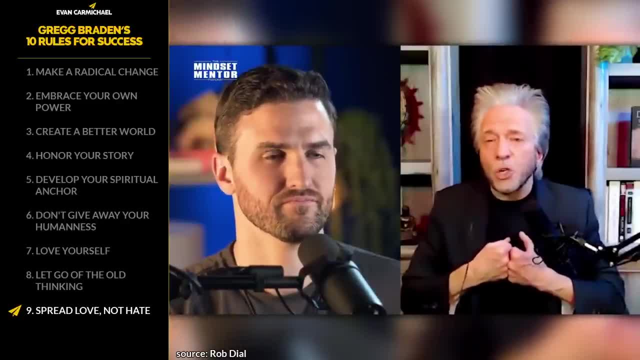 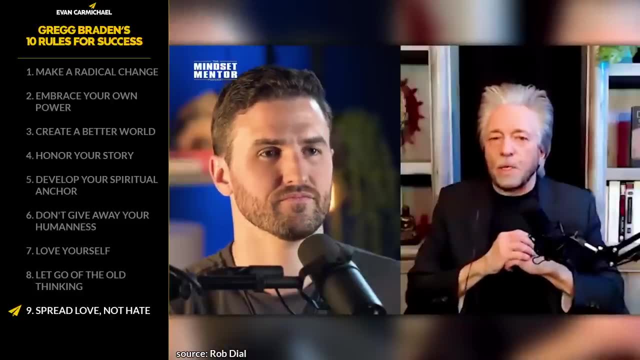 the dinner table. some of them cannot even complete the meal. There's so much hurt and so much anger And what you're saying, Rob, is historically it's a very old, old game And it's being used now because it works When you can keep people a population. 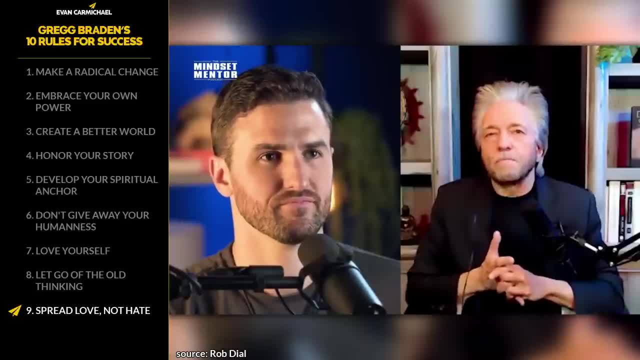 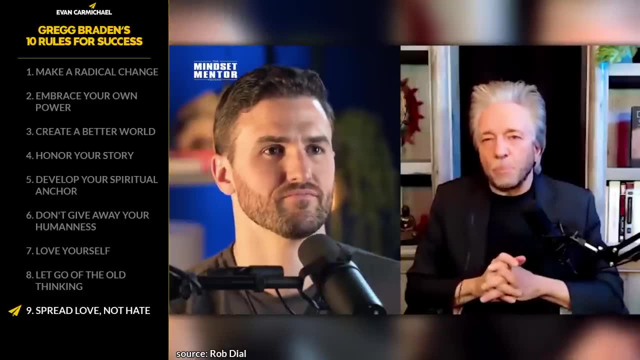 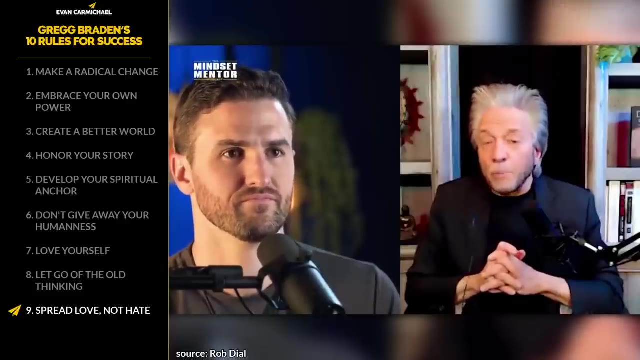 divided? there is no. it's hard to have common shared values and common shared opinions, And this is what's happening to America right now. The very fabric of America is the family. the family unit, the values, the history, culture is all under attack And as we give in to that division, what happens is our society. 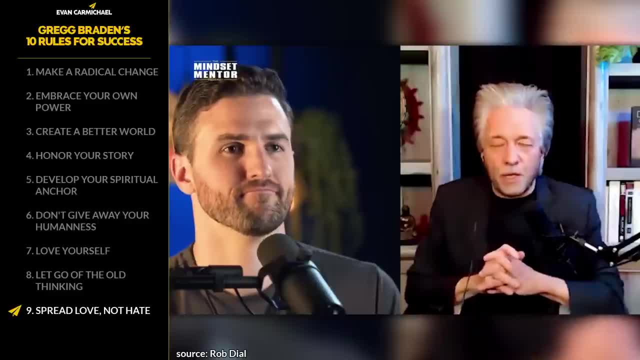 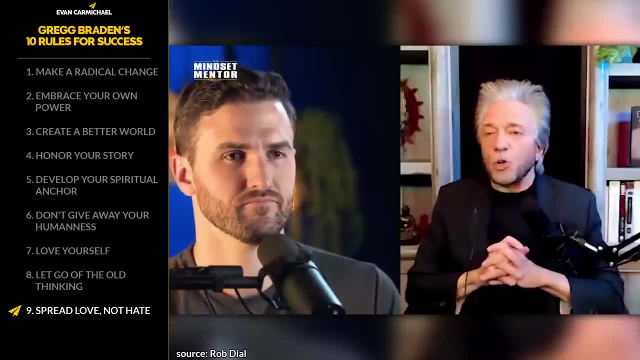 becomes ripe for a new way of thinking and a new way of living to sweep in. And it happens before you know it. So is it right, wrong, good or bad? I'm not going to say that here, I'm saying it's. 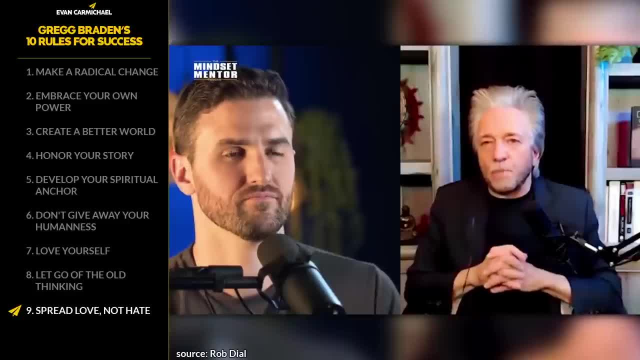 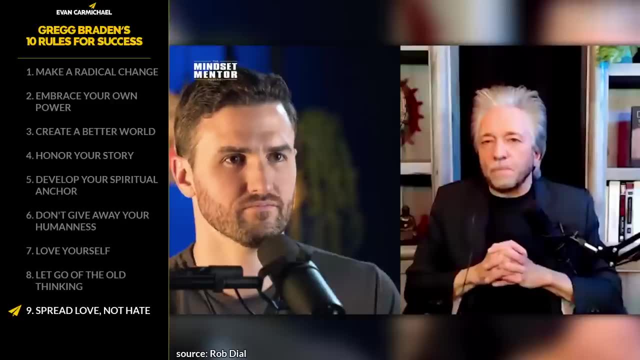 important that we be aware and not fall into the dangerous game that's dividing us from our friends, our families, our communities, our society, dividing us between nations, Because, at the end of the day, we're just people And, at the end of the day, we all want this. We've heard this. We 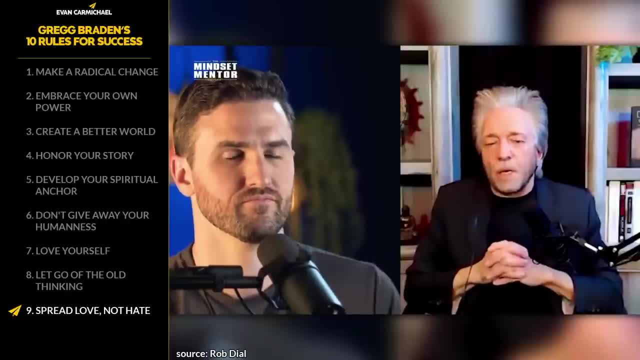 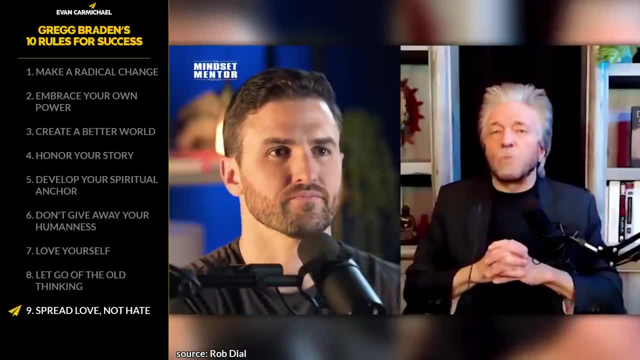 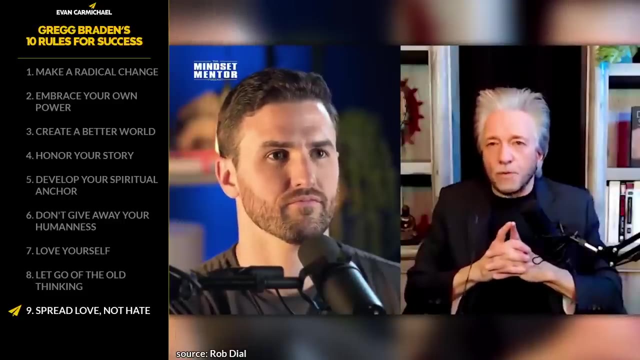 all want the same things for ourselves and for our children, And we have a pretty good idea of what that is. So it is, it's an awareness, And I think the most fundamental, the most radical act that any of us could do is to do what you've done: Turn off the external. 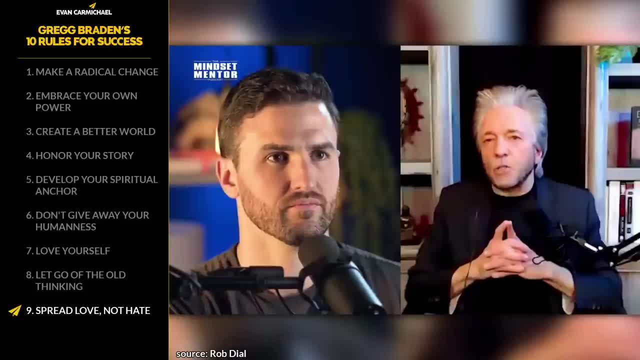 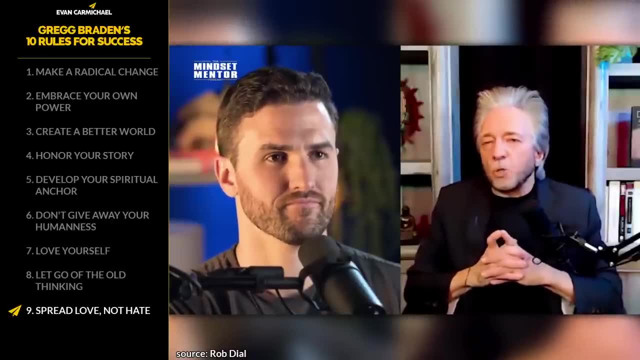 Noise That distortion And think for ourselves And you look around and ask yourself: are these things really happening? And if they are, make changes where changes need to be made, But do it from a place of kindness rather than from a place of hate. There's so much hurt in. 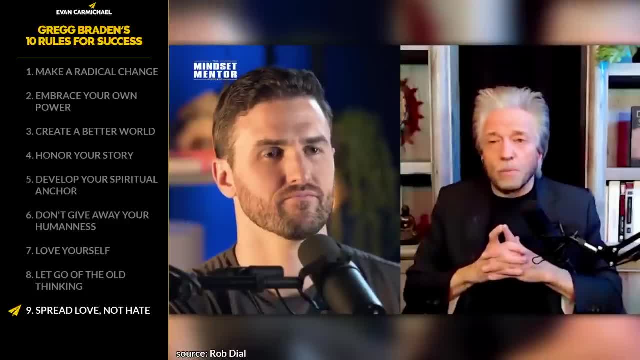 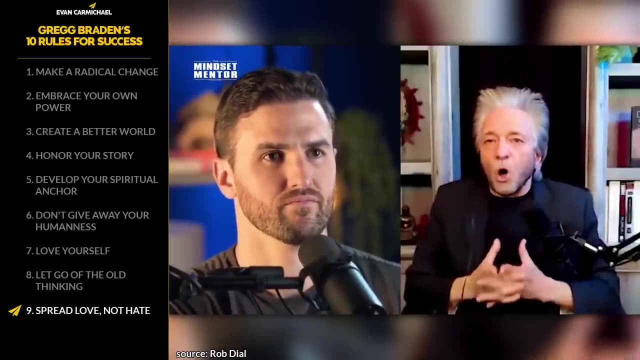 our world right now And we all are hurting And we're all mourning loss. Every person on this planet has lost something. We've either lost loved ones and friends- I lost my mom to COVID right at the end of the year- So we've all lost. And if people haven't lost loved ones or friends, we have lost a way of life. 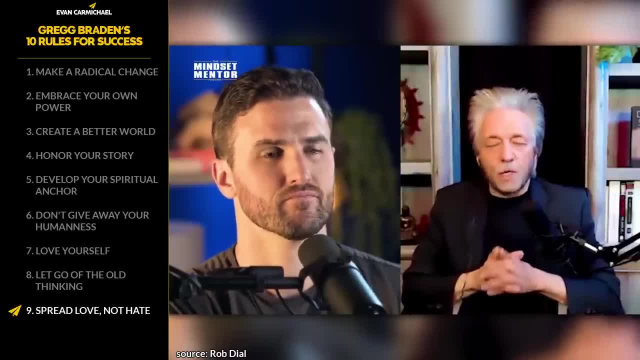 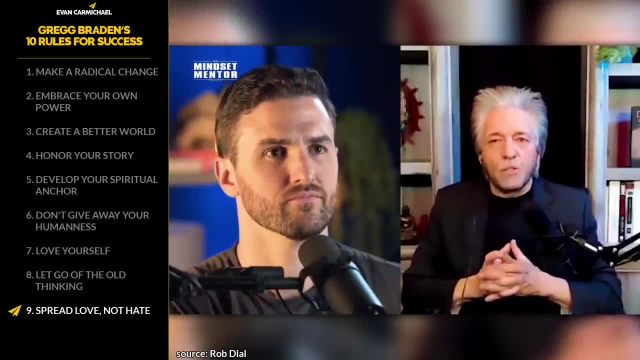 So there's something we are all in mourning, whether we recognize it or not, And if we don't have the tools to address that mourning, what happens is our deep hurt is expressed as hate, And you're seeing that hate in the world today, And so this comes back. 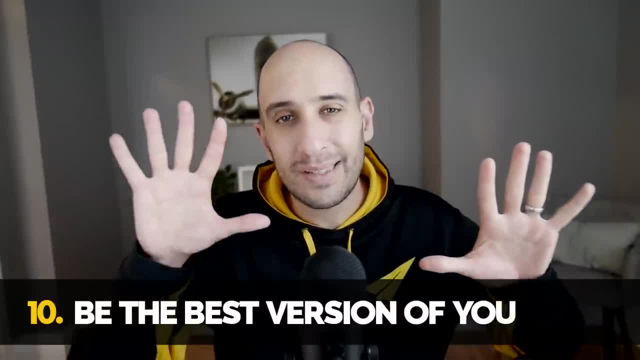 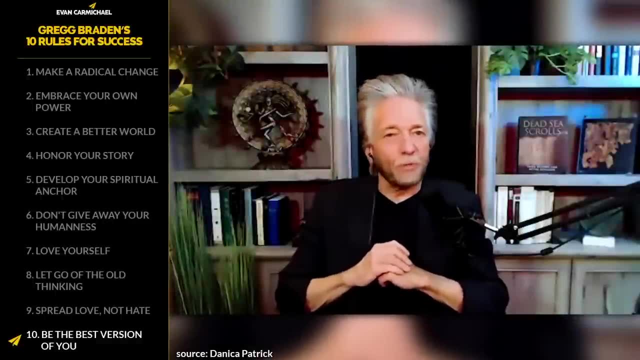 To the beginning of this conversation And rule number 10, the last one before some very special bonus clips- is be the best version of you. We covered a lot of ground And for some people they've heard it before. For some people. 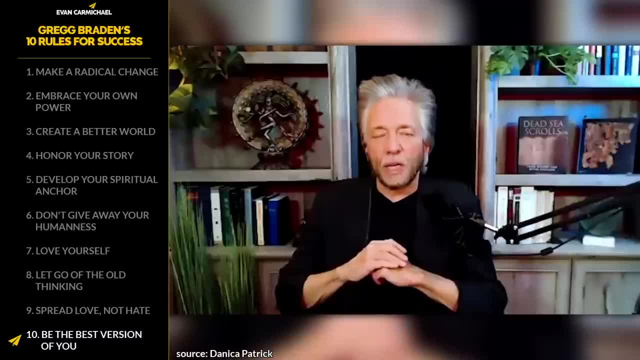 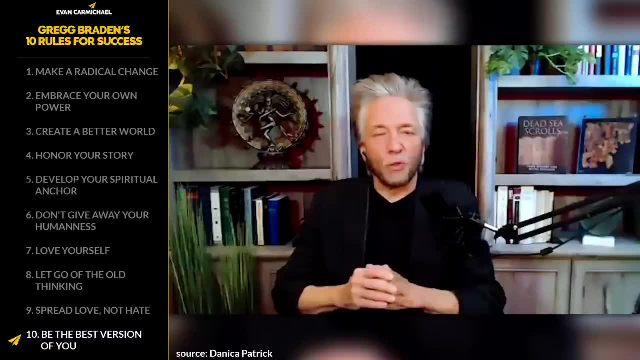 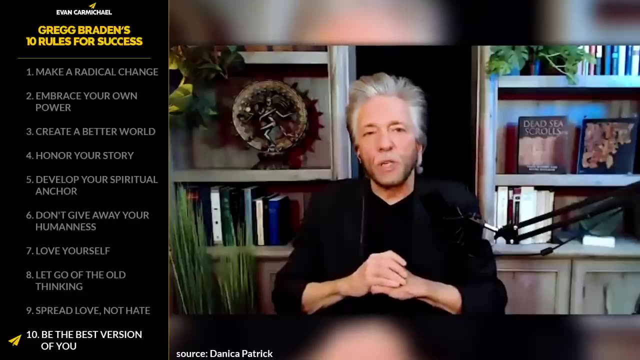 it may be new This we're talking about the scientific way of interpreting and understanding what already exists. And, whether we're in a simulation or not, whether this is a virtual reality or not, we're here, And we're here learning something, And I think the best that 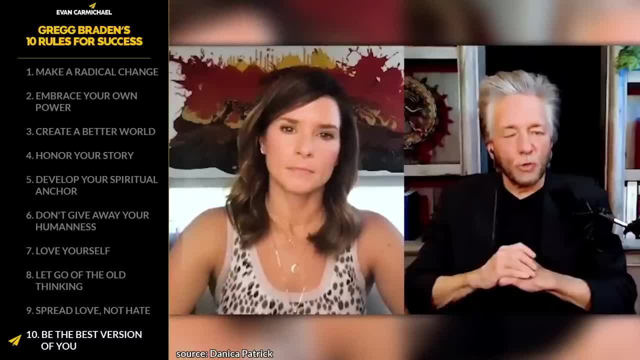 we can do is to be the best version of you, And we're here, And we're here learning something. And I think the best version of you is to be honest, truthful and factual with ourselves when it comes to who we are and what our potential is, And to take that information. 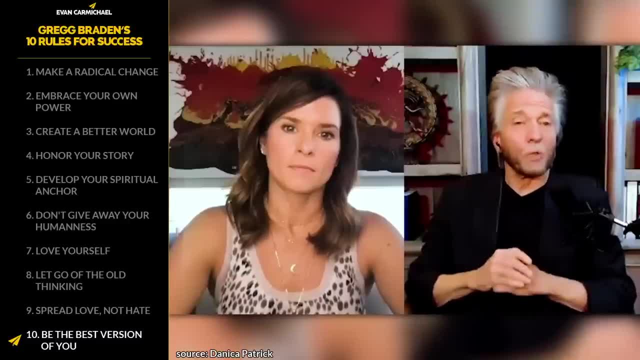 to become the best version of ourselves and our lives and create the best world possible. Because we are in this world And whatever it is that we're here to learn, I think this is the path to the learning. I know so many people. 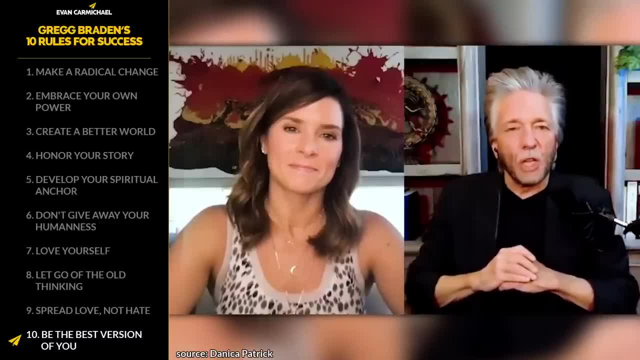 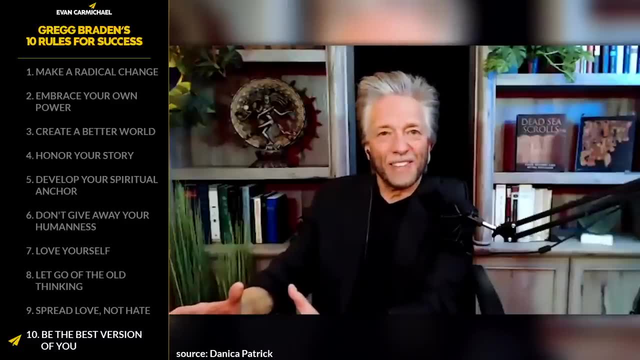 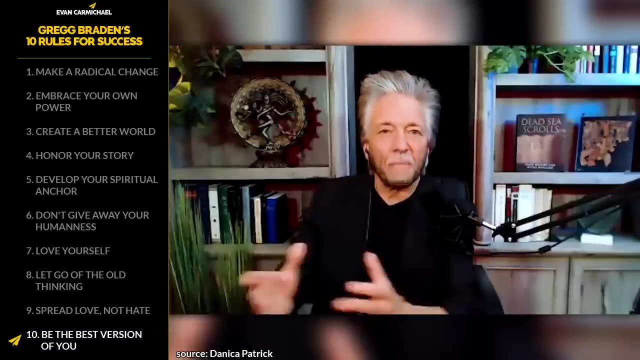 and you probably do as well, who've had such painful lives, Danica, that they will make the search to understand who they are the diversion in their lives, And by diverting from the reality of everyday life, they miss life itself, And I believe that life is here The beauty of this. 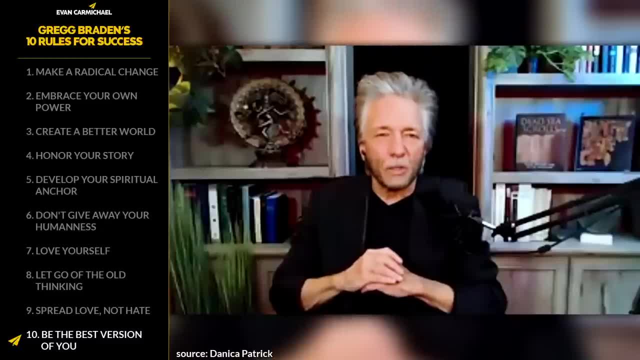 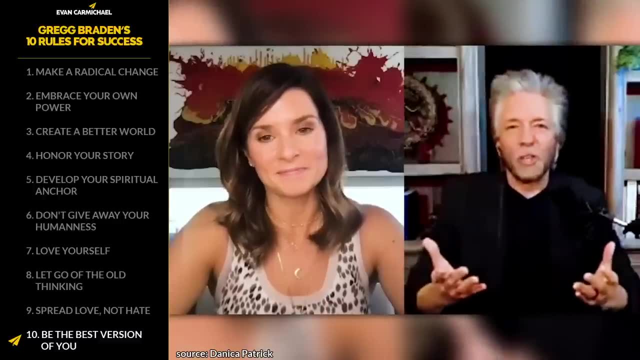 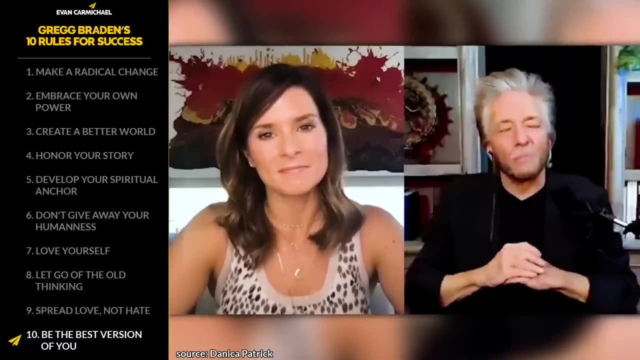 world. this is such. we take it for granted. the colors and the sky, And just water, and the way water works, and music and our ability to create these vibrations that move our soul. This is what life's all about, So I just want to invite everyone. I think it's good. 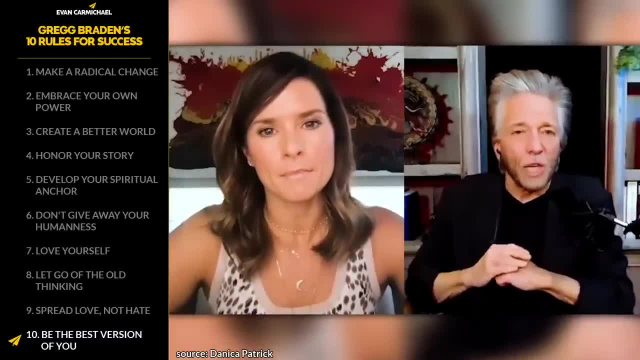 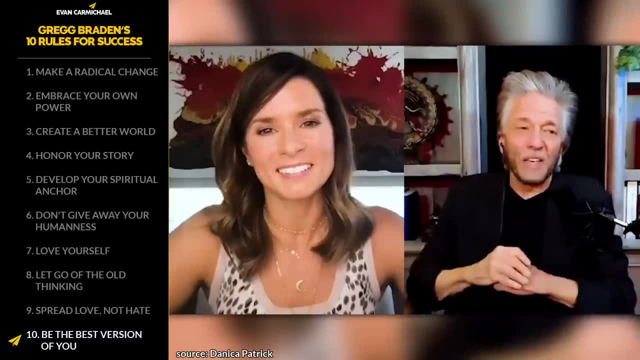 to entertain deeper understandings and to use science as a language, but it comes right down to it. It's about you and me and everyday life, being the best people we can be and finding the joy that really makes our soul sing, Because I think that's our compass. That's how we know when we're on the right path. 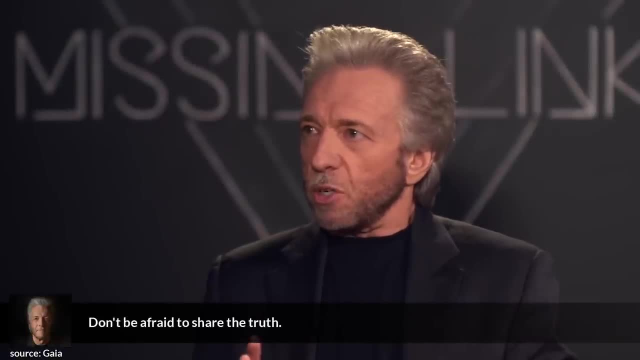 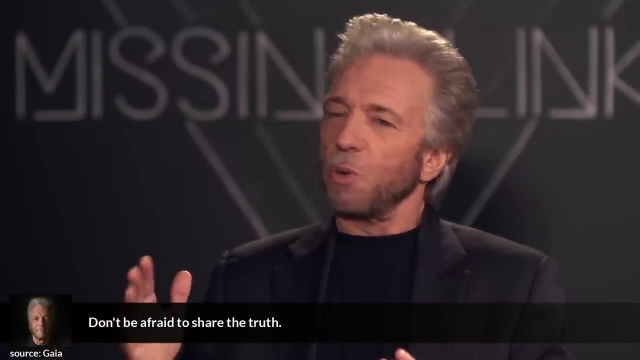 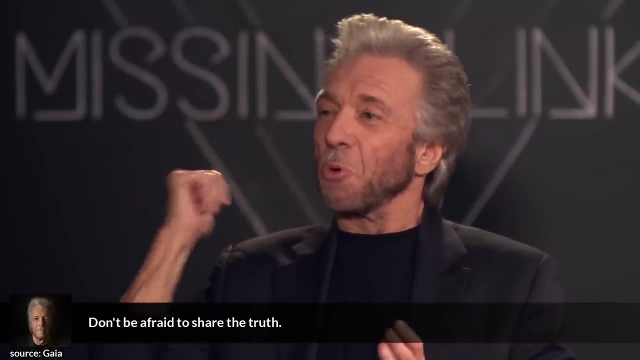 I had a colleague once that said: change in a big corporation, change in a nation, is kind of like a big ship on the ocean. When they want to turn around and go back the direction they came from, they don't turn on a dime. It's a broad, long, sweeping turn that eventually gets them going. 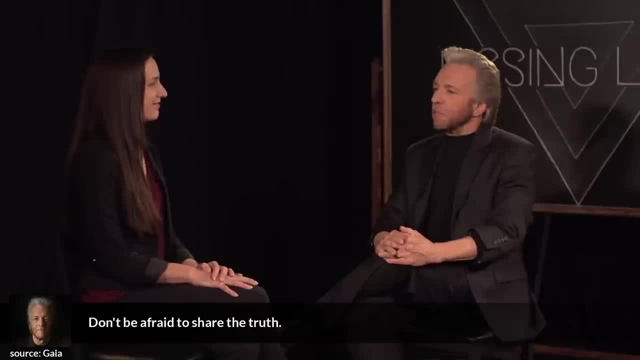 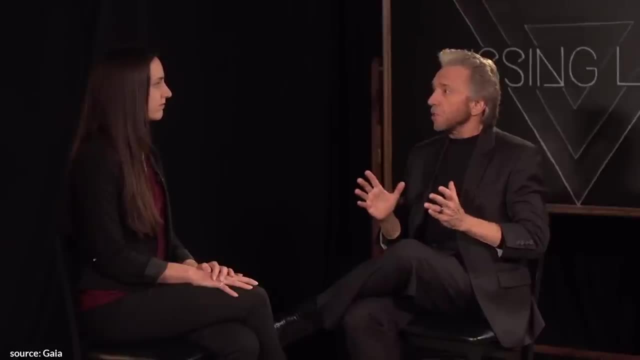 the other direction. Change is like that, But it is difficult. I have friends in academia that have devoted and dedicated their entire lives- 40,, 50 years- to teaching, And what they have said to me they've said, Greg, if we share this new information, it 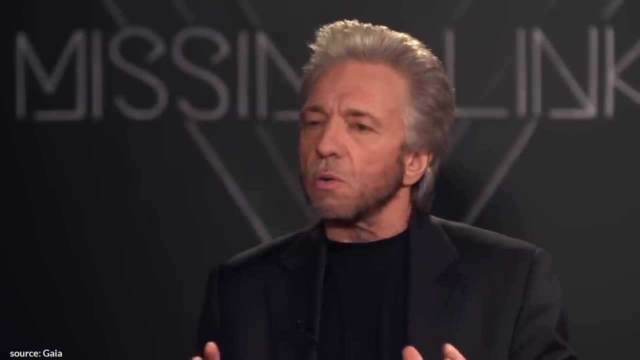 invalidates our careers, is the feeling, And I said no. If you share this new information, it actually validates science, because science is designed to be constantly updated. You're showing your students how valid science is because it's not locked into a specific way of thinking. 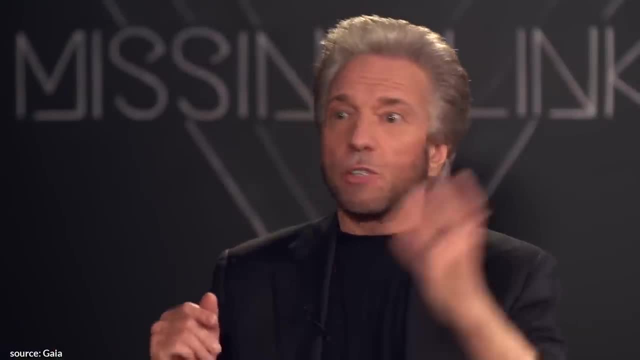 And they say: well, you know, think of how much money it would take to change the textbooks. And I say: well, that's no problem at all, because they're all digital. You change it on one computer and it's changed for everyone. 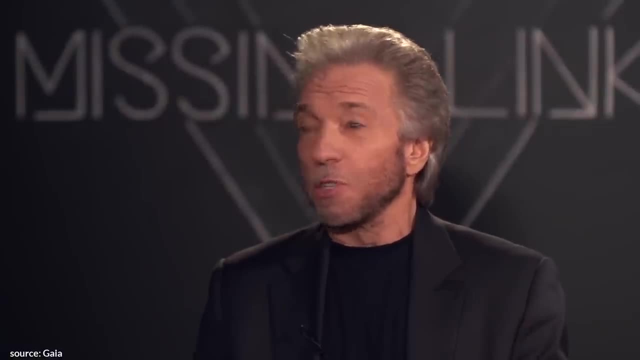 And then they say, well, I have to go back and change my notes that I've created for 50 years. And I say, hey, that's your job, You know, that's what you're paid for. So it's a combination. 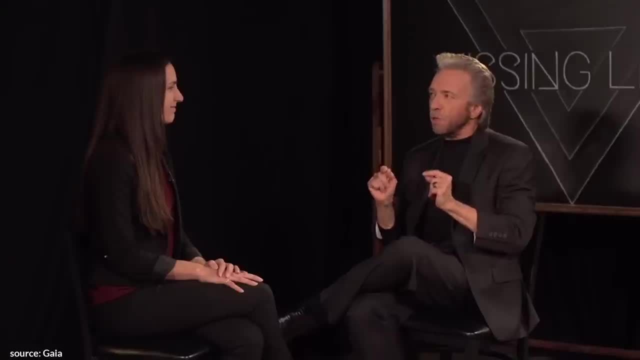 of things. But I will say that mainstream academia is very invested in a scientific story that we now know is false And if we cling to this story, we are teaching our young people a false story And we're not helping them to solve the problems that we're leaving them and asking them to solve.